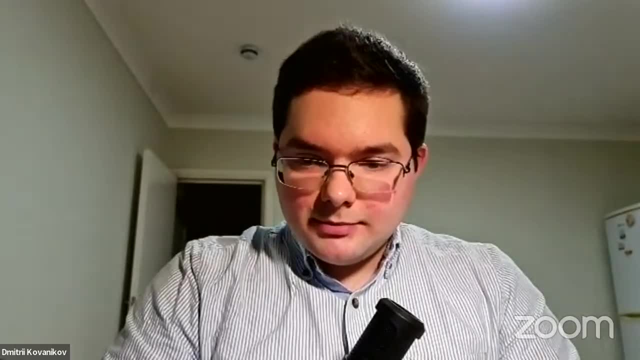 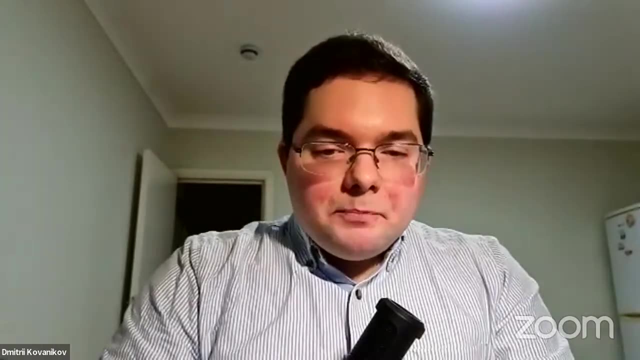 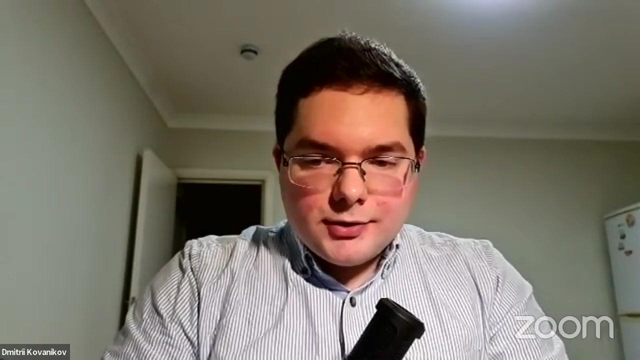 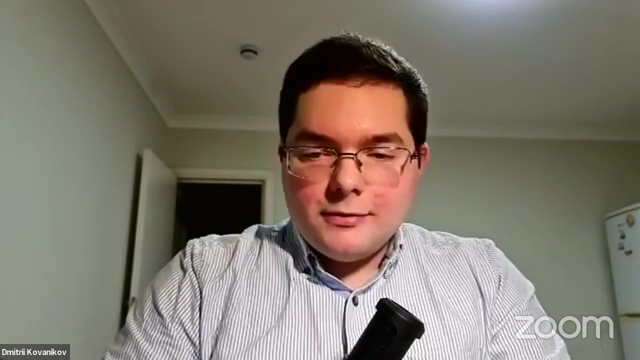 Awesome. See, if people can hear me and see me, That's great. I'll just share my screen And yeah, as I mentioned in the introduction video, I will answer all the questions after the lecture, So but feel free to write them in the middle. If you see something, I will go through the chat. 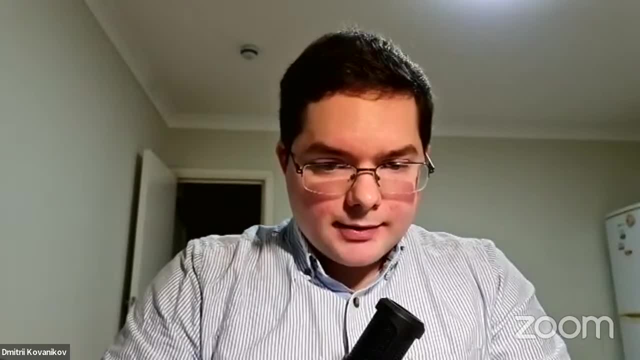 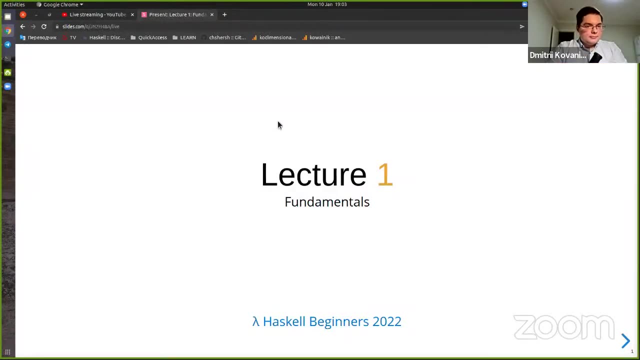 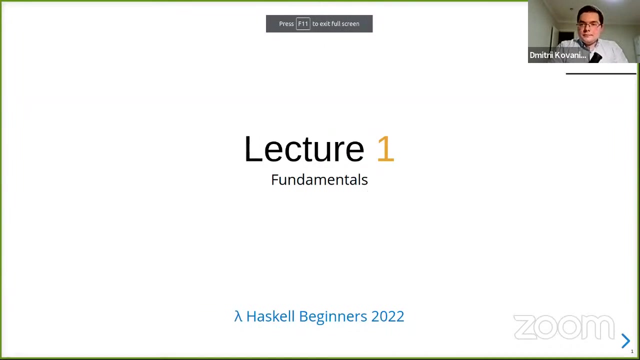 Afterwards and see if there is anything. So Let's start and welcome everyone to the first lecture of my Haskell course for beginners. I'm really happy that you all are here and I'm really excited that you are eager to learn functional programming in Haskell. 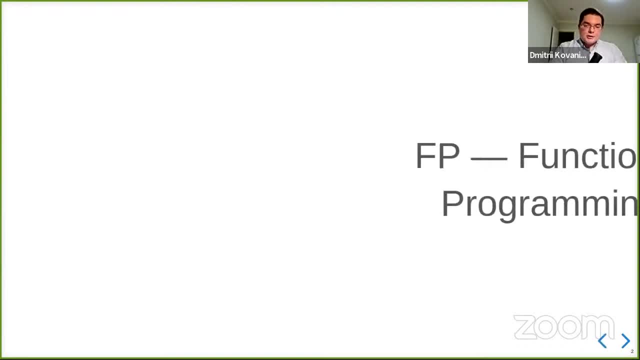 So let's start. So, functional programming, or FP for short. What is this? What is this beast? So I mean the name suggests it's somehow related to functions. So let's figure it out. First, understand what is a function. 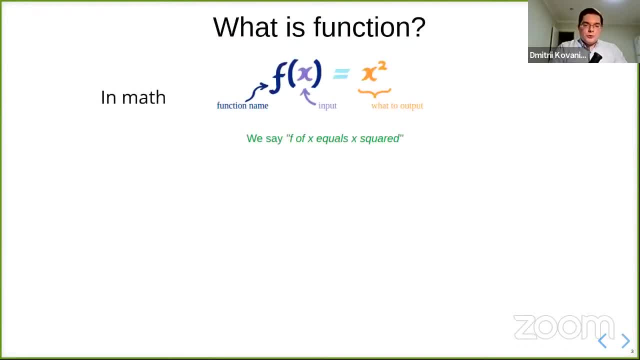 And in math function is a straightforward object, So it has like a name and it has some arguments, some input, and it says what it returns on this input. And for example, in this case we say that f of x equals to x squared. 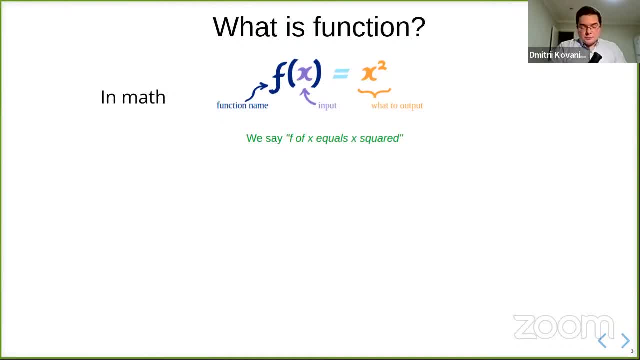 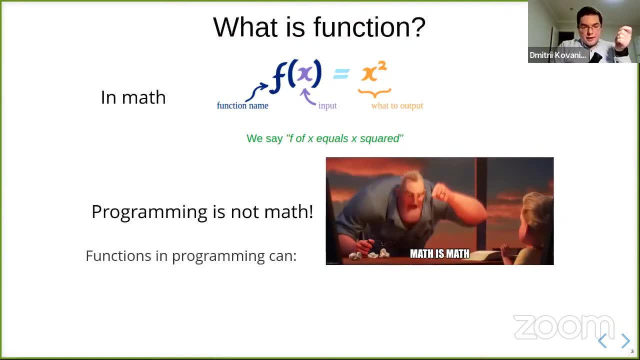 So this is a function that takes one argument and returns some value. However, functions in programming are not like in math And, unlike math, they can do other things that functions in math can do. For example, functions in programming can loop indefinitely. 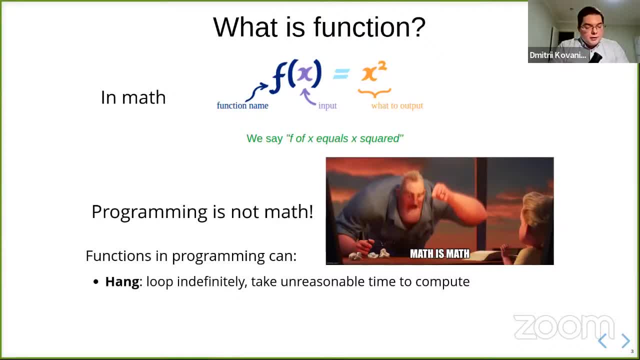 They can work forever or just take a very unreasonable time to compute. It's a very long time. Math doesn't care about how long it takes to compute a function. It doesn't have the notion of computation. But in programming we care about this. 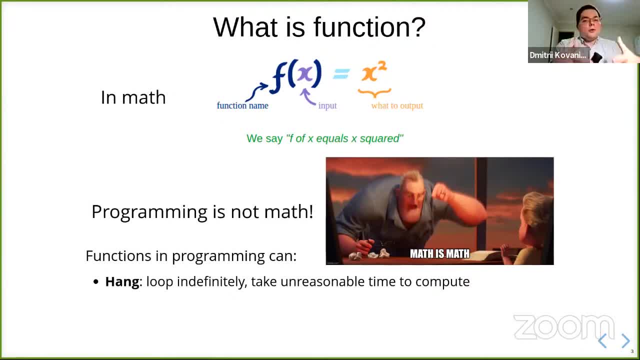 Moreover, functions might loop Not only like by accident, just because of some bug or error, but intentionally. For example, if you have a web server for an application, it's actually not supposed to stop, It's supposed to work indefinitely. 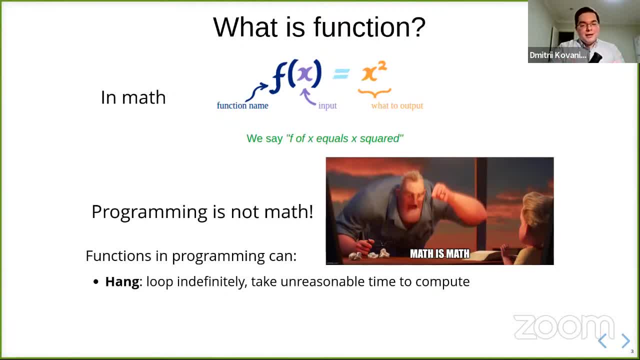 And if it stops, probably something bad is happening. So yeah, some functions are supposed to work all the time. Also, functions in programming can have side effects, So they can read from files or maybe send requests to some servers over the internet. 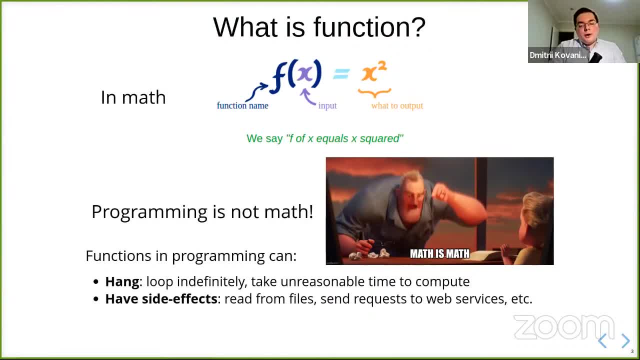 Yeah, Functions in math can do this, So we need to care about this stuff. And because of this, functions in programming can throw exceptions. For example, if you try to read a file and you don't have such a file, so you throw exceptions. 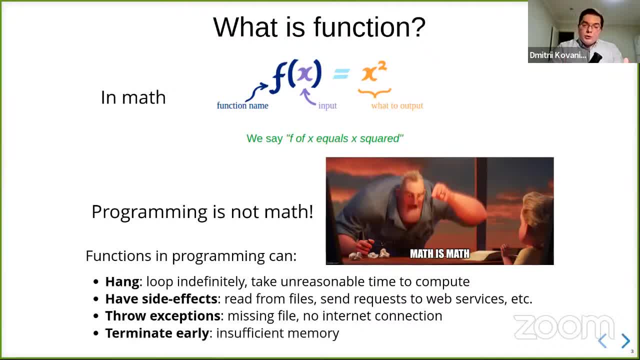 It's some situation that you haven't handled And also functions can terminate early. In programming we have resources like memory, And if functions take just lots of memory, they will terminate early because there is not enough memory to compute them. But math, again, math doesn't care. 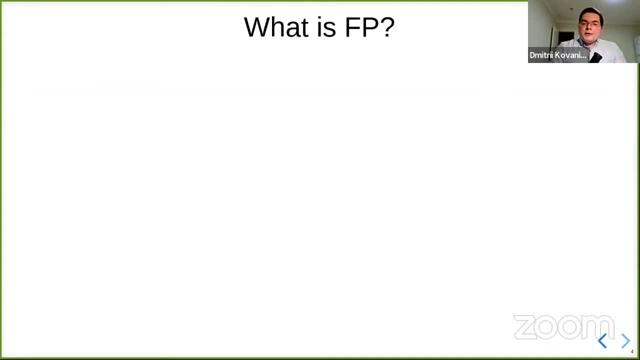 But still, functions in functional programming are trying to be very close to the definition of function in math. So not exactly the same, So just keep it in mind, But still very close. So what is functional programming? So there is no standard definition like accepted by everyone. 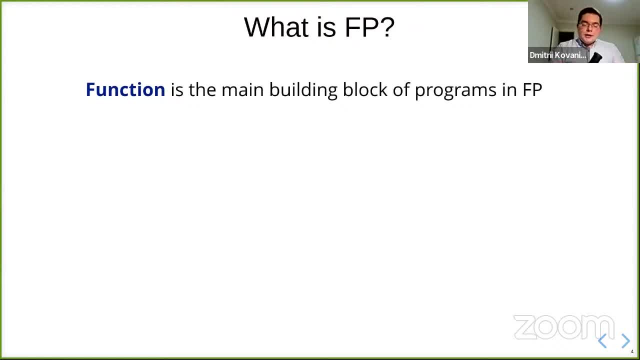 What is functional programming? There are very vague, different definitions, But the main point of functional programming is the focus on functions. So function is the main building block of functional programming, And what it means is that in functional programming languages it should be as easy as possible to create new functions, to call functions, to combine them, to compose, to define new functions using existing functions. 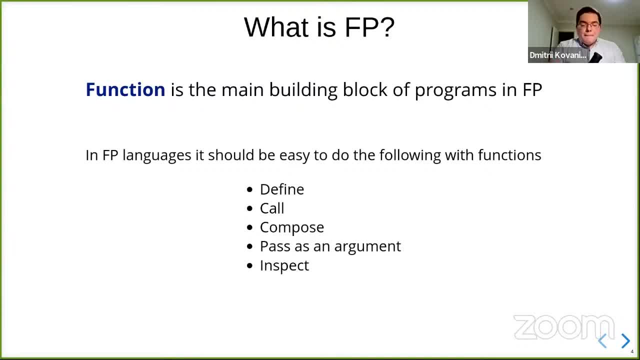 You can use functions as arguments to other functions. You can inspect functions, Basically do everything with that. So, unlike object-oriented programming languages, Where it's easier to work with objects, So it should be easier to work with objects. But in FP it should be easier to work with functions. 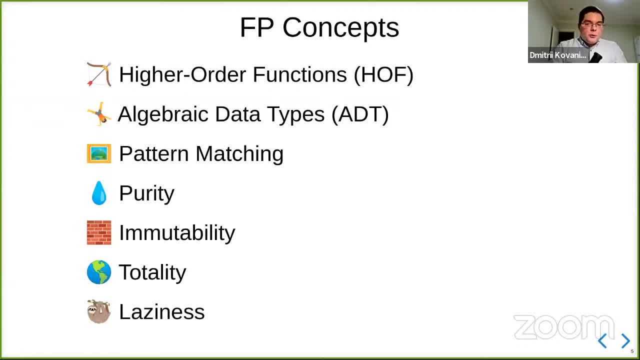 And there are different functional programming languages. But there are some FP concepts that are kind of similar, maybe shared by different languages, And these are the main of them. The first one is the most important, It's the higher-order functions. This means that functions can take other functions. 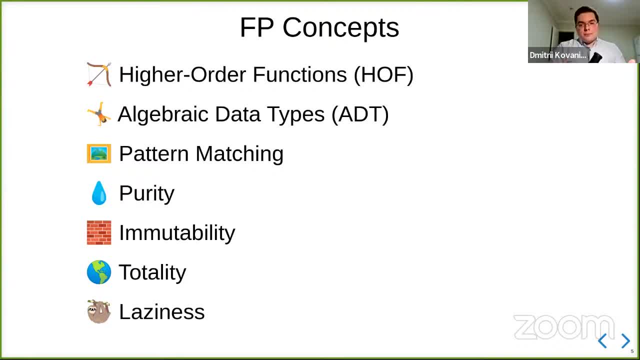 As arguments, As their input. This is a very important concept And we are going to talk about this today. Also, functional languages have algebraic data types. It's a way to create very flexible data types And it's very helpful. 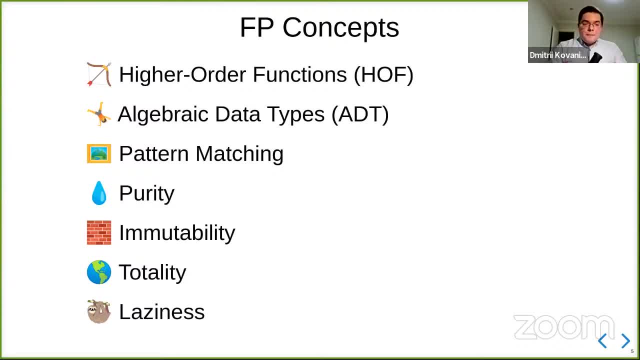 And we're going to talk about this in the second lecture. So once you have algebraic data types, you might want to have pattern matching. This is the ability to describe patterns for your inputs and how your functions behave on these patterns. This is also a really important concept. 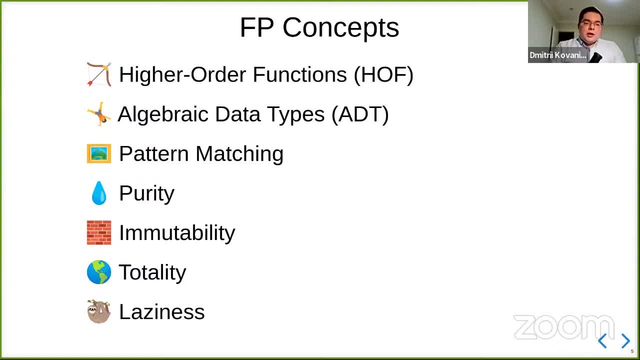 Additionally, functions in functional languages are pure usually And it's encouraged to have them pure, Which means that pure means they don't have side effects Like reading from files or sending requests, So this makes functions closer to the mathematical notion of functions. 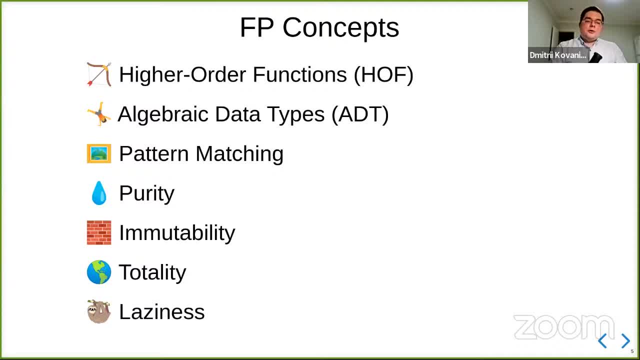 Also, all values in functional languages are usually immutable And immutability is encouraged. Immutability is when you can't mutate variables, You can't change values, And it might be difficult to understand this at first, But it actually makes some things more robust and more reliable. 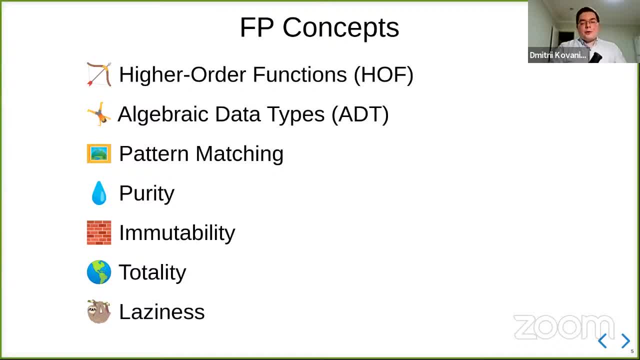 And we're going to talk about immutability today as well. Another concept is totality. Totality means that functions work on all inputs, So they don't hand, They don't throw exceptions, They don't have some cases that are not covered. 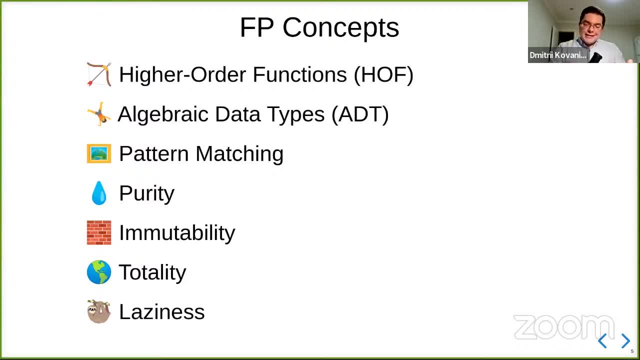 And that's also an important concept. And finally, laziness. So it's not usually like a concept of all functional programming languages. So Haskell is, I guess, the only kind of popular language which is lazy by default. And again, we're going to speak about this today. 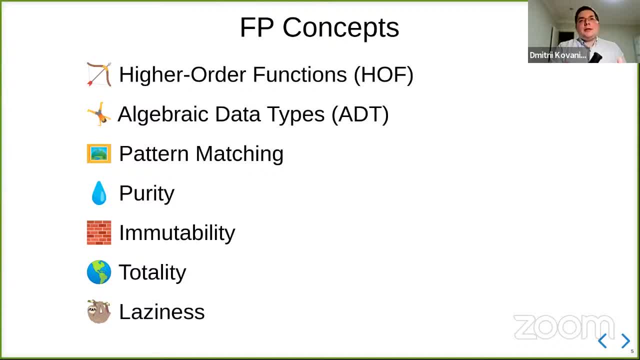 But usually in functional programming languages. laziness means that you work with some infinite streams of data And the streams have some events And you want to process them. And you want to process them lazily, Like when the events come, you want to process them. 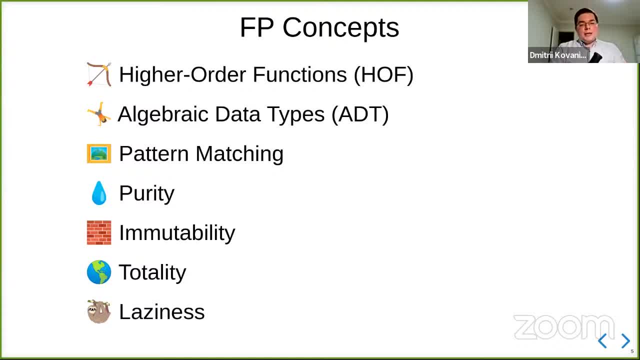 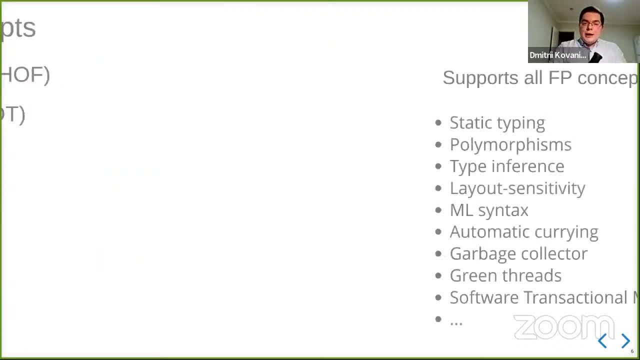 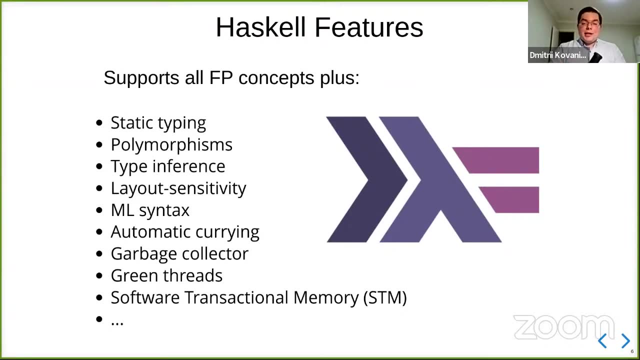 So this is usually what it means by laziness in functional programming languages, And they're pretty good at this. So these are the general functional programming concepts, But besides that, Haskell has its own features, So it's a statically typed language. Not all functional programming is statically typed. 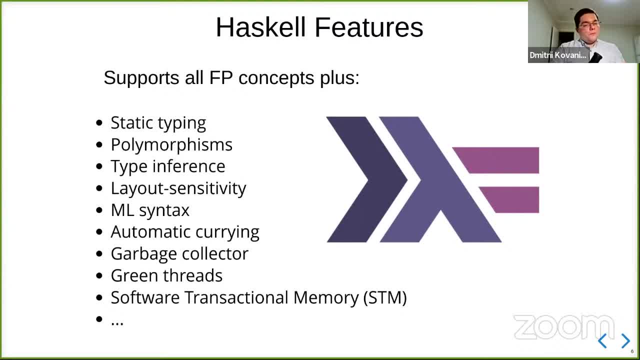 But it has statically typed, So you need to write types of functions and expressions in the code explicitly, And Haskell has polymorphism So you can actually write types of functions that work not only just for single type But for two types, For different types. 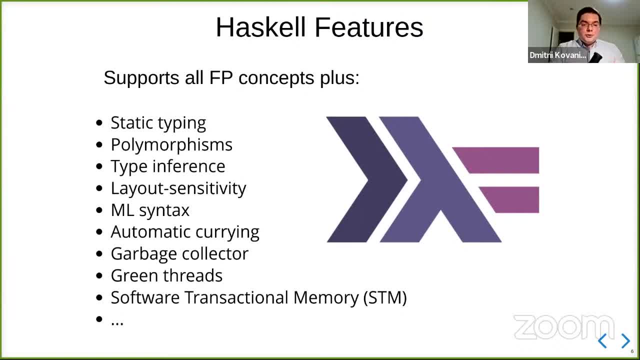 And this is very handy. So you don't need to write boilerplate code. You can just write polymorphic functions. Also, on top of that, Haskell has type inference, So you need to write types, But you actually don't need to write it all the time. 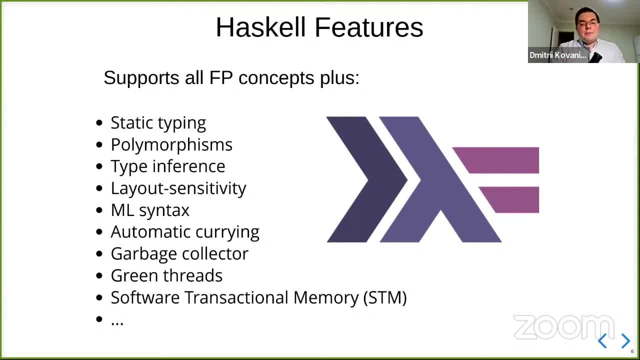 So Haskell has type inference, Which means it infers types of expressions for you. You don't need to specify types everywhere, Just only like in important places in the relevant. There are some syntactic features of Haskell, So it's layout sensitive. 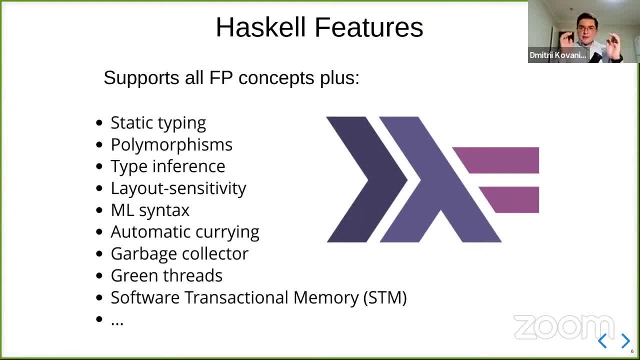 Which means that you don't specify blocks of code with curly braces. You specify them in the same intonation Like in Python. Also, Haskell is coming from the so-called ML family of languages, So ML is short for meta language And most of the mainstream programming languages. they have C-like syntax. 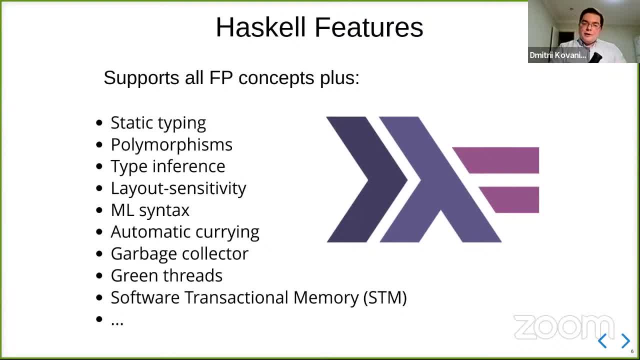 So Java C, sharp, Python, Ruby, JavaScript, They're like in the same family But there are other family of functions- Haskell, OCaml F, sharp. They have different family And this is the thing that makes also Haskell kind of maybe difficult to learn. 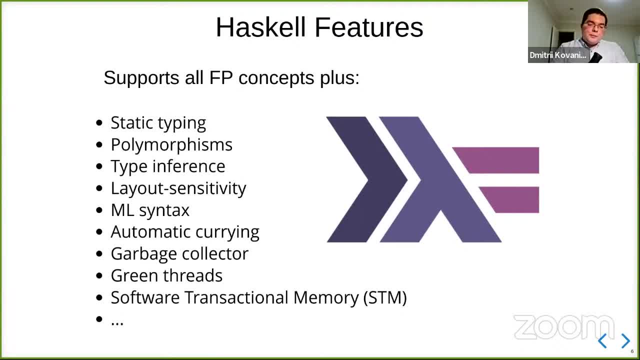 Because it has different style of syntax. We also have automatic array- And we're going to talk about this today- Which means that you can apply functions partially And get also other functions, And you don't need to have extra syntax for this. 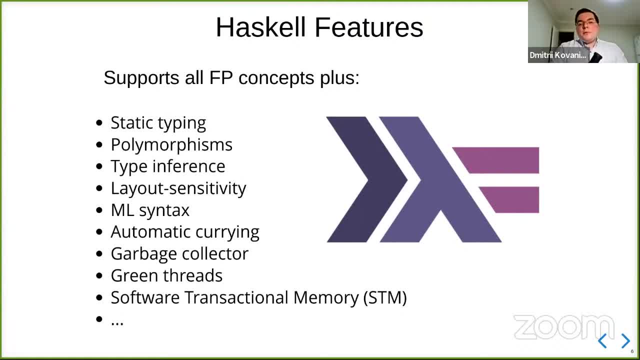 It's not true for other languages, But these are the programming Like type level, Some programming level features. But Haskell also has its own runtime system And this runtime system has a garbage collector. So when you allocate new values, you don't need to worry about memory management. 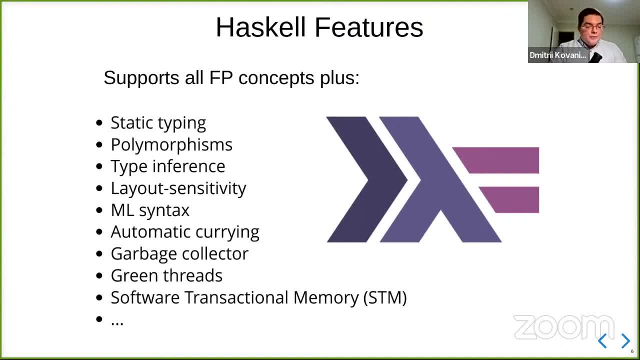 Haskell does this for you. You can create threads, And Haskell has green threads, Or so-called lightweight threads, Which are like, don't take a lot of memory, And you can have thousands of thousands of those threads without worrying about memory consumption. And also Haskell has software transactional memory. 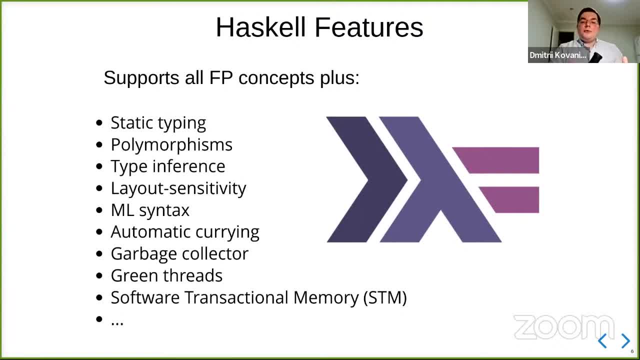 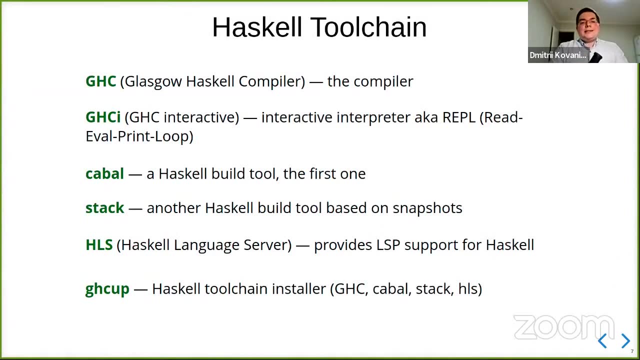 Which is kind of neat concept when you want to have atomic operations. So Haskell kind of pushes this functional programming on the concurrency And all the functional programming concepts are really important in concurrent programming. So before we talk about Haskell itself, let's talk about Haskell tool chain. 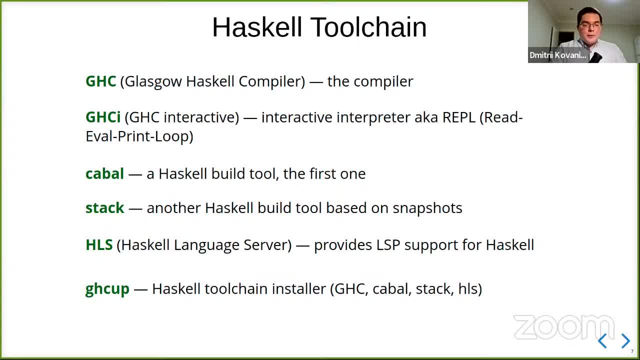 These are the main tools in the Haskell ecosystem. So the main one is a GHC, Which is a Glasgow Haskell compiler, And this is a compiler for the language. it takes Your code And it produces the program that works with it And also does some of that. 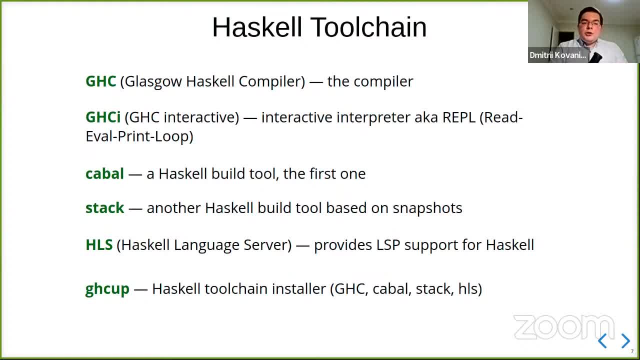 This is the main compiler. There is GHCI, Which is interactive interpreting, And we are going to work with this a lot. There are two build tools in Haskell called Cabal and Stacks, So you can have one file, But then you have multiple files. 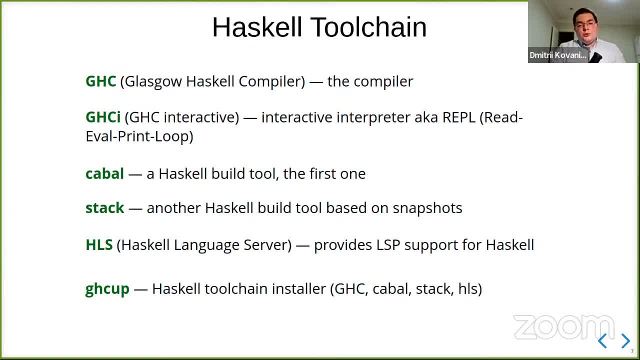 You may want to organize those multiple files in the projects And you may want to use projects by other people. So this is where you want to build. So Cabal is the first one, And Stack appeared later. This is what you need to do to use. 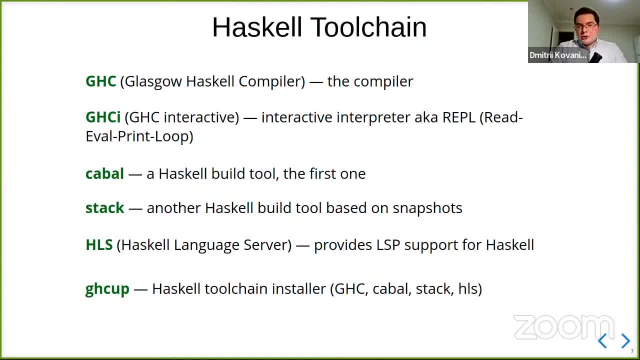 HLS is a Haskell language server. It is an implementation of a language server protocol for Haskell. So basically, if your IDE has language server support, You can have Haskell support out of the box. This is kind of mostly the main support IDE in Haskell at the moment. 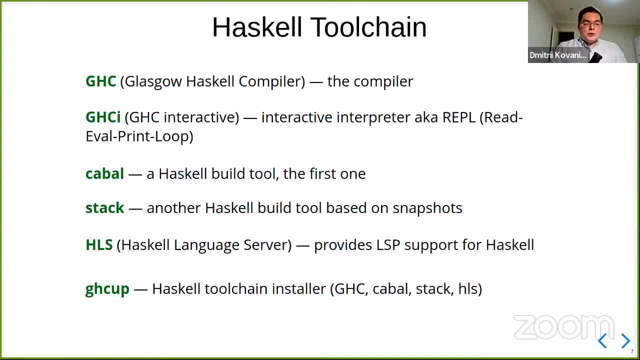 And finally there is GHC app, Which is a tool for managing all of the above tools. So you just usually install GHC app And you can install everything else with it And you can set versions, You can set default versions- Kind of managing all the stuff. 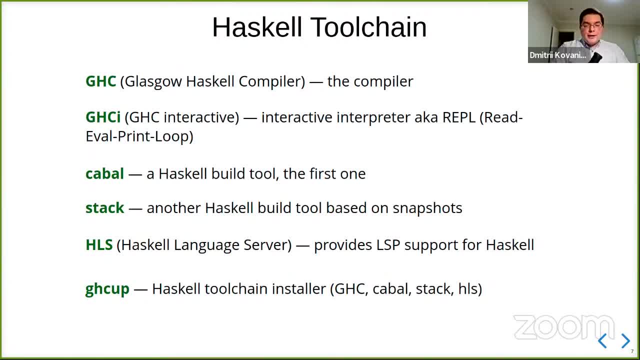 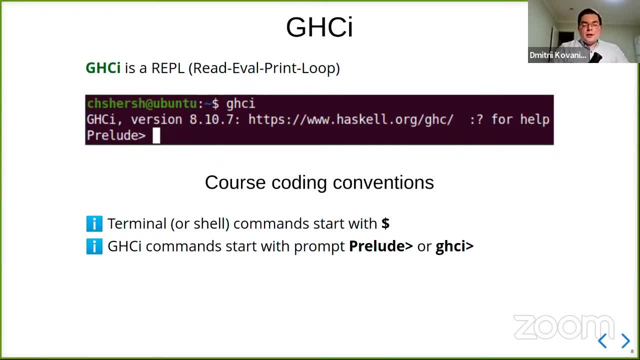 So once we have familiarized ourselves with the tool chain, Let's start with Haskell. So the first one is GHCI. GHCI is a REPL, And REPL is short for Redeveloped Print Loop. What it means is that it is an interactive interpreter. 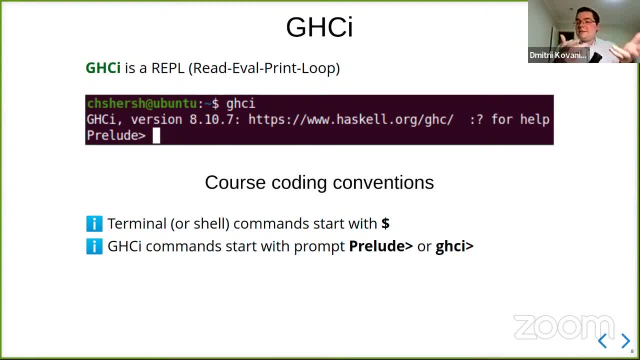 You write something inside it And you immediately get the feedback of evaluation of what you write. So you may call some functions And do some computations And you will get the result immediately. So it's like reading your input, Evaluating your input. 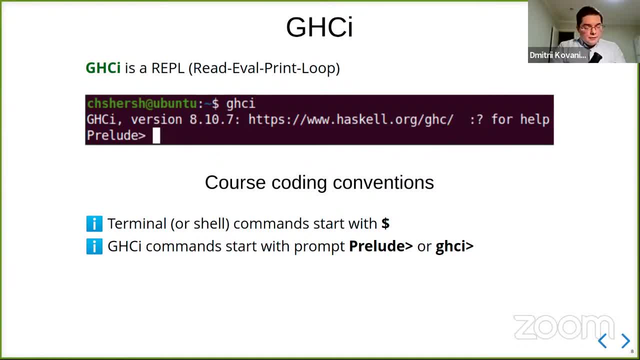 And printing the output And doing this like step under step. This is what does it mean. And you don't need to install GHCI separately. If you install GHC with GHC app, You get GHCI out of the box, So you run it in your terminal. 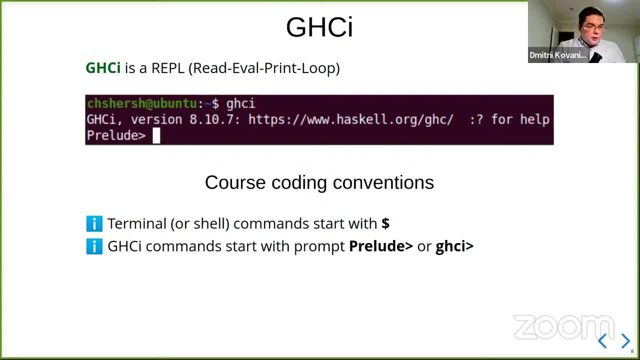 And you can type it immediately in the terminal. And we are going to use GHCI a lot in this lecture and presentation To see how Haskell works, And the convention of this slide is that if there is some command in terminal, It will start with $. 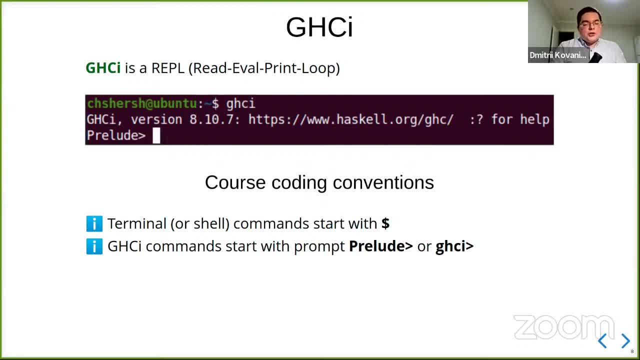 Which means that I'm calling outside of the shell. But if it's a GHCI command- It's like Haskell expression or something- It will start with a prompt, Like prelude arrow or GHCI arrow. So this is a prompt where you can start. 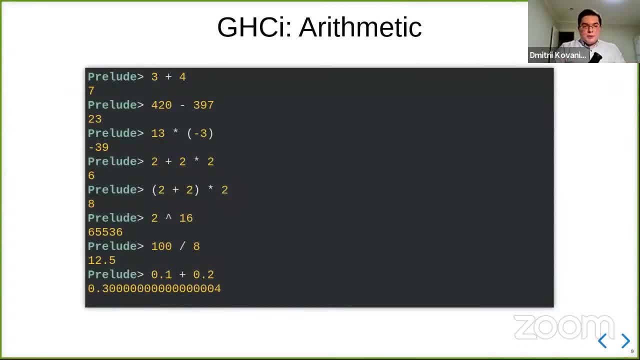 And let's start with fundamentals, With the basics. So in GHCI you just type, Or you can type arithmetic expressions, For example 3 plus 4. And the GHCI will immediately type you an answer Which is 7.. 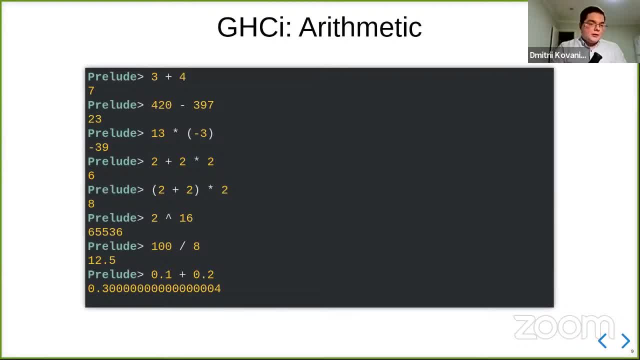 So you can do all the basic arithmetic operations Like addition, Negation, Multiplication, Division, And if you want to use negative numbers, You put them in round brackets. So Haskell don't mix it with subtraction operator. You can use multiple operators. 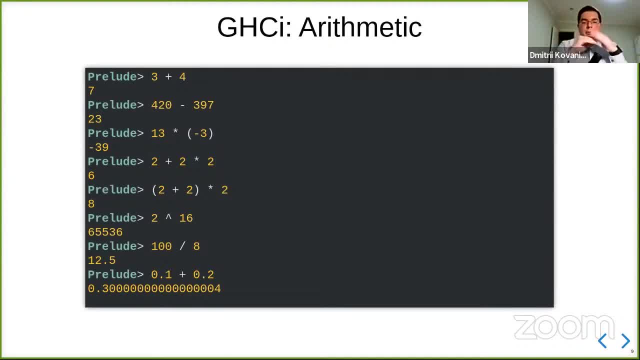 And Haskell will put implicit round brackets for you. We all know from school that multiplication has higher priority than addition. But if you want to have your custom order of operations Or if you want to be more explicit, You can put your round brackets manually. 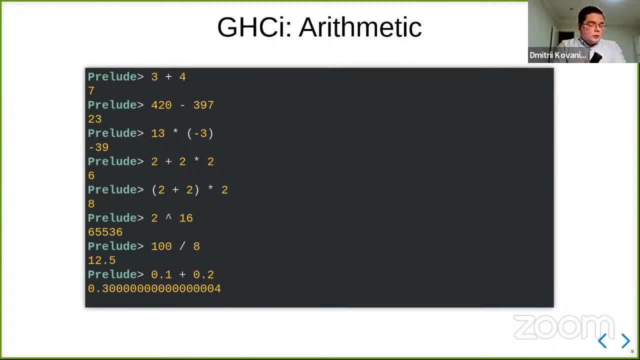 This is just basic arithmetic. Like you can use power operator And if the result of your application is like floating point number, Haskell will deduce this automatically for you And you will get like a floating point result. This is basically arithmetic. I actually often use GHCI just as a quick. 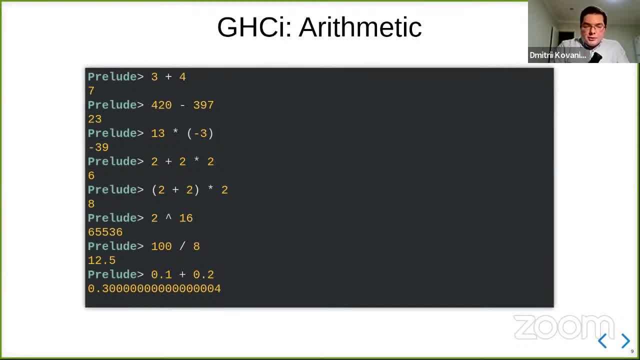 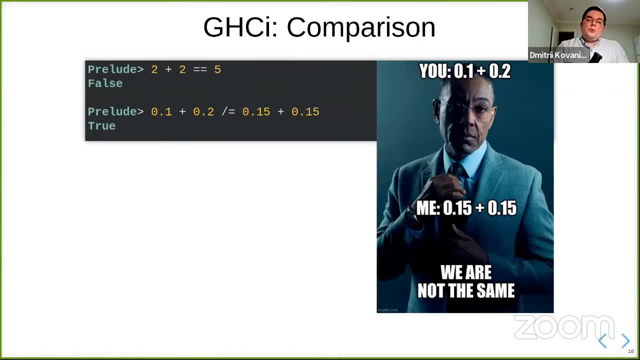 Calculator And still I just type some numbers If I want. Okay, Haskell also have comparison operators, Like all the basic stuff there. If you want to check two values for equality, You use the equal equal operator And GHCI will print you false. 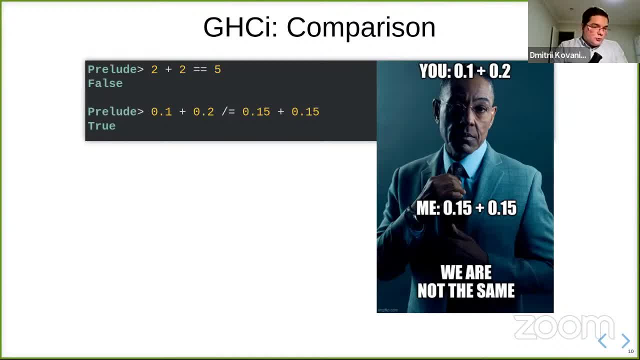 If it's not, The result is false. If it's not true, Or true. If it's again true And not, equals. operator is slash, equals, So it's kind of like mathematical When you put slash on top of the equals. 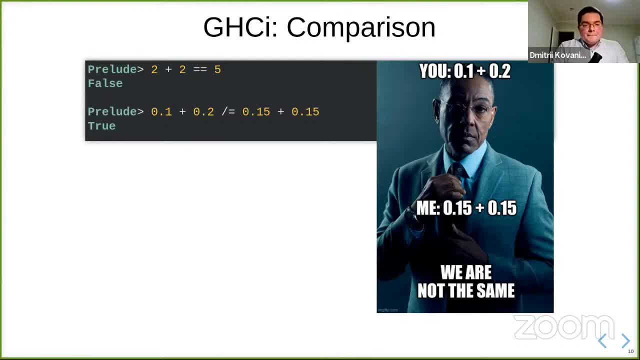 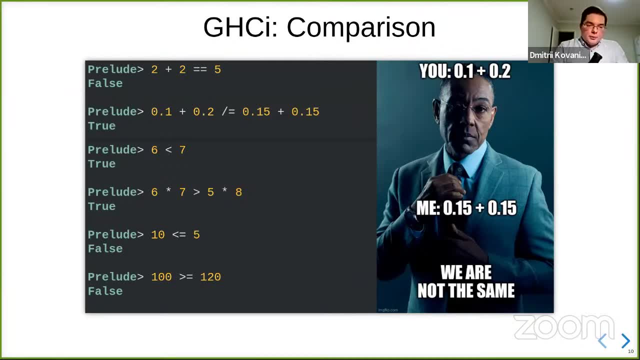 But You in programming before This is just checking operators And there are comparison operators Like less, Greater, Less or equal And greater or equal. This is just some basic operators and standard common functions That you use with Haskell to compare values. 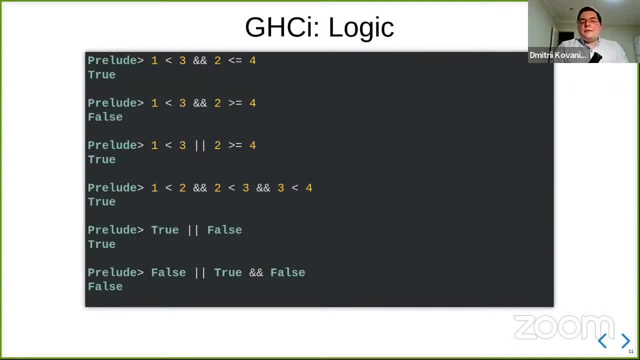 Also You can like combine different values If you want to check if both your conditions are true. So if you have two expressions That returns true or false, You can use like double on percent operator Which has the both should be true. 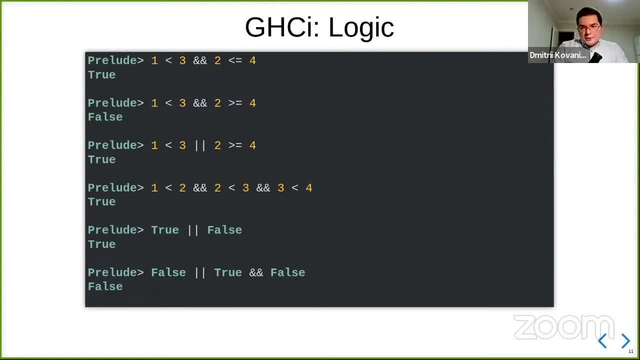 Or you can use this operator, Which is like and operator, Or you can use the or operator, Which is a double vertical lines. It says that at least one of the expressions should be true And it will return true. You can change this operators. 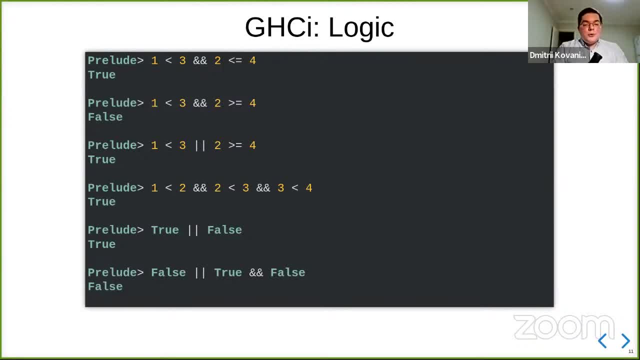 If you want to have multiple expressions, You can use values true and false directly, So we don't necessarily need to produce them from other expressions. You can use them direct. These are just plain Haskell values. So these are just some basic operators. 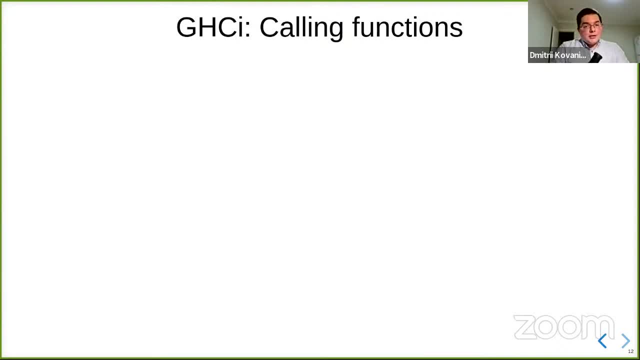 But Haskell has functions And by default You have access to some functions And there's the syntax of calling functions in Haskell. is the same, Is the same, Is the next. You put the name of the function in the beginning And then you put all arguments to this function. 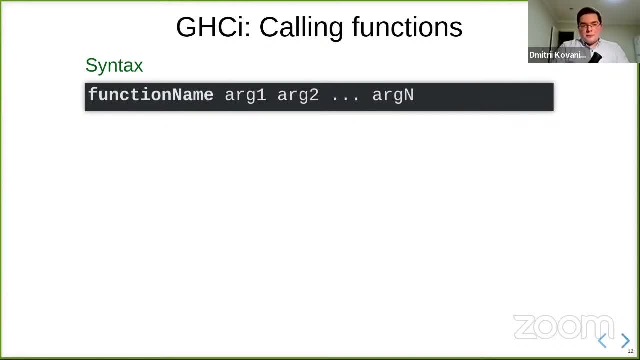 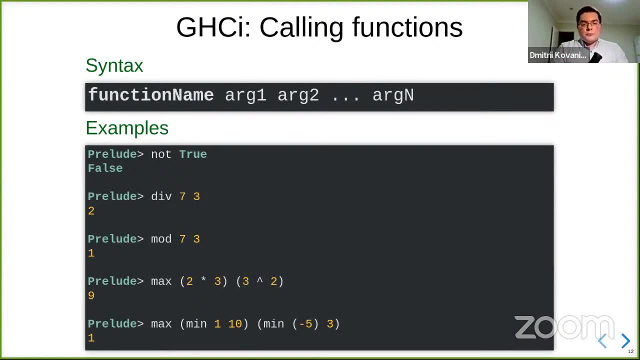 Separated by space. So no commas, No round brackets. For example, There is a function not That takes a boolean And returns the other boolean. So if not From true, It equals false, So we just Pass it. 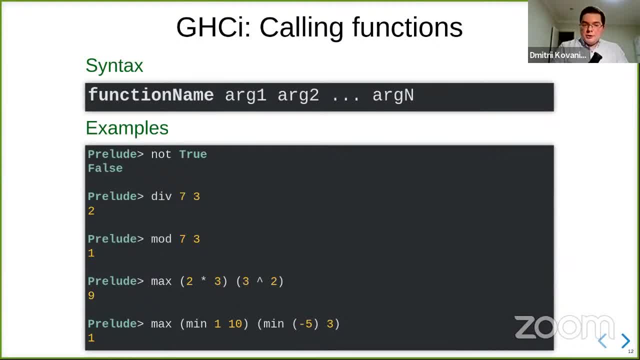 Another argument. In a separate, separated There's function division, Integral division, And if you divide integral seven by three, We get two. Again, We have two arguments And we just separate them by space. But sometimes We may want to group arguments. 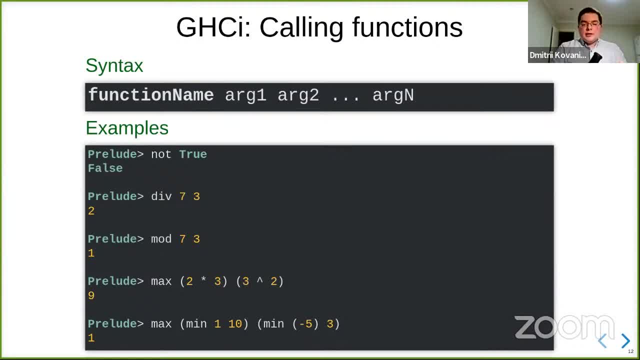 For example, This Two multiplied by three, It's a single argument. So Just to Help Haskell to understand this one, This is the one argument. We put it in round brackets. This is how we group arguments. So the function. 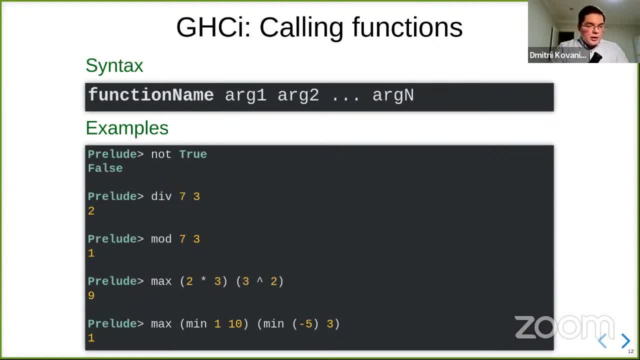 Max. It takes Maximal Of two values. The function Mean Takes Minimum Of the values And we can use Nested functions Inside, But we don't. We don't want to skip this round brackets. It's really important to remember. 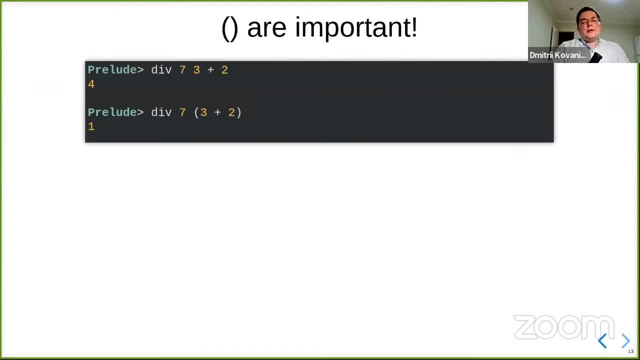 And again I want to emphasize this. So depending on how you put parentheses, The values can change. So If we just In the first example We divide seven by three And we get two, And then We add two, 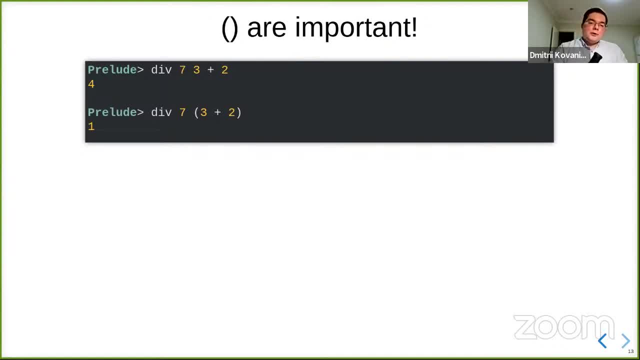 And we get final four. This is how the results. But in the second example We first Add Two And three And we get five. Then we divide seven by five And we get one. So round brackets is important. 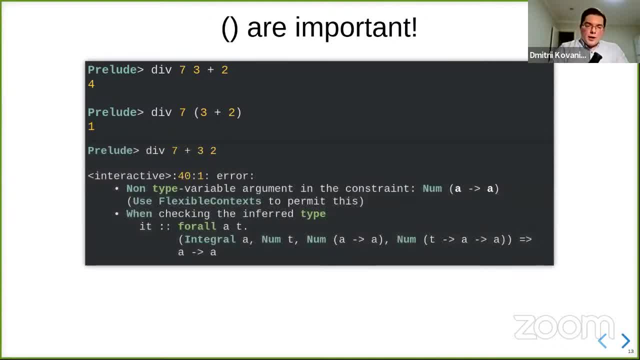 If you Skip the brackets And if you put them in the wrong way, You will Get A Wrong, You will get an error message And it will look Very scary. So But what it means is that you haven't passed enough arguments. 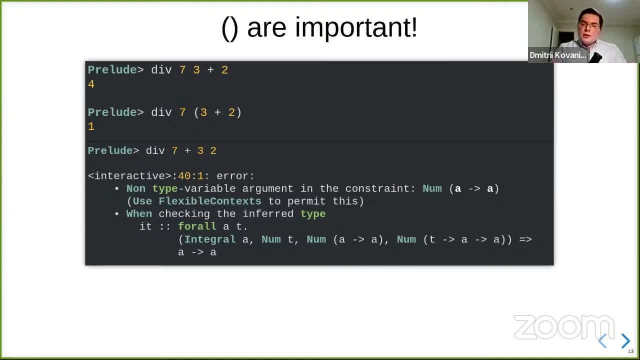 To div. But because Of how Haskell works, How types Most, The error message Doesn't say exactly that And it may look scary. And if you don't understand This, Totally fine. I mean, It's Some gibberish. 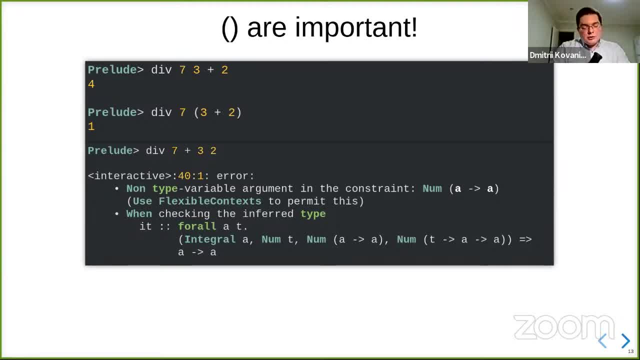 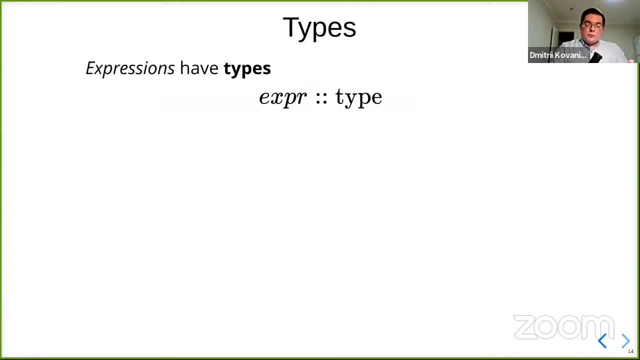 It doesn't make sense For now, But Sometimes If you See some errors, Just check If you pass enough arguments To Your functions. So Just Some practice Basics And let's go to type. So I 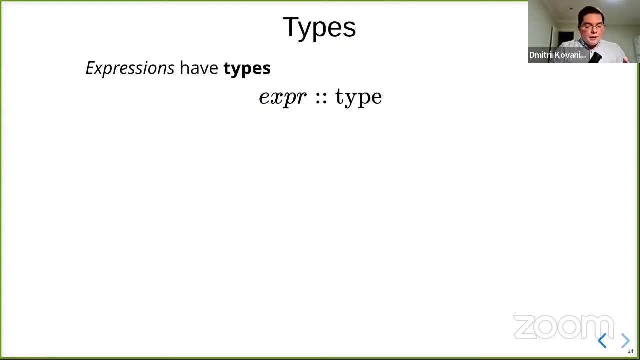 As I mentioned, This is The type Language And And strongly type, So which means All expressions, All values, They have Types And usually When you Want to specify Type Of expression, You put. 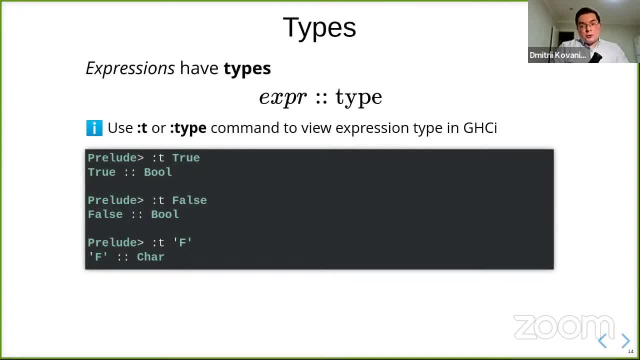 Expression. On the left You put Double Columns And you Write The type. And In GHCI There is A special Command Type Boolean. Okay, What is the Type Of All? 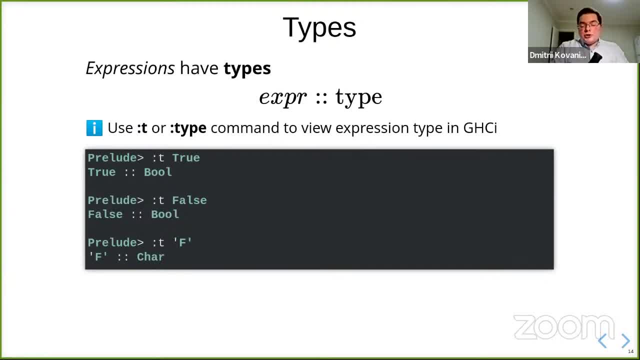 Type Of All Is Also Boolean. And What Is The Type Of Character F? Put In The Single Quotes, It Says Okay. So What Is The 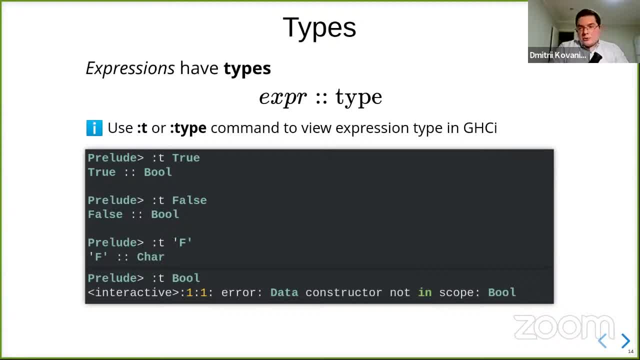 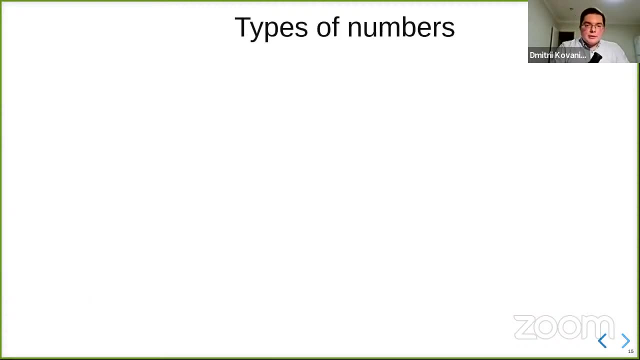 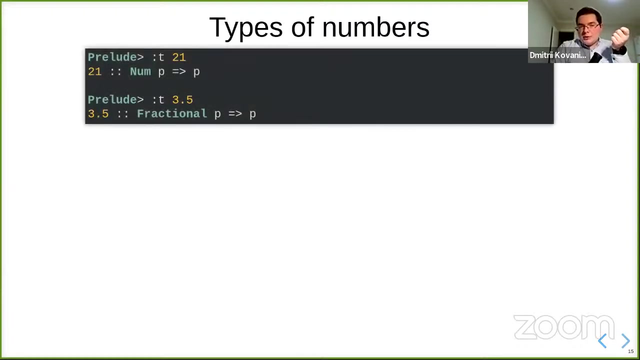 Type Of Bull. We See An Error Message, So It Means Because We Cannot Have, We Cannot Check The Type Of A Type Because Types Are. 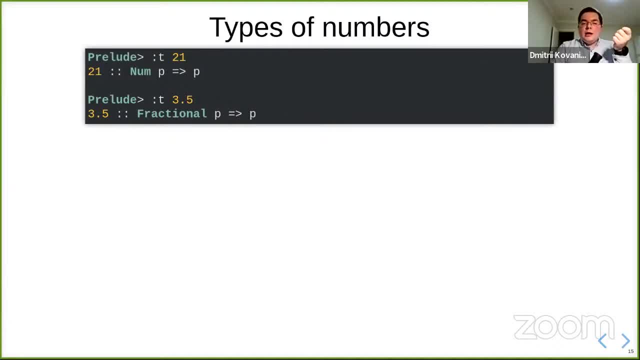 Unexpected. So Let's Say We Want To Check The Type Of Number 21.. And We Won't See Like Some Type. We Will See This. 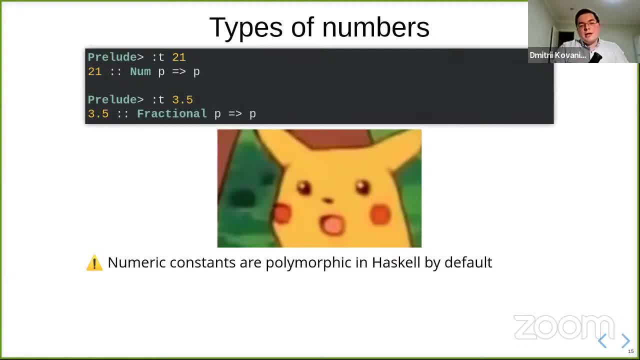 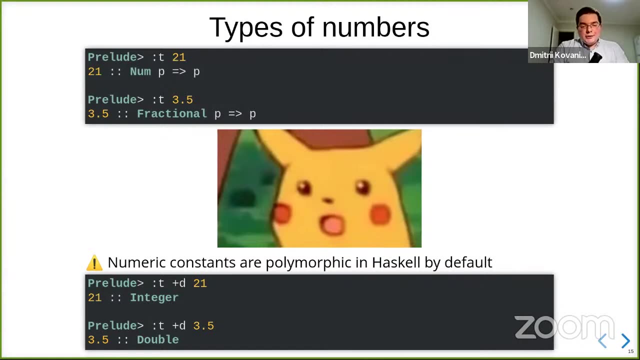 Like Double Arrow. We Mean Different Things, So Things Are By Default Very Polymorphic, So And You May Get Hard Times, But What You Can. 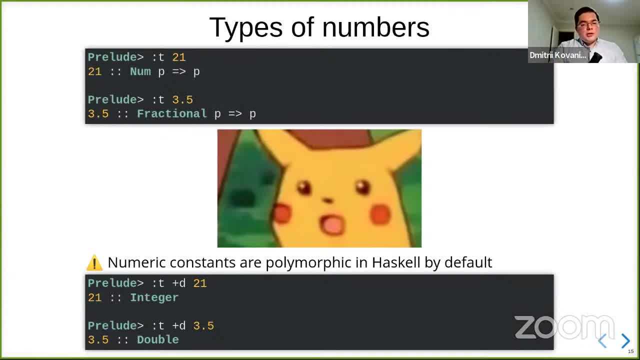 Actually Do. When You Expect Types Of Numbers And The Plus, The Option Just Tells You Which One Just I Will Be You. So If We 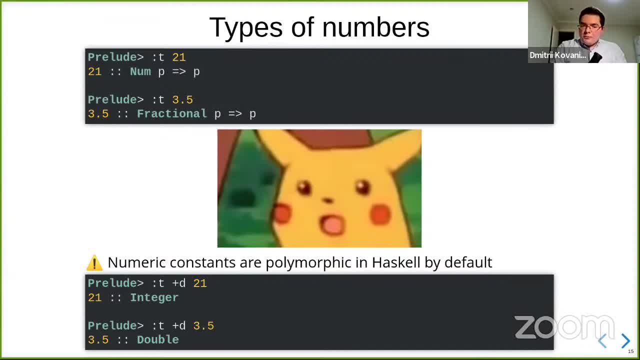 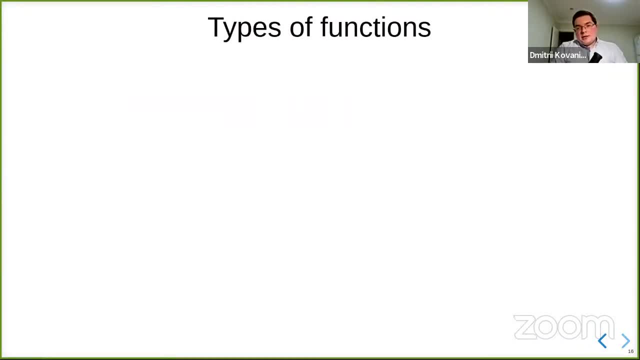 Are Having Like An Integral Number. Just I Will Tell That You Can Check The Types Of Functions. So If You Check The Type Of Function, 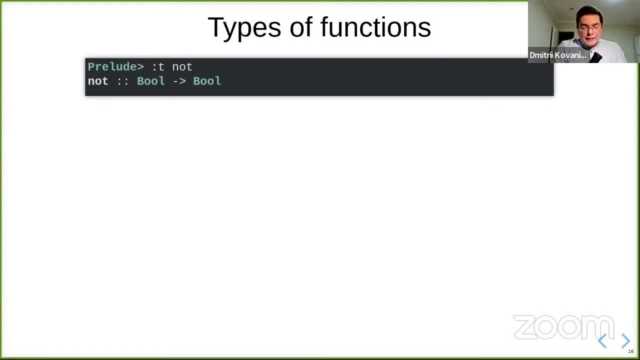 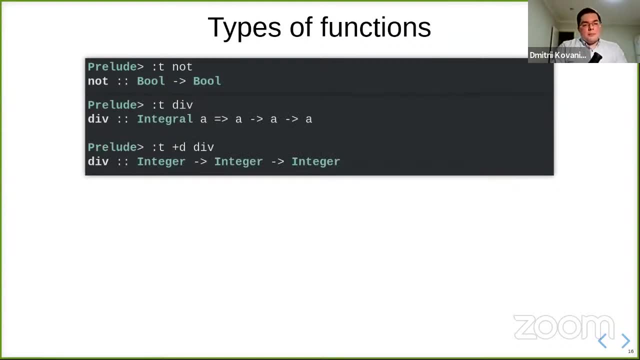 Not. You Will See That's Okay, Not If They. There Is An Arrow And Is Letters And You Can. If You See This, You Can. 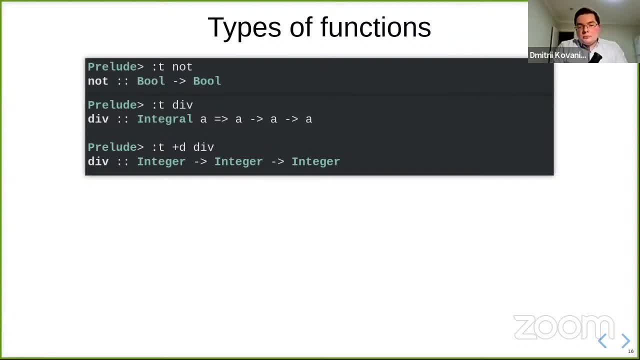 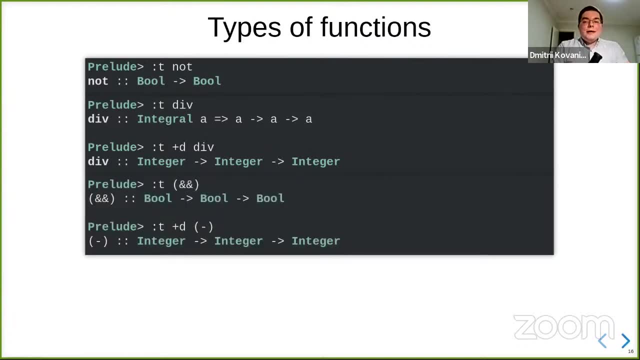 Try To Add Plus The Option And Check If The New Type Will Make Sense. And We See That Is Just Written Using Operator Symbols. So 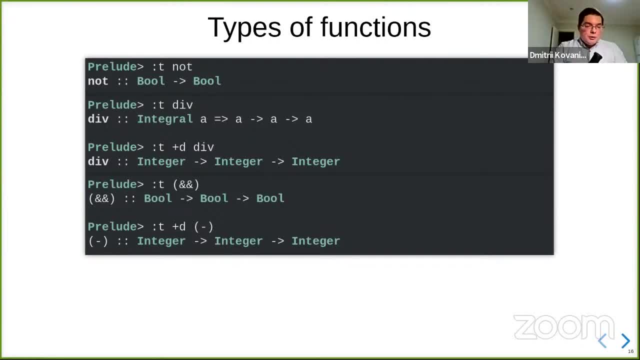 What Are Exactly Operator Symbols? It's Written In The House Of Standards, So It Just Specifies All The Possible Symbols. But Between Your Arguments While 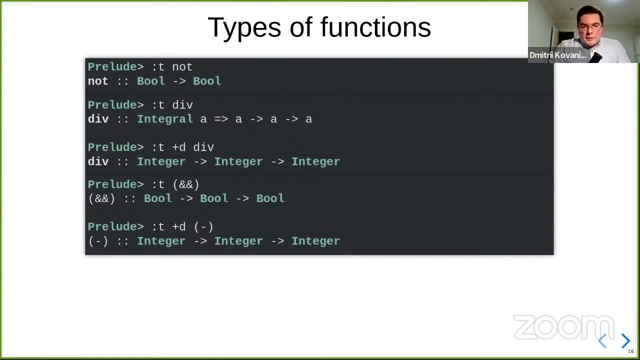 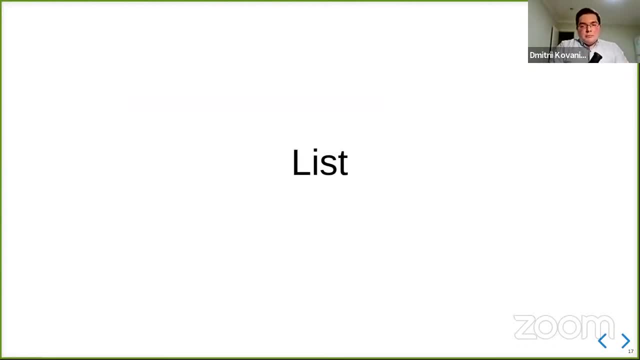 In Case Of The Function, You Put Function To Begin And Then All The Arguments Of This Name. That's Basically The Only Difference Between Operators. 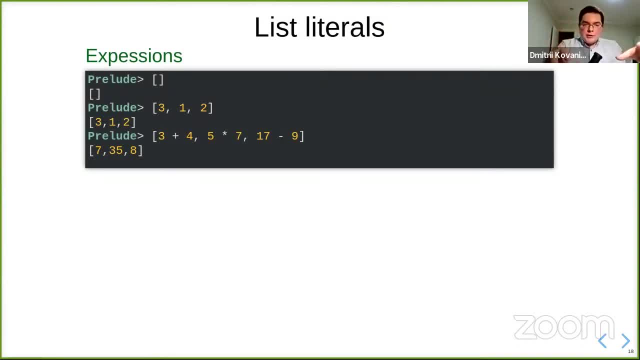 So This Is Just Sequence Of Elements And Empty List. You Just Square Brackets Without Anything In It. So But If You Want To Put, 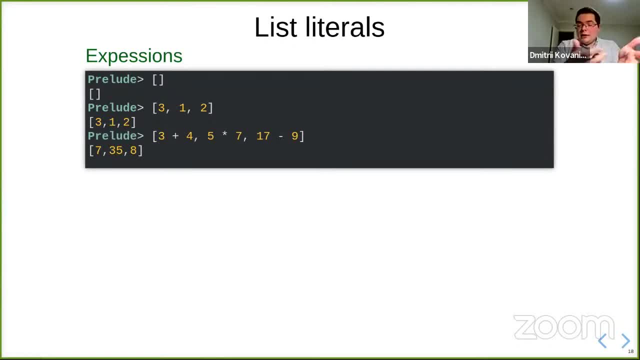 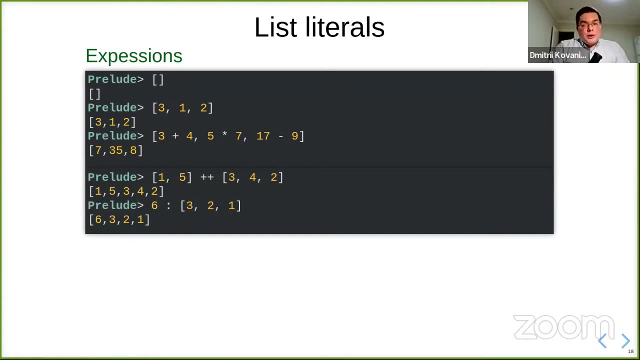 Some Elements In The List. You Can Have Some Expressions In As Elements Of The List And Just I Will Kindly Evaluate Those Expressions. 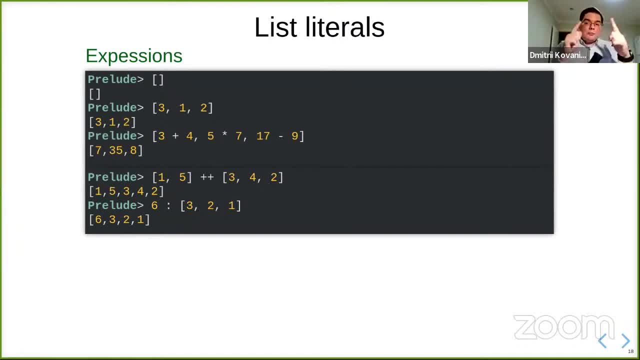 For You When It Will Print The Final Result In List. There Are Two Different Operators Need To Remember And There Is Another Special Operator Called. 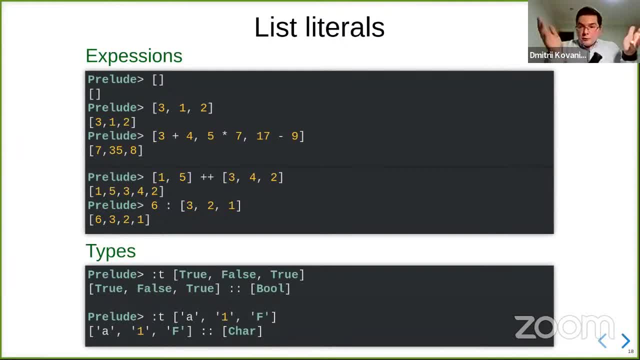 Home Which Takes An Element On The Left Side And List On The Walls And The Letter. This Is True And We Inspect Its Type. 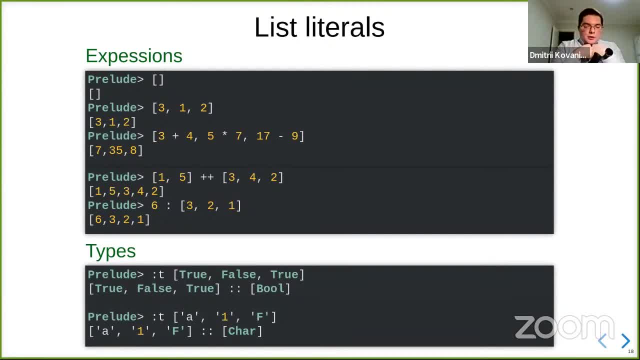 JCI Says That It's A Bull Put In Square Brackets. So What It Means. When You See, This is what it means. So let's familiarize ourselves with basic and fundamental Haskell functions to work. 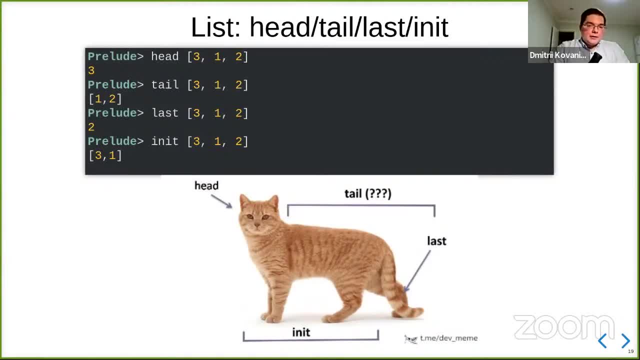 with lists. So first of them is this like four functions: head: it takes the first element of the list. tail: it returns the list without the first element. last, as the name suggests, takes the last element of the list and in it it takes all the elements without the last. 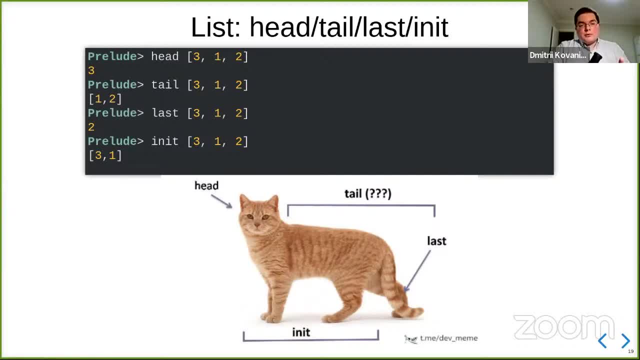 There is a picture for better understanding. This is a very important function. the beginnings are very helpful And it's really nice that they all have like four letters long. all good functions are four letters long But actually those functions are not encouraged to use because they throw exceptions on empty. 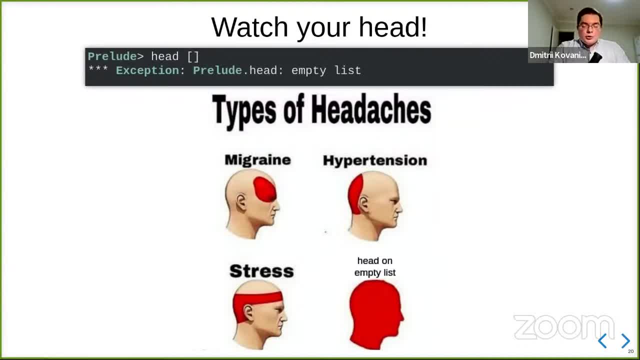 lists. Haskell takes a list and returns its first element. So what happens when you give it an empty list to head? Well, we see an exception. There is no first element in an empty list, So we get an exception. This is actually problematic. 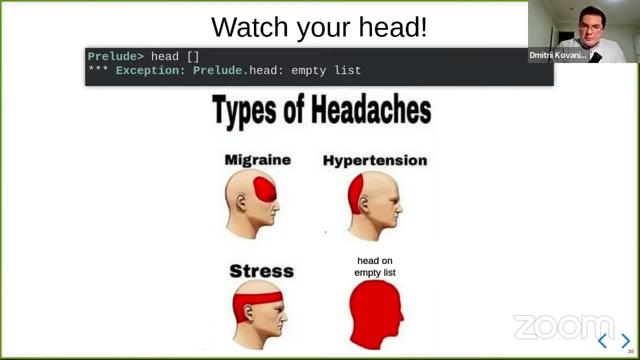 Lots of people have this inspection and they don't know what is happening in their code. That's why it's suggested not to use such functions In Haskell. it's always possible, according to my experience, to write code in a such way that you never need to use these functions. 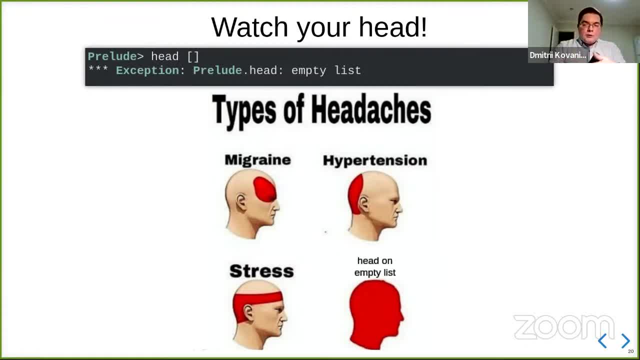 Well, we still. we might use them in the beginning For now, as we haven't learned all the Haskell features and all the syntax. but in general, just no discussion. You should be careful when you're using these functions. Just a heads-up. 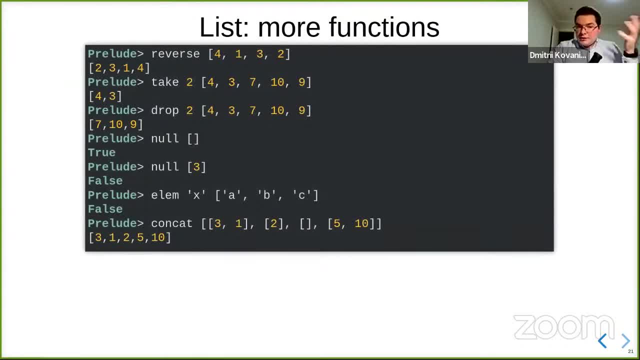 Okay, So there are more functions to work with this. for example, a function reverse that takes a list and returns a new list with reversed elements- Very helpful. There is function take. It takes a number and the list and returns the first elements of the list with the size. 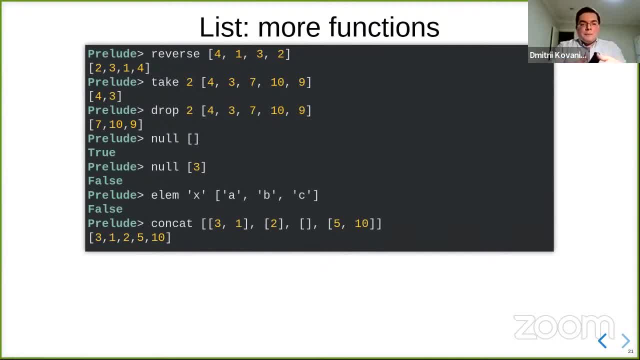 of the number. So take two. takes: returns the list with two elements. Okay, Drop function returns the list without the first two elements. So drop two returns. Null is a function that returns Boolean value whether the list is empty. So if list is empty it returns true. 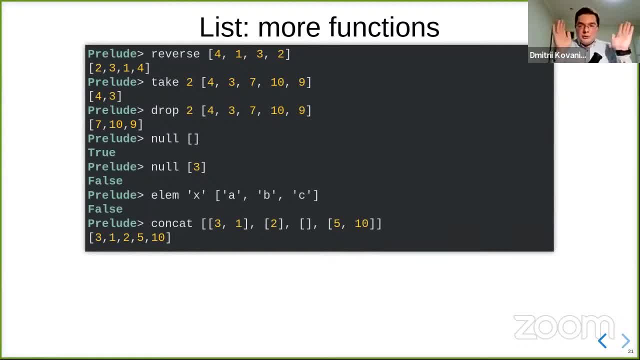 If list is empty, it returns false. So it's not related to nulls in other programming languages, just to check whether the list is empty. Another helpful function is lm. Again, as I said, all good functions have four letters, which is great. 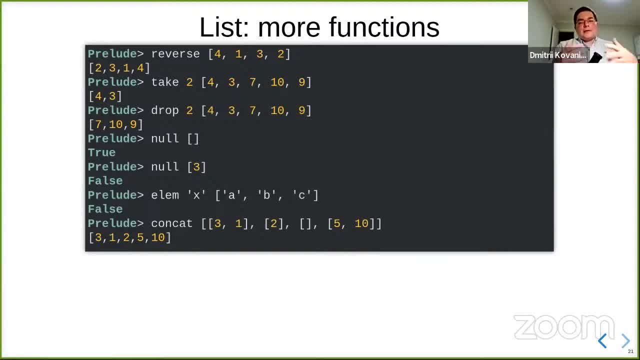 So it takes an element and it takes a list and it checks whether this element belongs to the list. So lm, in this case the character x, is not in the list of characters a, b and c, But lists. again, lists can also contain other lists. 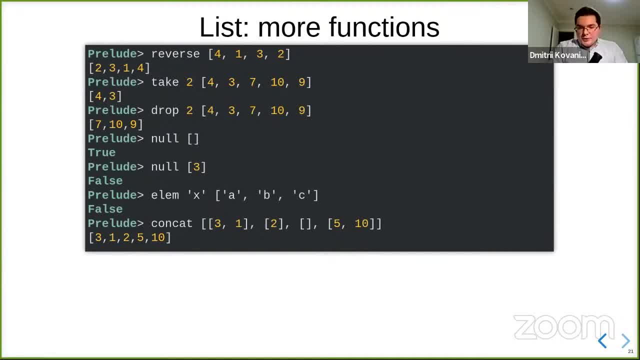 So there is nothing wrong with having a list of lists And we have a function, concat, that takes a list of lists and it just flattens this list, Just concatenating all this list, and we give not a list of lists but just a list of elements. 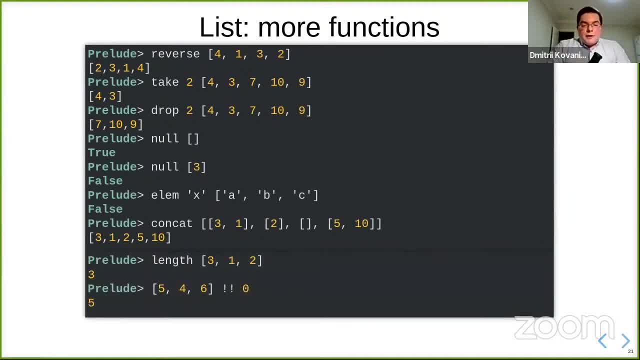 inside. So that's how concat works. Other functions are usual stuff like length. Length returns the number of elements in the list, as the name suggests, And there is this double exclamation operator which is like index operator. It takes, it returns the element of the list by the index. 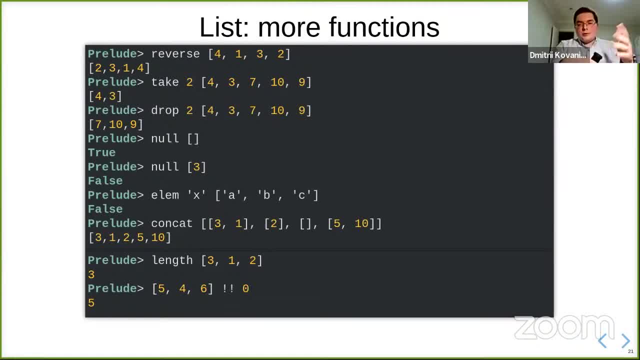 So indexes of lists in Haskell start with zero. So the element by the index zero is just the first element of the list. So same this, these two functions. again, they are not recommended to use because they are very, very slow. So length doesn't like. return your length immediately. 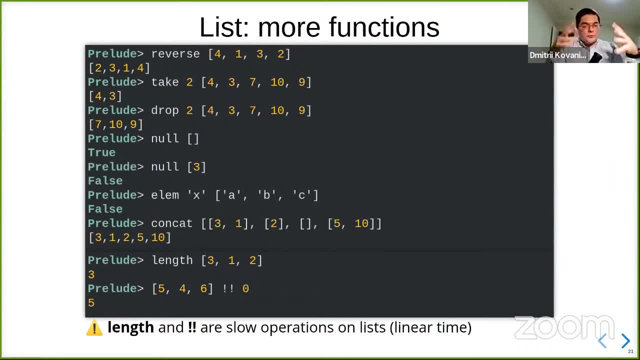 It needs actually to walk through the list to calculate length every time. So that's why length is so slow, And the same is true for the double exclamation operator. So lists in Haskell they're not like. they're more like streaming sets when you consume. 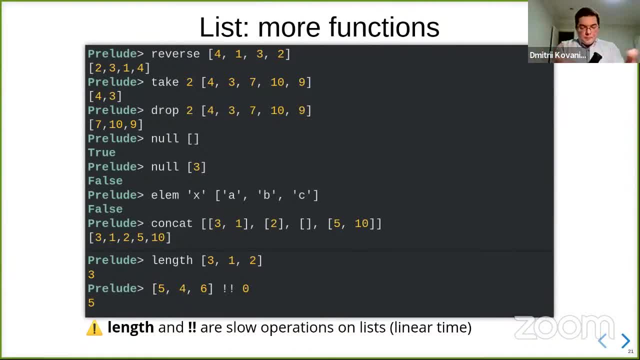 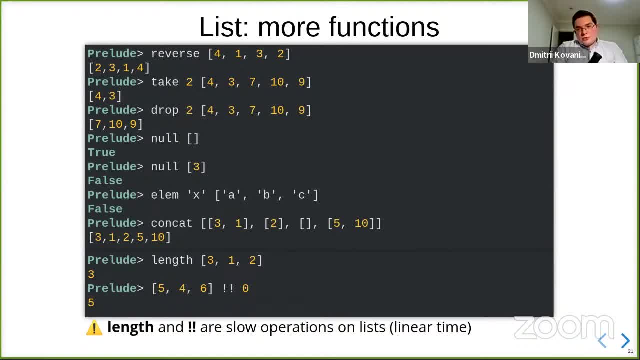 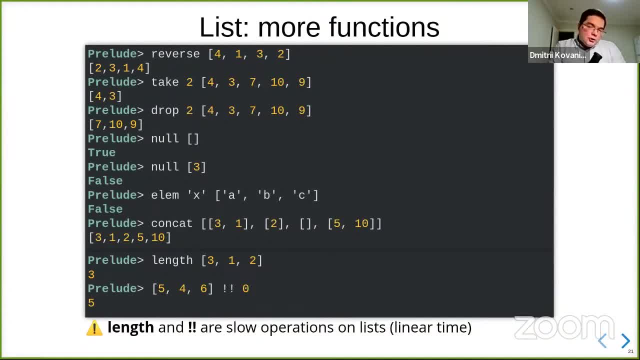 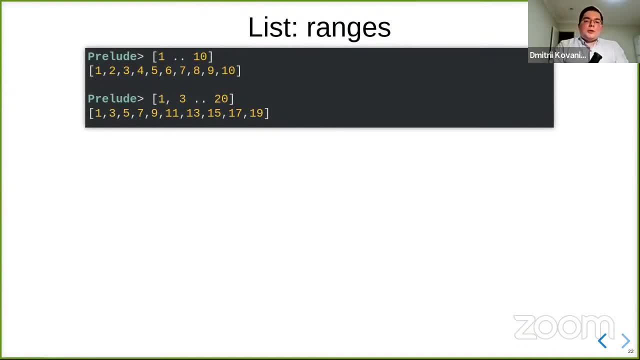 But generally, if it's possible to write code without using this function, it's usually a good thing to do. Okay, There is a nice syntactic feature called list ranges, So it allows you to create elements from one element to the beginning. 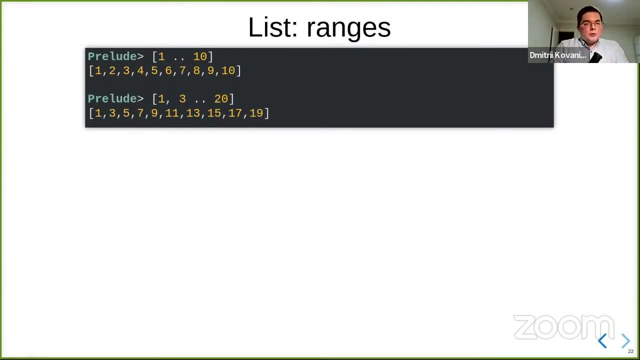 So you just put double dots between two elements, For example one dot dot dot, and we have a list of all elements from 1 to 10.. We can specify a custom step And how we do this. we specify the first element. 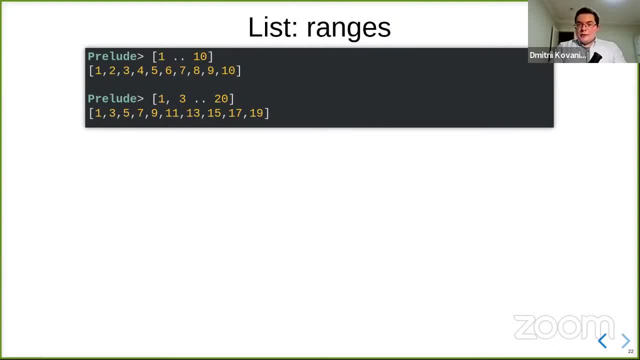 and the second element of the sequence, And Haskell calculates the difference between the first and the second element And it will increase the second element by this difference until we reach the final element. So if you want to have the list of all odd numbers, from 1 to 20,. 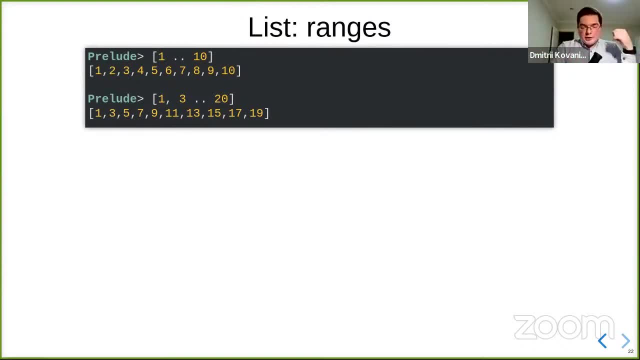 we just write 1,3.20.. Just nice syntax construction. It doesn't work in the opposite way. So if you want to have a list of ranges of elements from the 10 back to 1, like 10,, 9,, 8,- 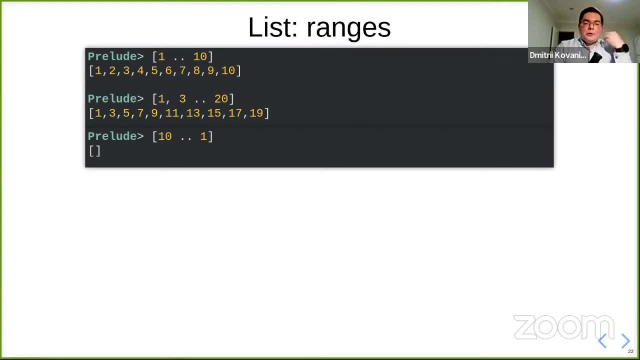 even if you just write this, we get an empty list. And this is happening because the step by default is plus 1. So we get 10, Haskell has to check 11. And it says: OK, both 10 and 11 are greater than 1.. 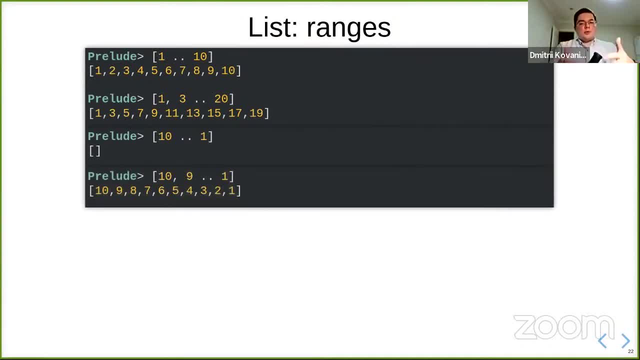 So we just return an empty list. So if you want to have a range in opposite and reverse order, you need to specify the previous time like 10,, 9, and only then 10. And then the step will be minus 1, and you will be good to go. 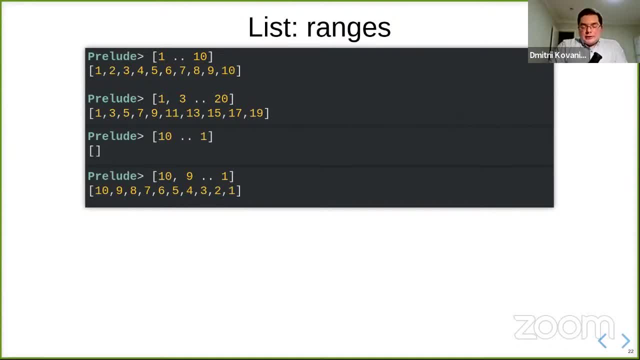 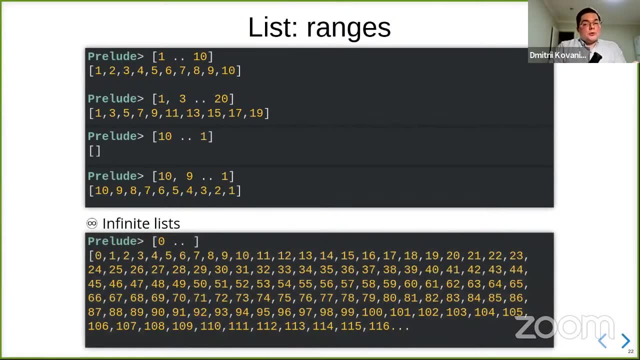 So this is just a nice way to create some sequences of elements going one after another, And we are going to use this syntax a lot. And what's cool, in Haskell you can actually have infinite lists. So if you just write 0, dot dot nothing. 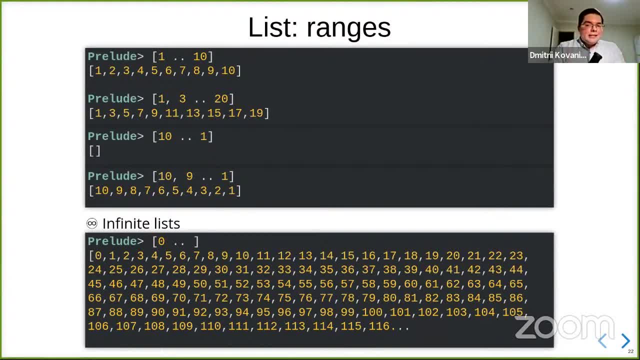 just square brackets and close, you will get an infinite list of all numbers, from 0 to well to the last number. I mean there are infinite number of numbers, so you don't get a list And if you try to print this in JCI, you will see that in JCI. 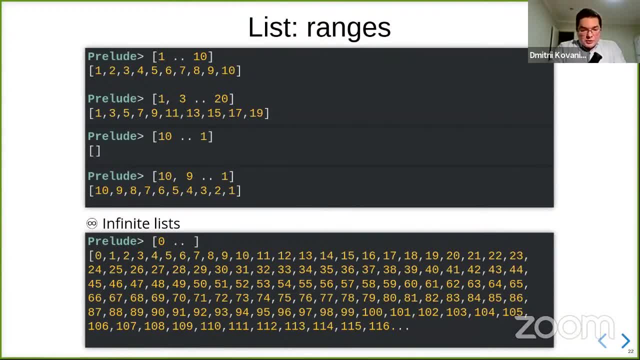 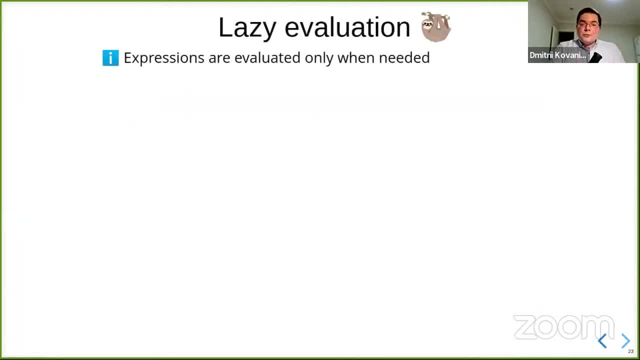 you'll just print all numbers one after another without stopping. So how does this work? This is actually worked because Haskell is lazy And let's look more into lazy. So a lazy evaluation means that values are evaluated only when they're needed. So what does it mean? I need it. 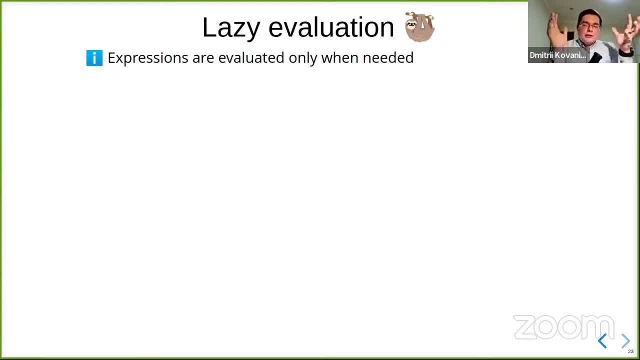 Well, I'm kind of using this vague term needed. I mean in Haskell. people like formal definitions And there is a formal definition. what does needed mean? But for now let's kind of be more intuitive. So now a case needed means I mean we want to evaluate in JCI. 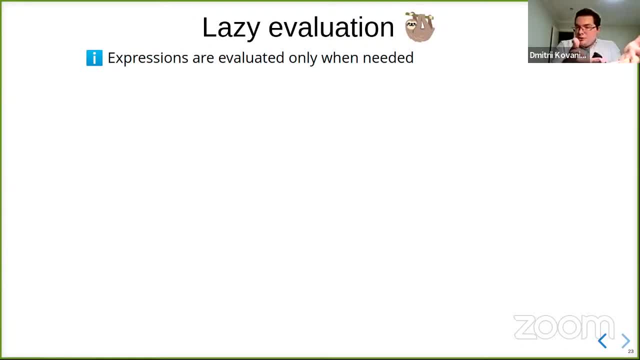 we want to print the result. So if we print the result, it means the value is needed. So if the value is needed and everything itself needs to calculate it, it also will be evaluated, but nothing else. So not more, And which is great because it will save our computation times. 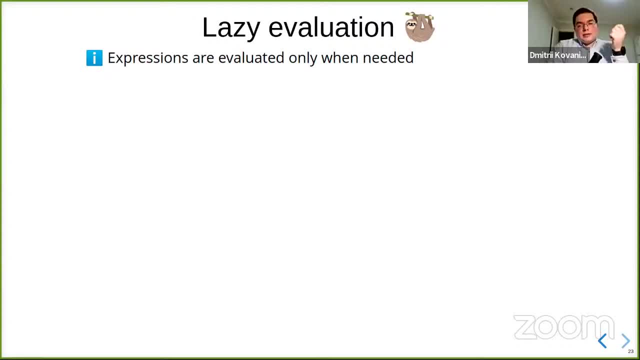 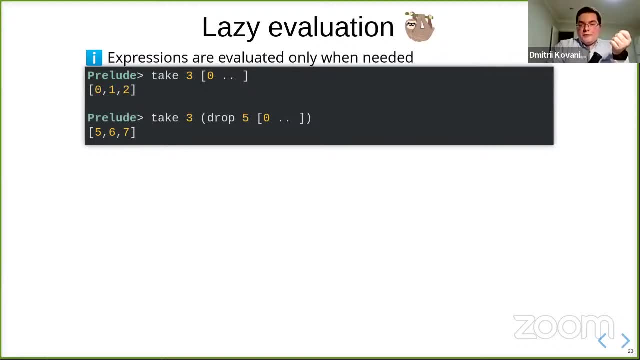 And it will also allow us to have such cool things as infinite data structures. So, for example, if I apply function take three to infinite list from zero, I will get just the first three elements of an infinite list And I don't need to store this infinite list of numbers in memory. 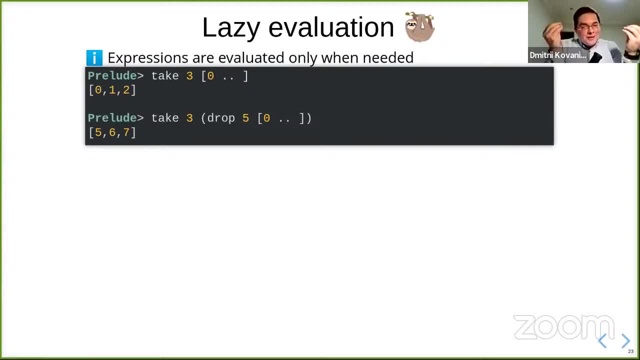 which is great because I don't have infinite memory to store infinite lists in my laptop. but I will get the result immediately And I can apply functions in sequence. And there is, And they compose nicely And I will also get this. So, for example, if I drop five elements from the infinite list, then I take three. 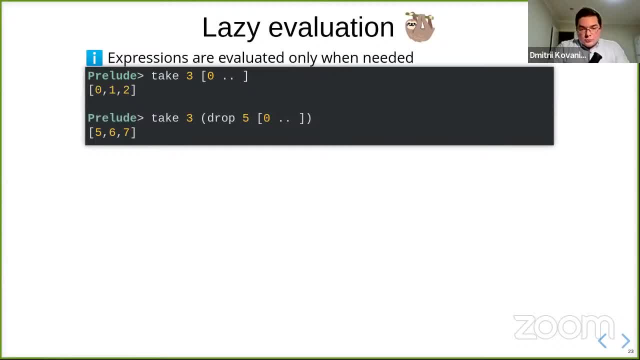 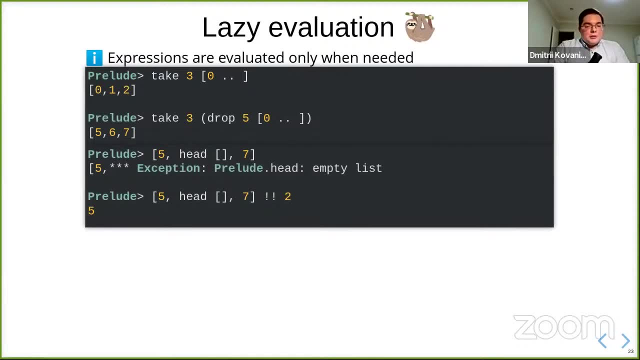 I will get all the elements from five, six, seven, all the three elements. So this works nice. Another consequence of laziness- not consequence, but another feature. For example, we have a list of some elements. So this is a list of three elements: five, then head of an empty list and then seven. 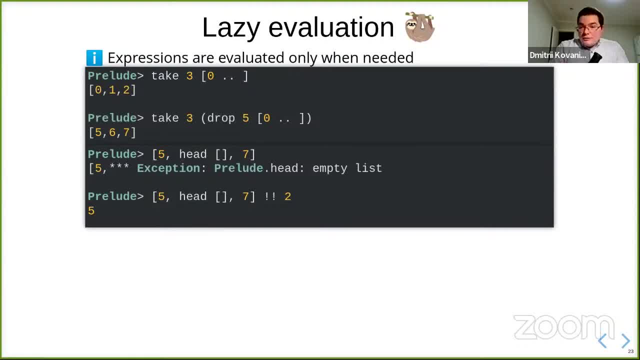 So if we try to print this list in JCI- we'll just evaluate as it is- We will see that It opens square brackets, five comma and exception. So Haskell tries to print the list from the left and it sees that head of an empty list is an exception. 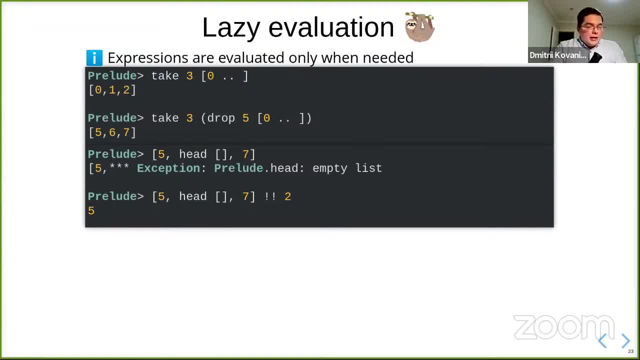 So it just stops this exception. But if I just take the second element of the list, I mean starting from the index zero, zero, one and second. So the third element I will. oh, there is a typo, it should be seven not five. 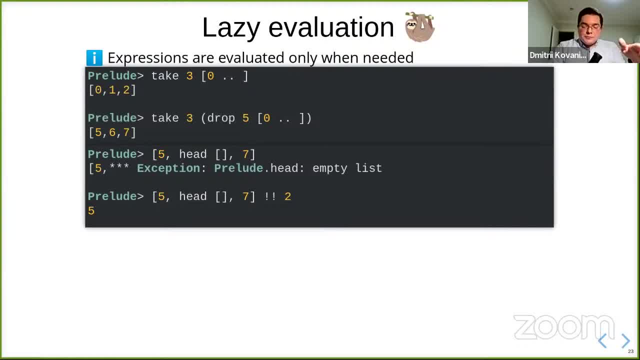 It should be seven. Second element of the list is seven. So actually there is no exception, because I don't need the value Head. I just need the other element, like seven, And this is great because it's not evaluated. So I can deal with this later. 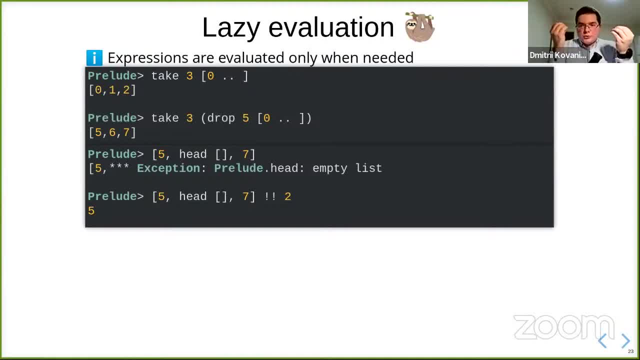 I can do this value And this is what means by lazy evaluation. So we only evaluate values that we need, Even because seven is after of the head. Haskell just walks past this head evaluation doesn't try to evaluate, So it doesn't care. 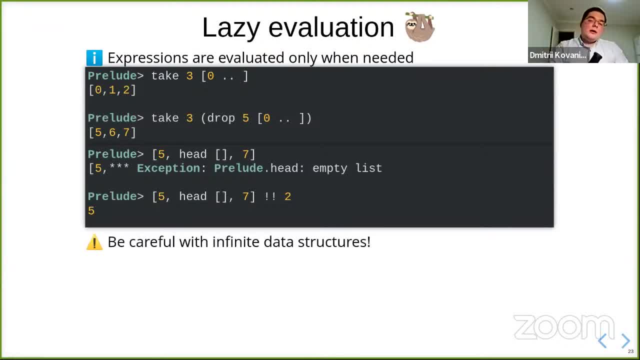 I mean I don't need it, So I don't care, Just leave it as it is. There are some consequences. So, because lists can be infinite, so if your functions work with lists, you can. you now need to think that does it really work with infinite? 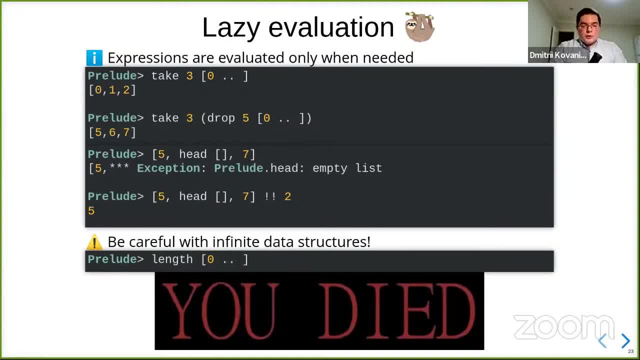 So not all functions work with infinite lists. If you want to, if you try to calculate the length of infinite lists, your computer will hang, because I mean it's not possible to calculate the length of an infinite list. So that's why also, length is not encouraged in functions, because your functions can take up the list. 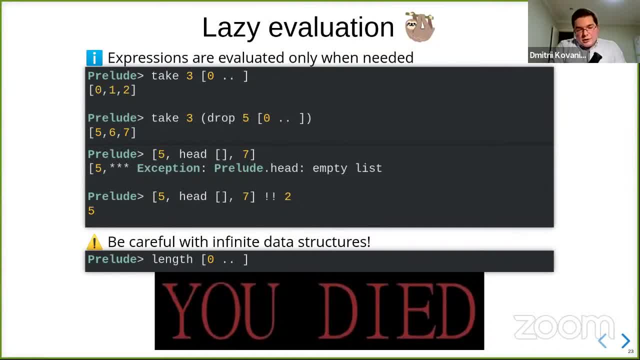 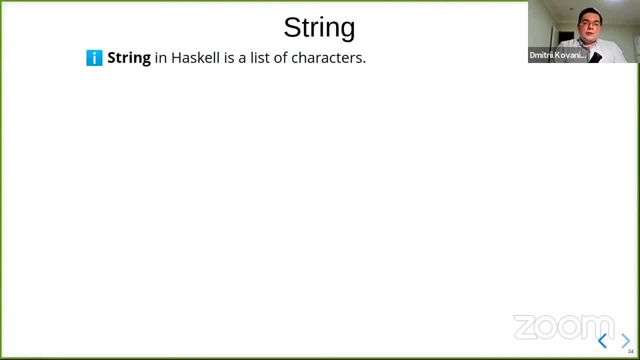 And length will just hang, So just try to avoid. But if you know that list won't be infinite, so there is no harm. So another important data structure in Haskell is string, And in string string in Haskell is actually just a list of characters. 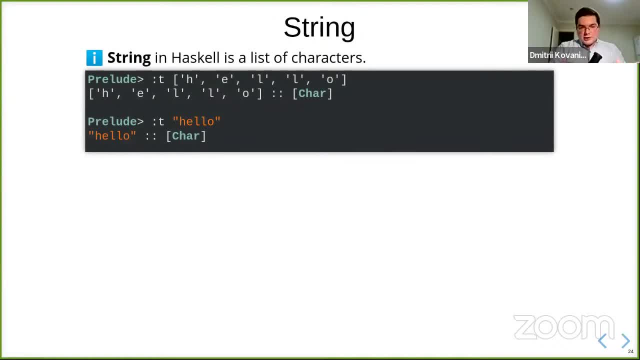 So if I inspect the list of characters put in single quotes, comma separated between square brackets, the type will be list of char characters. But if I just put the string between the double quotes, hello, it's type And there also will be just char. 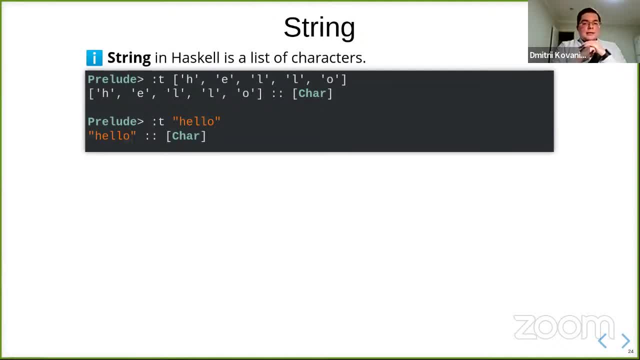 And this is on one hand. Haskellers don't like this because list of characters is not really an efficient representation of strings. So if you want to have like, if you want to do something in production, if you want to worry about memory and performance, there is a better, there are better ways to represent strings. 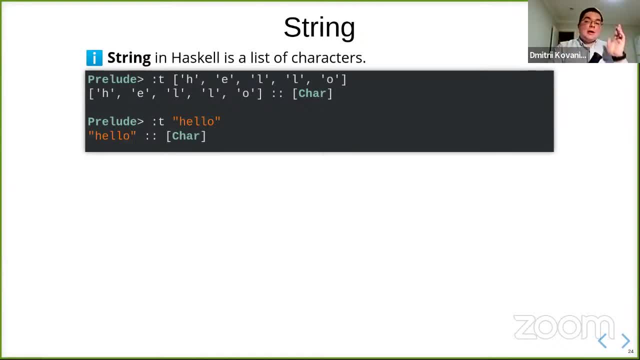 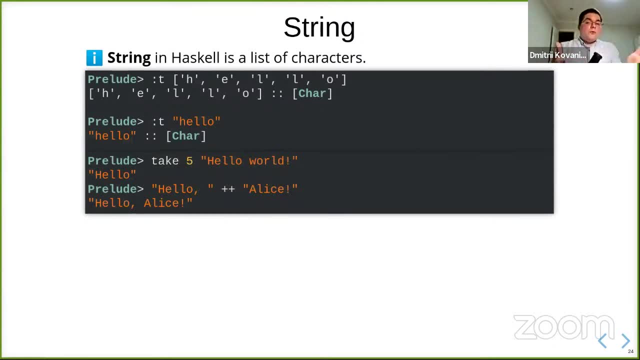 And this is not not far the best way, but it's great for education because, well, string is just a list And you already own no lists, so you can just use all the functions that work with lists on strings. So take, it works with lists, so you can just use it with strings as well. 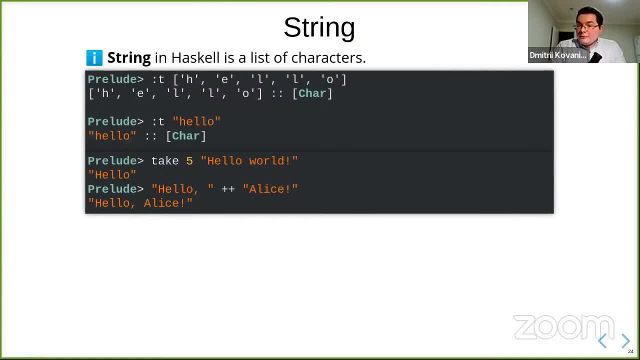 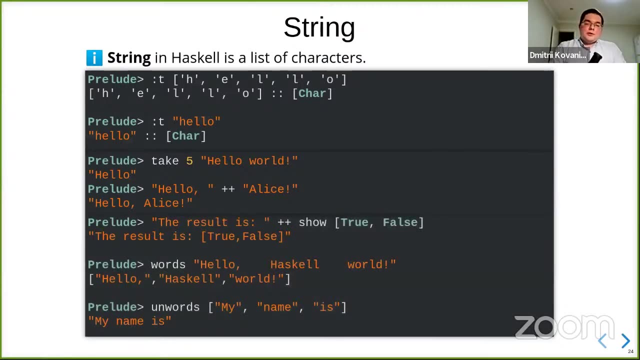 Just take five. hello takes returns you the string and then your first five characters. You can use the same plus plus operator to append to strings, because there is a list and you use plus plus to append the string to lists. There are also specific functions to work with strings. 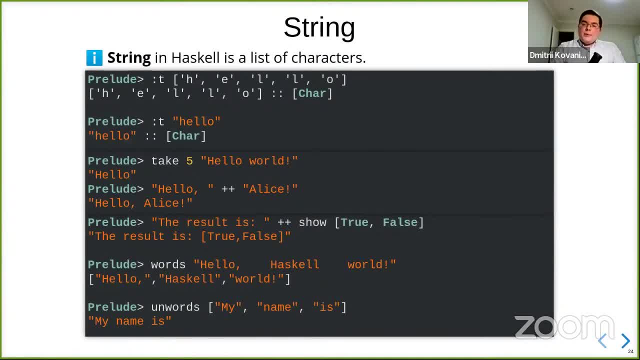 There are special functions: show the take. This is a value and converts it to a string, So it's a polymorphic function. Again, we will talk about it later. but there are also functions that like words, that take a string of words separated by space and it removes all spaces. or like line breaks and returns a list of strings without those spaces. 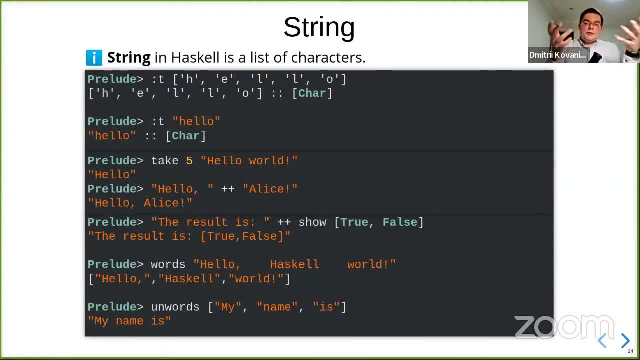 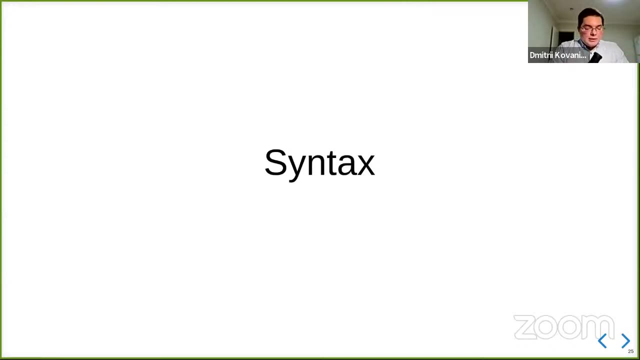 Or the opposite of this function on words. it takes a list of strings and it puts a single space between those words. This is a kind of neat functions to work with string. So we familiarized ourselves with the basic values, steps and we're now ready to write some real Haskell code. 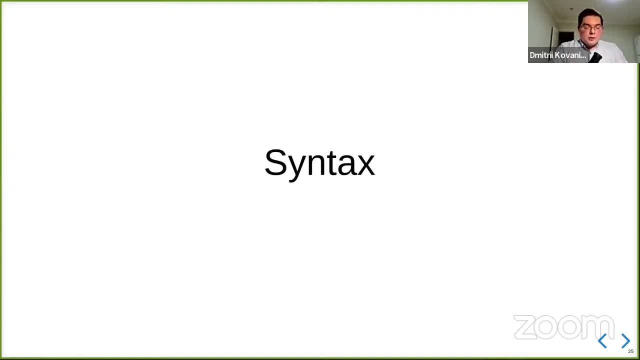 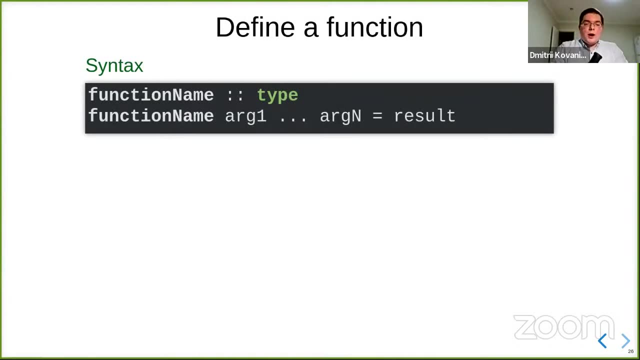 So let's create our own functions. Let's start writing our own functions and writing more Haskell. So the syntax of defining the function is the following: You write the function name, You write double column And then you write type of the function. 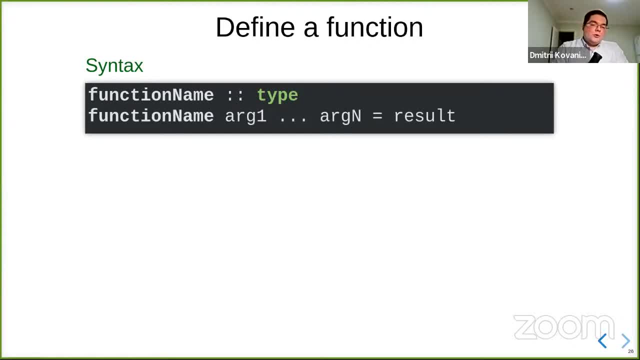 Then on the next line you write the function name again And you write as many arguments as you specified in your type And after the equals sign you put the result: What function returns. So you kind of duplicate the name of the function twice. 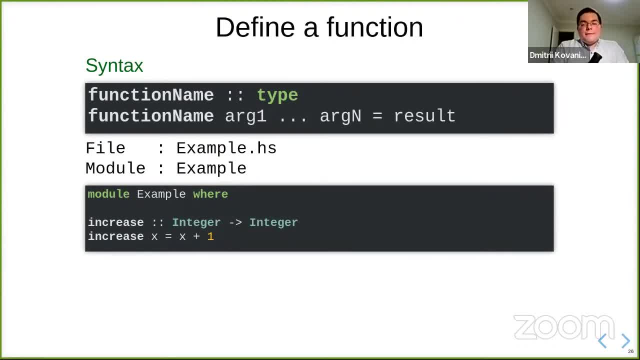 So let's look at an example. Let's create a file called examplehs, And hs is an extension of Haskell. You put in the Haskell files are called modules, So when you write the file you need to start it with this keyword module and the name of the module and the keyword where. 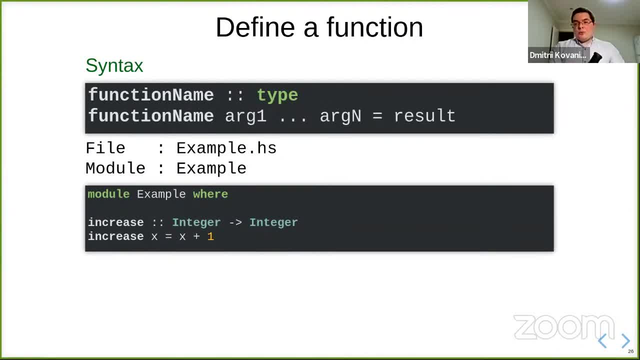 And the mod by convention, by naming convention. Haskell modules should have the same name as files. There are some conventions when files inside some directories, There are some naming conventions. but we don't care about this for now. So we have a module example. 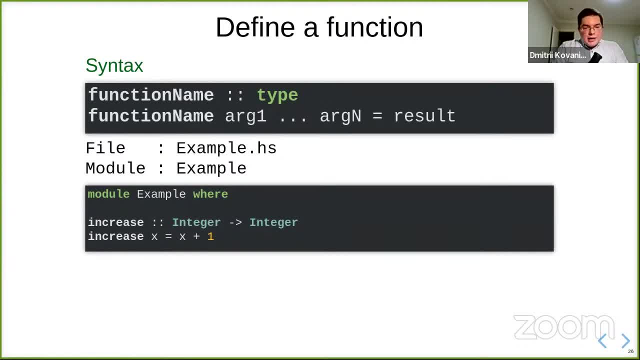 And we write a single function, A single function called Increase, write that name, write its types of its function, from integer to integer, And, sorry, what it does, it takes a number and it increases it by one. So just, we have one argument and it's only one name is what does this function does and how we can now check if it's correct or if it works. 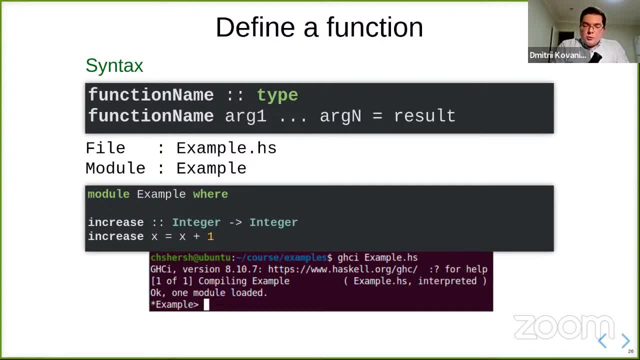 Well, we can. when we call JCI, we can just pass the path of this function to JCI and JCI will load it. It will compile it, As you can see, And it will check for any errors. So there are errors, it won't compile. 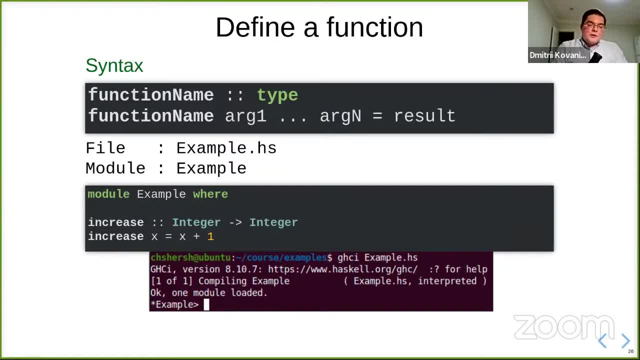 It will tell you the errors, But in our case everything is good And, you see, the prompt will change. It will now say this example, because you are now in the example module And if we now call this function increase of five, we will see that six. 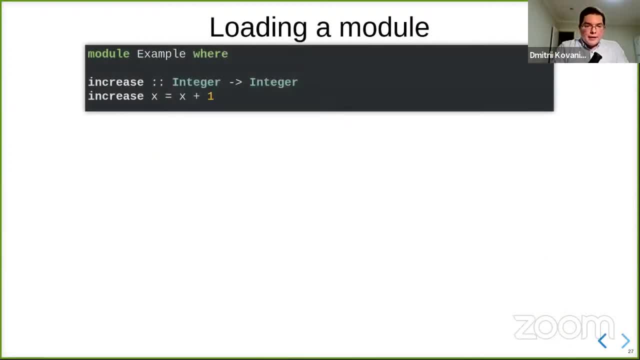 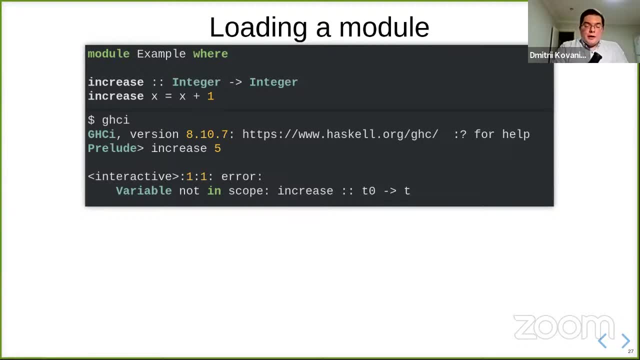 Okay, we wrote our first function and it works. So let's get. if you write the half module and if you just start JCI and if you try to increase the number, we It won't see this function because it's like it's not in scope. 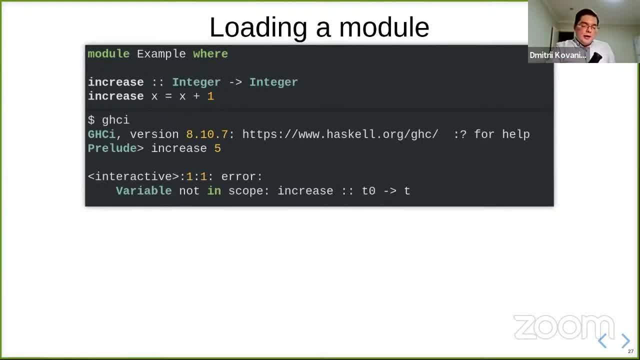 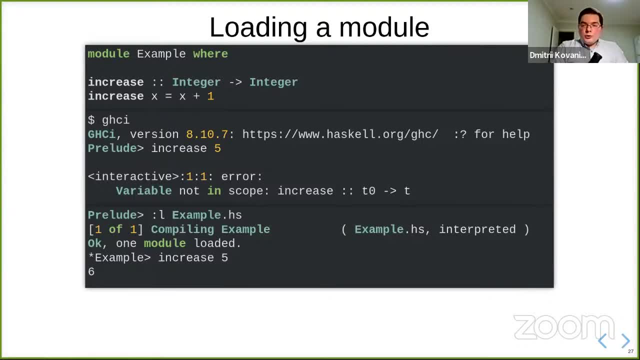 JCI doesn't know where to look this function, So you might happen that you start, started JCI and then you created file. what you can do? There is actually a command called load, which is a colon L, and you can specify the path to a module and or then JCI will load this module and then all the functions that are exported by this module will be available. 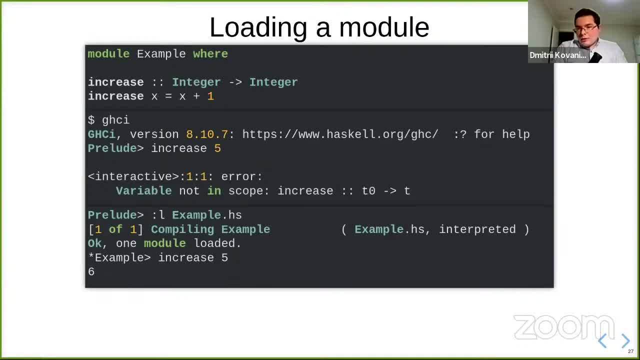 So this is another way how you can load and check. Okay, You can actually have your own custom pretty prompt like not example, not really good, but maybe some pretty lambda or something like that. There is a link for JCI configuration and how you can do this, but in slides I will always use like prelude or JCI prompt. 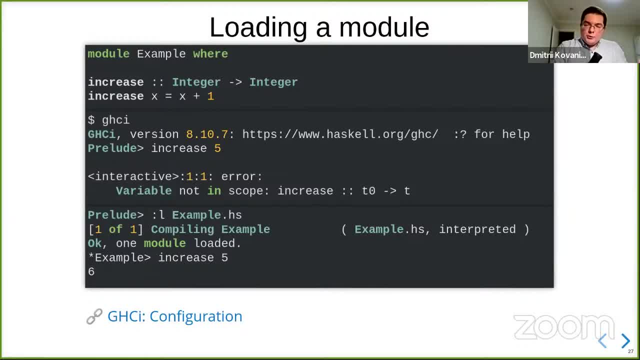 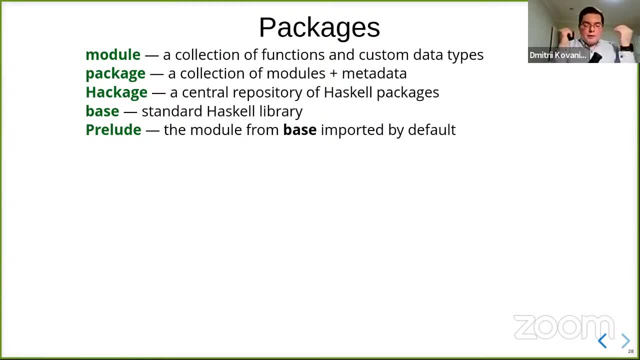 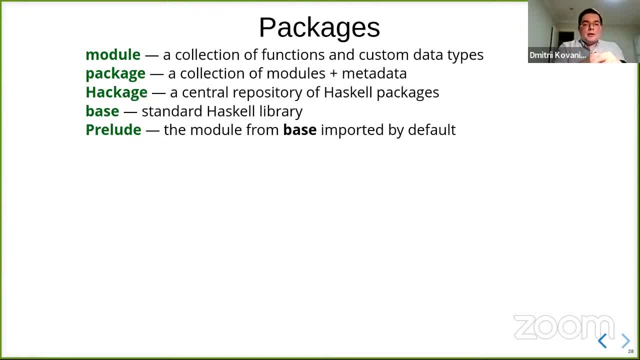 This single file is called the module in Haskell, but now we have multiple modules. So let's say, we wrote several files and we now want to organize them And if you want to put them in like in the same, in like kind of the same idea, you can put them in a package. 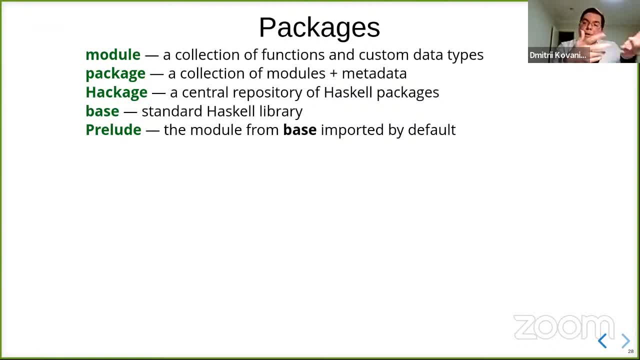 So package is just a list of modules plus some metadata, For example, who is the author of this module. So what is this version, What is the short description and some other metadata. Then there is Hackage. Hackage is a central repository of modules. 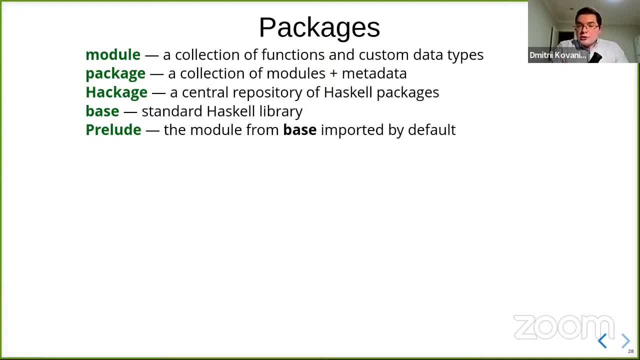 Of all Haskell packages So you can create your own package, You can publish it on Hackage And other people might use your package if they find it useful. And also you can use packages by other people And they're taken from Hackage public place. 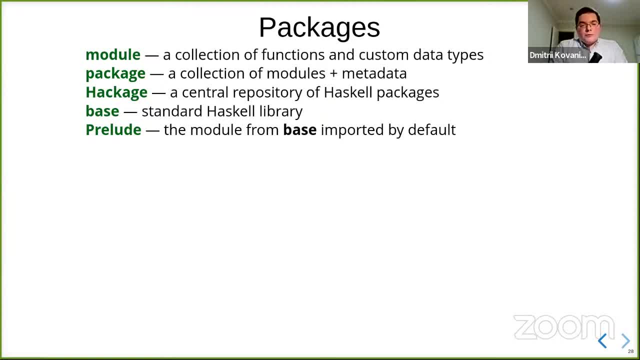 There is like several special packages. One of them is Bayes, And Bayes is a package for standard Haskell library. It contains, like, lots of modules, which is standard library Haskell, And there is special module called Prelude, And Prelude is a module containing all functions and types available by default. 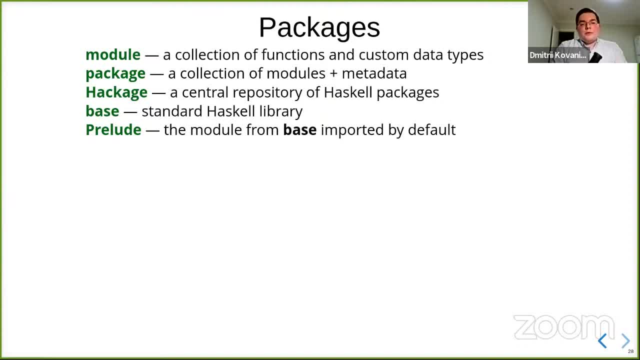 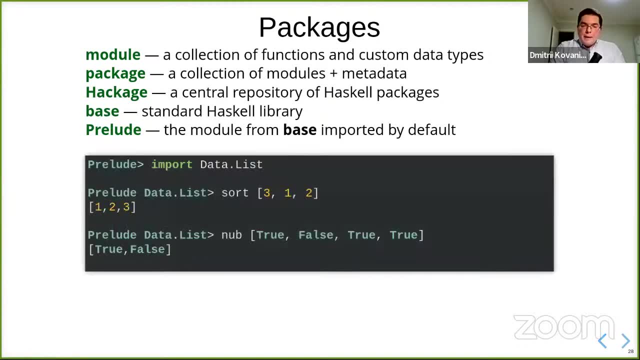 So this is what Prelude prompt means When you start file all the things that are in Prelude module. it is what you can use without requiring any other modules, But not all useful stuff in the Prelude. There are other modules. For example, there is module datalist, which contains other helpful functions to work with this. 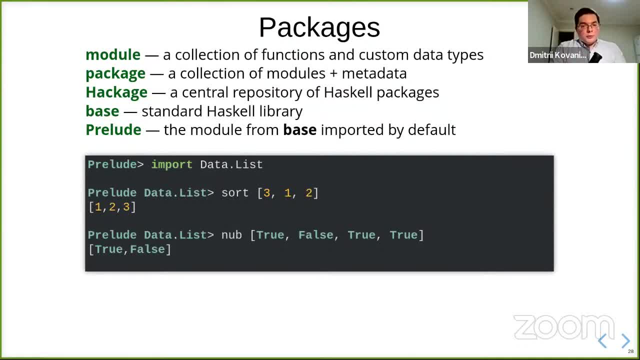 For example, the sorting function. It's not available by default in Prelude And if you want to bring this to scope, you can just write keyword import And write the name of the module And then you will be able to use the function, for example, sort function. 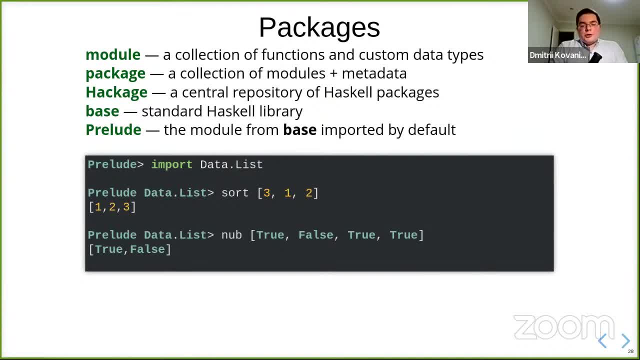 It orders elements and increases order And there is function nap which takes all the unique elements of the list And there are links You can browse Hackage, You can check modules in Bayes And you can see what's in Prelude. 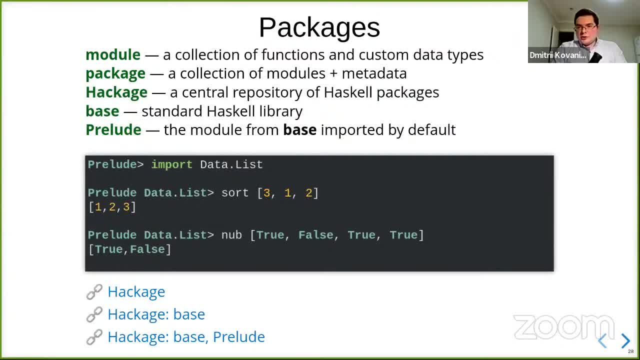 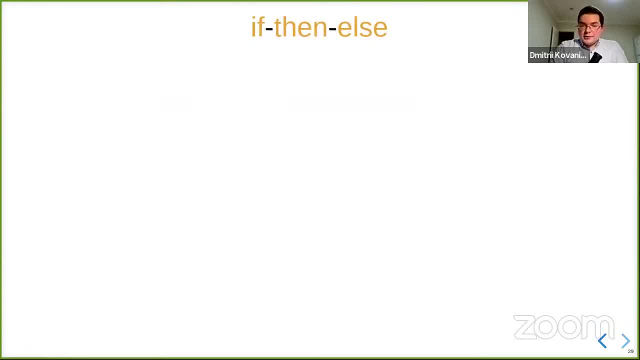 So you may be not able to get everything, Because lots of functions are polymorphic And you haven't touched polymorphism yet, But it may be nice to browse. Okay, Let's dive more into Haskell syntax. So if-then-else is a construction for creating conditional operations. 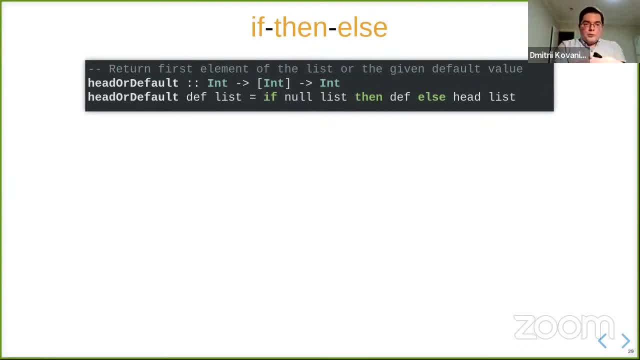 So let's write a function. I'll start the function with a comment, So single line comments in Haskell start with a double dash. And what we want to write? We want to write the function which we want to prove hat. So hat throws exception on an empty list. 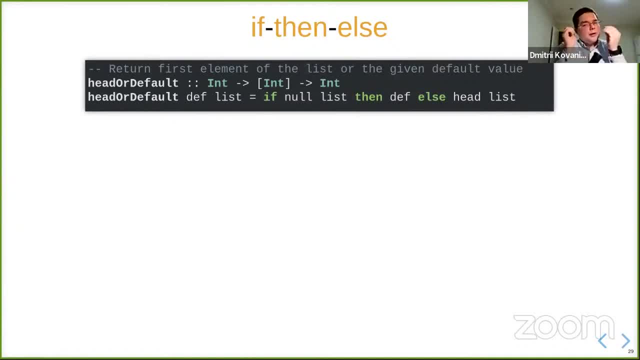 And this is unacceptable. We want to improve How we can improve. Well, one way we can do this is by creating a function that takes a default element that it can return when the list is empty. So let's create our function called hat or default. 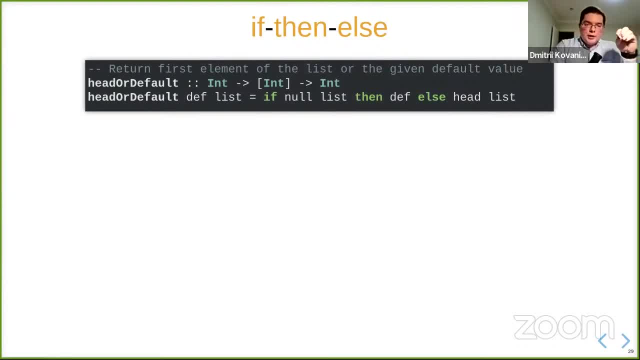 It takes an integer. So I'm not using integer, I'm using int. This is like a different presentation, more complex, more efficient for memory, But I will use sometimes int because, well, it's shorter, But it's a real type. 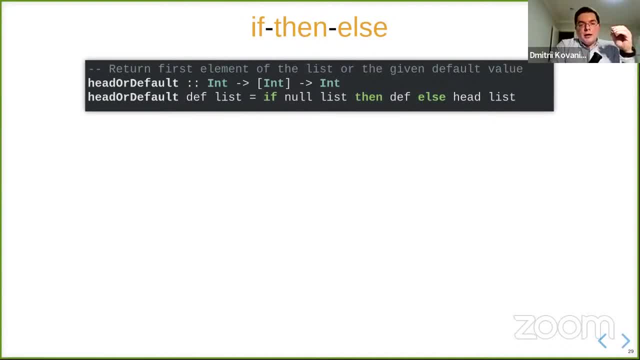 So the function hat or default. it takes an int, default value itself. It takes a list of ints and it returns an int. And it should return like either head of the list or default element And we give names. So of course default element called def. 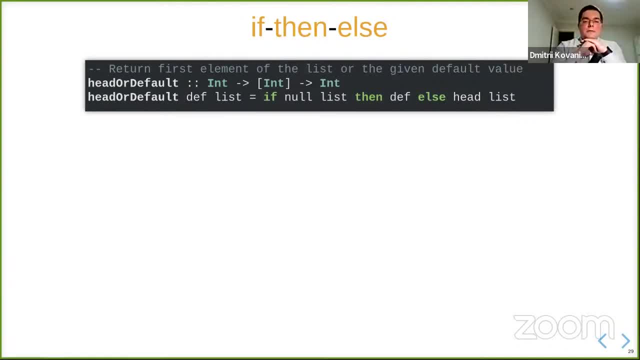 And the list is list. And here how we use if. So we check if list is empty. So remember, function null, it checks if the list is empty. So if function if list is empty, then we return default element, Otherwise else we return the first element. 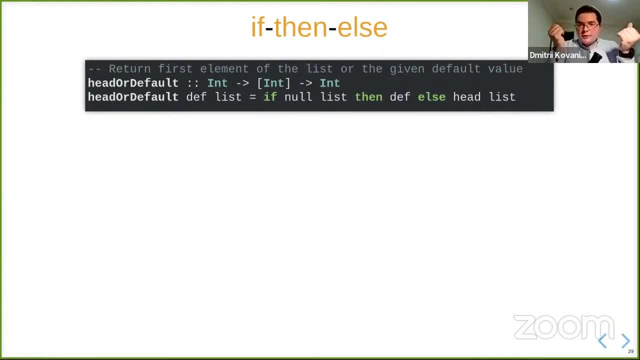 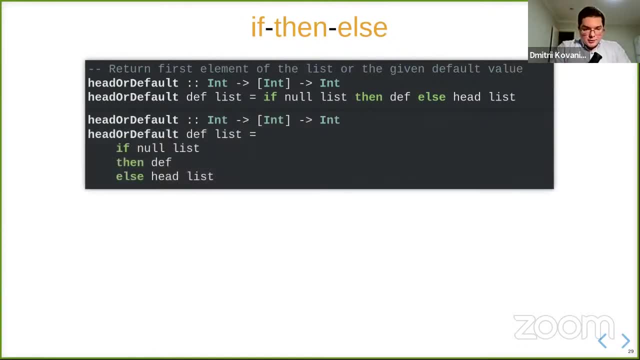 So here hat is safe. Hat is a safe function because we already checked if list is empty, So we can safely use hat. Also, you can put if, and else on different lines, But mind the indentation. So it may be helpful when your expressions become bigger and you might want to put them on different lines. 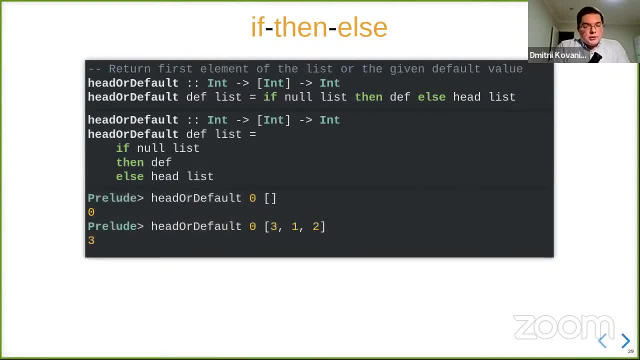 And this function works. So we give it an empty list And we get zero. Oh, if we get no empty list, we get the first element of the list. So important thing to know is that you're You always need to specify then, and else branches. 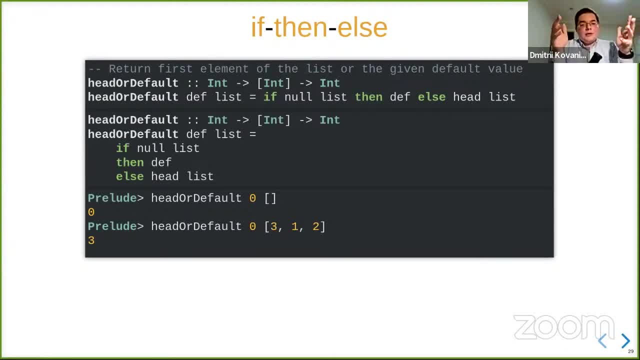 So it's not possible to skip then or skip else. In Haskell if and else is an expression And it always must return some value. So you must always return some value And they both need to have the same type. This is an important thing. 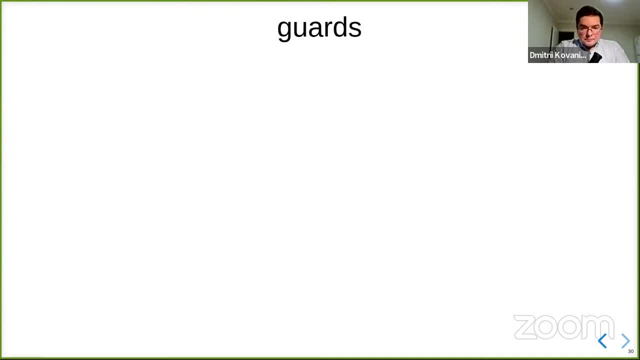 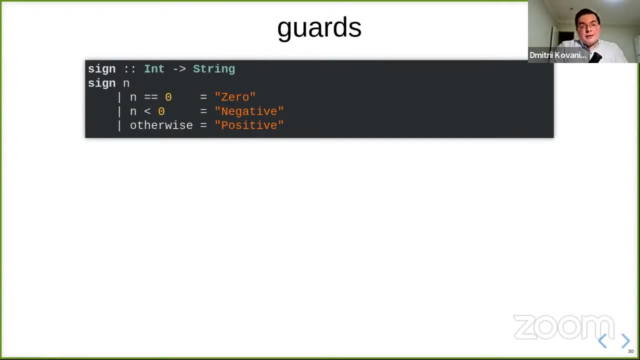 So another syntactic construction is guards, And guards help you to write multiple expressions, multiple conditions, So you can avoid writing nested if and else. So let's say you want to write a function: It takes an integer value and returns the string. 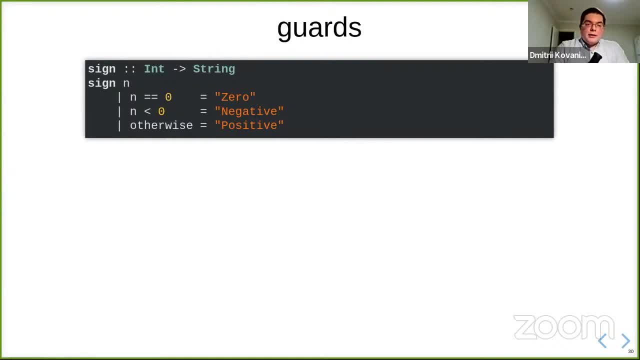 It tells us whether the number is zero, negative and positive, And guards is a vertical line where you put the function. So you write a condition And you write what the function should return on the right side of the equal sign of this condition. 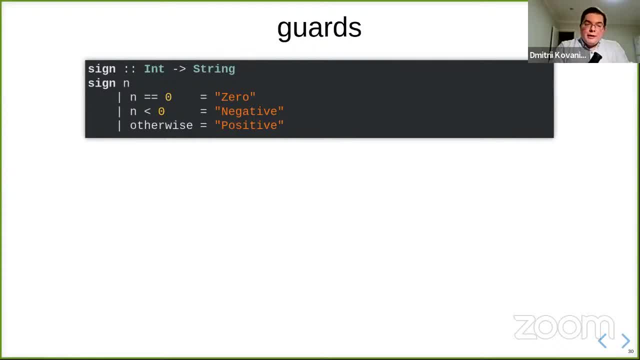 So if the number n is equal to zero, we return string zero. If the number n is less than zero, we return the string negative And otherwise we return the string positive. So usually all the guards end with otherwise, with otherwise. this is like a final condition, what the function should do when all conditions fail. 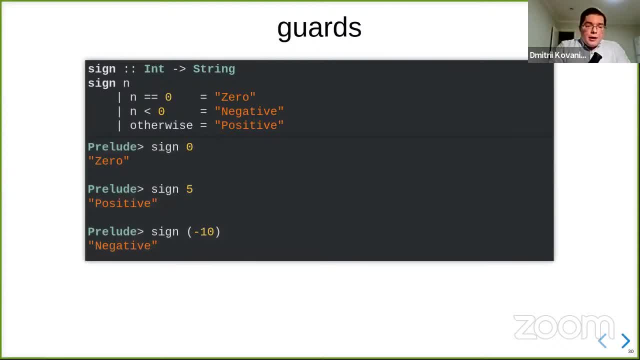 and you can see that this function works. and what haskell does? it checks all the condition from top to bottom, from the first one, and when it finds the first condition that returns true, it just returns them a result of this function on this little condition. this is a nice syntax when you need. 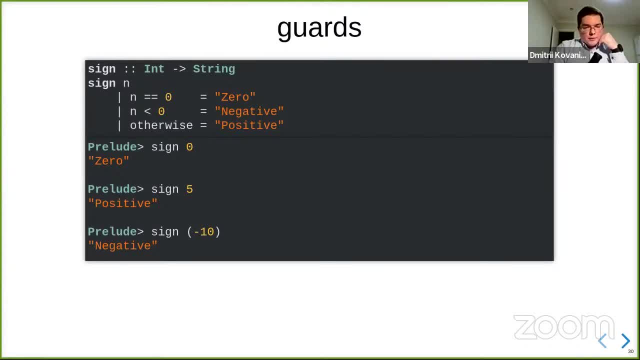 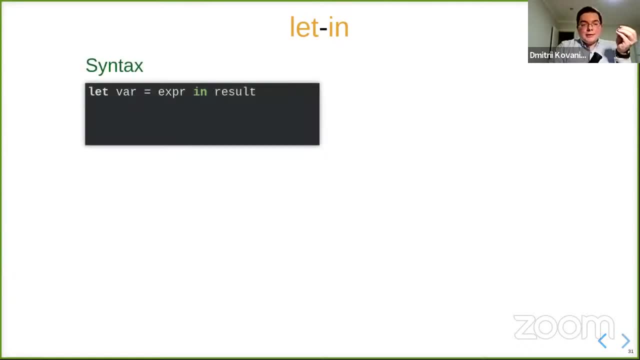 to check multiple conditions on the start of the function. okay, so let in is a way to define your own variables in haskell. so the syntax is the following: you use a keyword, let you name your variable some name. use a sign, not sign. you say what expression equals to and then you use the. 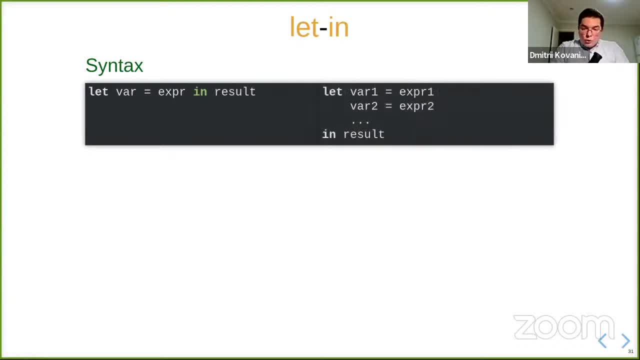 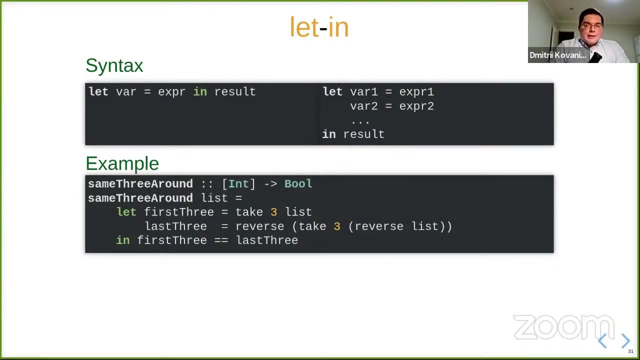 keyword in and return some result. or if you want to specify multiple variables, you put them on a separate lines again, uh, keeping the intonation uh like consistent. so let's write. let's look at an example. let's write a function. we want to write a function that takes the list and it returns true if the first 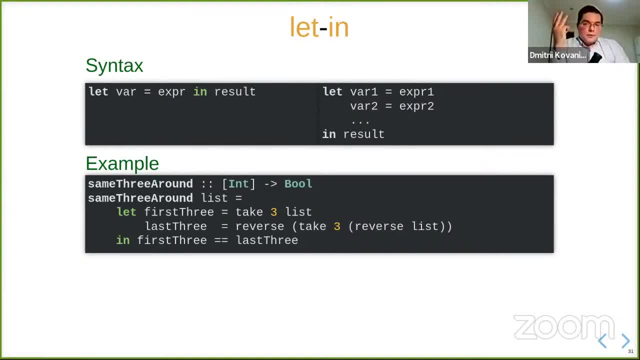 like three elements of the list are equal to the last three elements of the list. so let's see, we specify that it's type is list of ints, like input in square brackets. we see that list and we create the variable first three, which are just the first three elements of the list. okay, it's easy. we have. 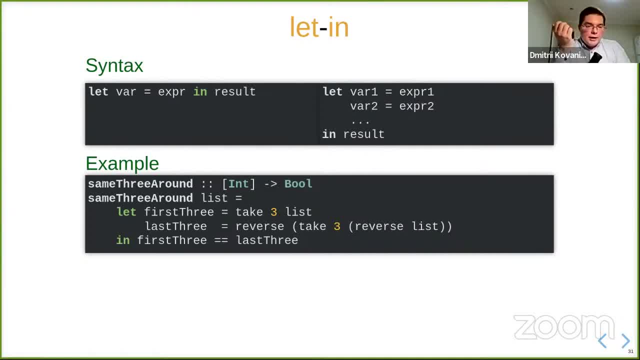 the function take, which takes the first elements of this, and just assign this variable to the result of. we are assigned to first three, the result of applying function take three at least, but how to take the last three elements of the list? well, it's more difficult. there is. 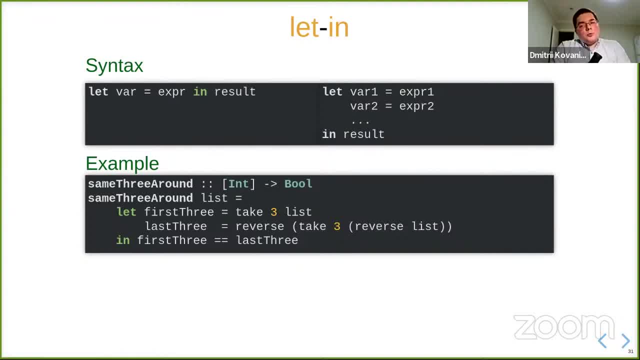 no function for taking like last three elements. but what we can do, we can reverse the list. first, we can take them three elements, so this will be three last, but they will be also in reverse order, because we reverse this and then we took three, so we need to reverse. 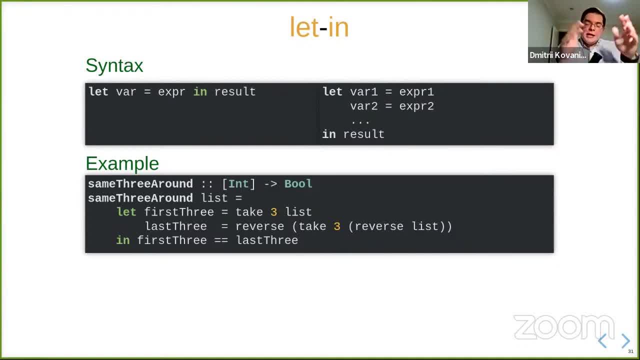 again. so you can see, this expression became kind of more complicated. it may be not the most efficient way, but it works. and then, after the in keyword, we just compare first three elements of the list and again, uh, we see how it works. if the elements not equal, they're not equal, it's equal. 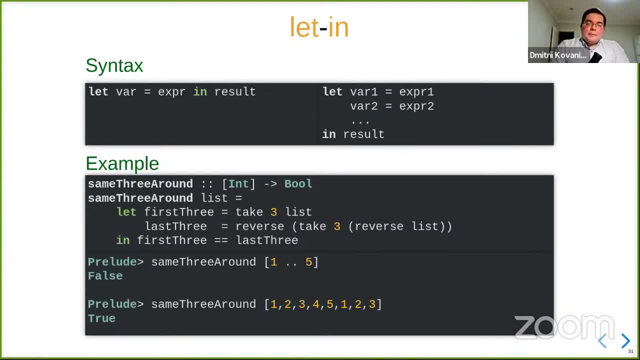 the function returns true. so it's important to know that um in, let there's always. again must be in. so it's just impossible to just create variables. you need to return something. if you assign variables, there is, there should be purpose in this, in sense like you need to use them later. 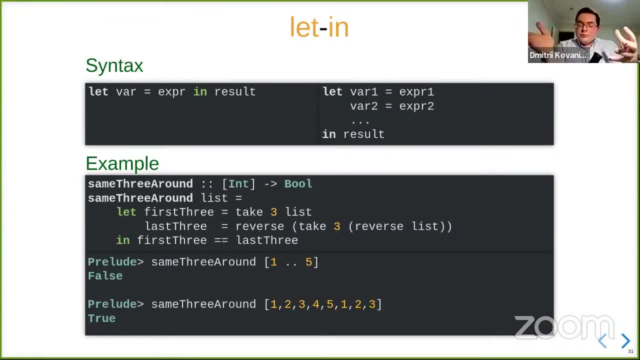 so it's not. it's not possible to just create variables. you just define them to some uh expressions and use later. and you may want to use them be when your expressions become bigger. you see this last three. it's kind of like you call lots of functions itself and when you have lots of uh. 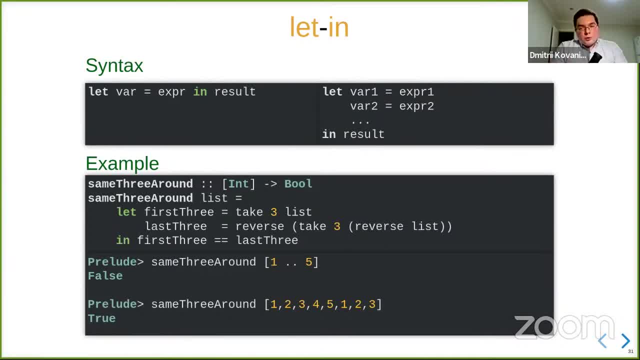 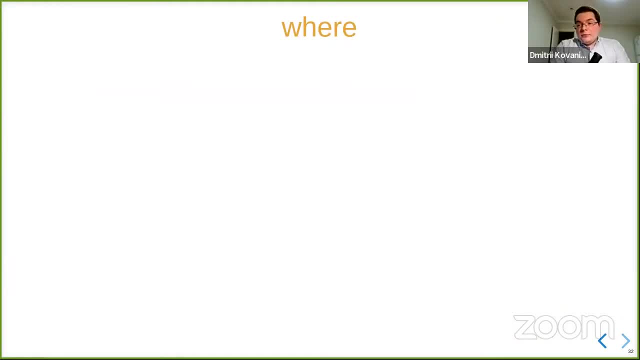 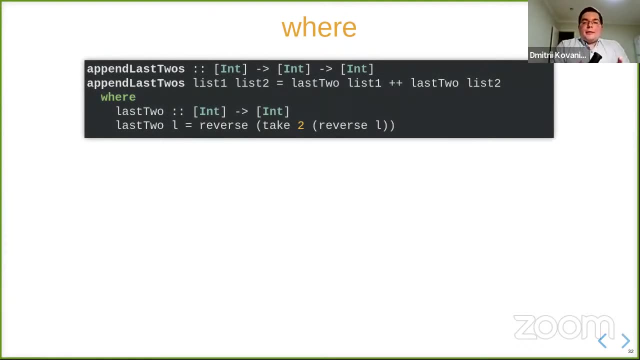 expressions. if, if you have, if you want to use them several times, you might want to create variables to use them. this is where you, this is when you use latin. there is another way to define local variables or even local functions, which is using the where- keyword. and what we want to write now? we want 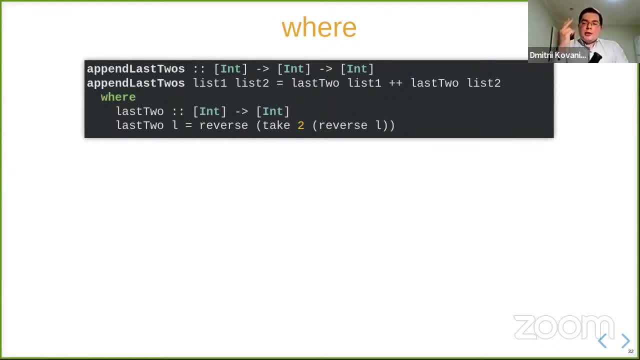 to write the function that takes two lists and it returns another list. and what should it take? it should take the last two elements of the first list, then the last two elements of the second list and just just append those last elements together. okay? so we think, okay, it makes sense to create a local. 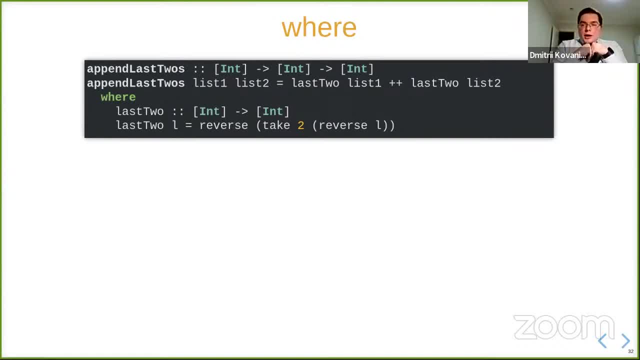 function that takes a list and returns the last two elements of the list and we use the where keyword and we write the type of this function. it's function from integers. you don't need to write type, but i encourage you to write that in the beginning and it's usually a good practice. 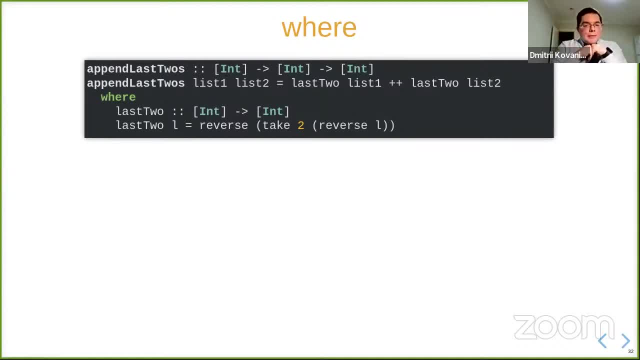 to write types of functions and global functions in haskell. so okay, we know how to take last two elements. we just did this with the previous example: just replace three with two and we get not last three but last two elements. okay, and in our function we apply last two to the first list, we apply last to the second. 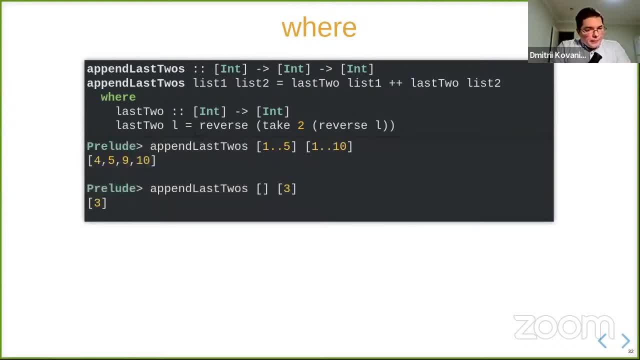 list and we combine results with plus plus easy and it works as expected. so both let and where are ways to create local variables and local functions. i haven't showed both examples, but actually these. both ways can be used for both variables and functions. you can use define function. 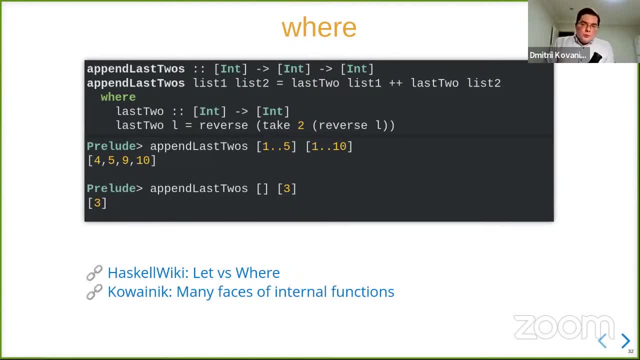 with latin variables as well, so you might wonder so which one to use. this looks like two ways of doing the same thing, but just with a slightly different statistics. what's the purpose of this? sorry, and there is some difference actually between them. i added some things where you can read. 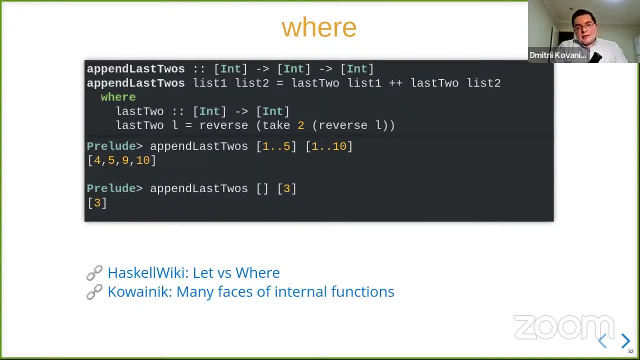 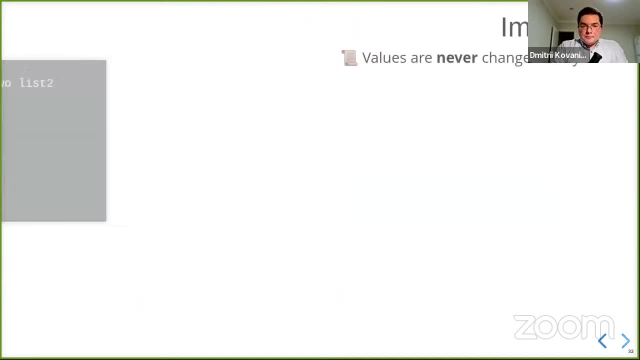 so there was a difference between scopes, which variables i've seen and other. so it's for now. you may use what you find more appealing, what you like more, what syntax you like more, find more reasonable. but the difference i did can sometimes kind of subtle. okay, now let's talk about mutability. so we 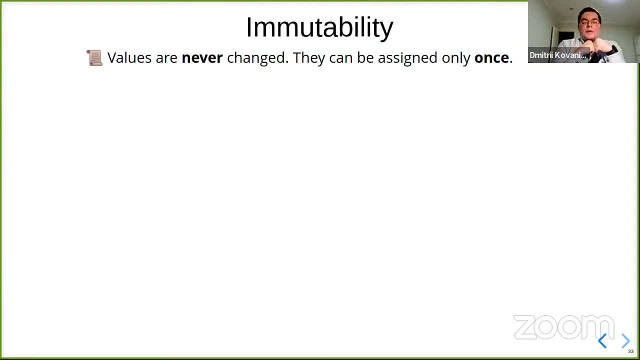 learned how to create our own variables, but, as i mentioned, the haskell is a mutable language. it means that you cannot change your variables. you cannot change values. if it's assigned once it's, then that's all it's done. you cannot change. so what does it mean exactly? 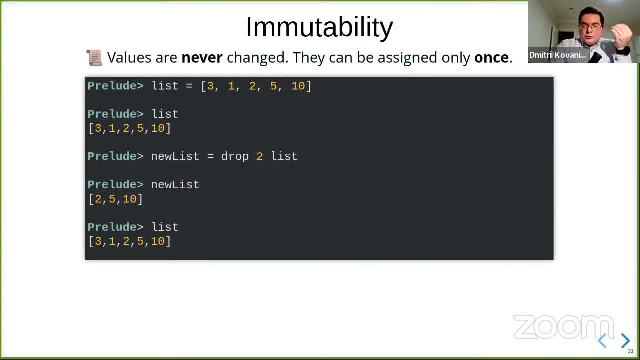 in jhci you can assign some values to variables. we just say: like variable list equals to some value, to some list, and we print in. when you do this just doesn't print anything. so you can just write list again to print its value in jhci and just i will print it list. but now we want to 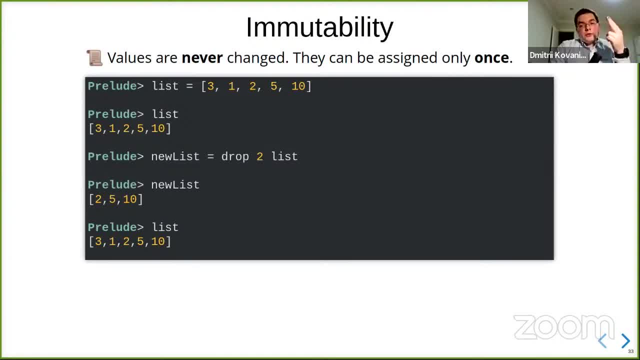 create another list which where we drop first two elements from our existing list. again, jacier doesn't pretend anything. but if we print our list we see, okay, it's the list, but without this end. but if we print the first list again, we see that it hasn't changed. so function drop, it doesn't change. 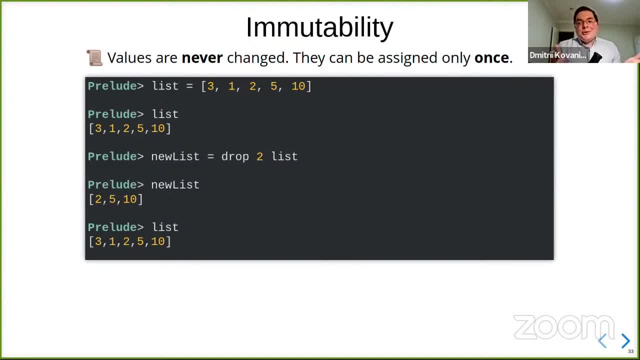 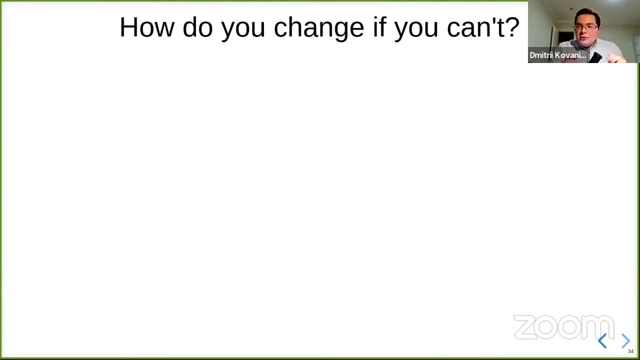 initial list and well, it cannot. in haskell you cannot change values, so how this function can even change this? all values are immutable, so you cannot change. all you can do is you can create new values, new variables equal to new values, and you must say: well, but sometimes i need to change. 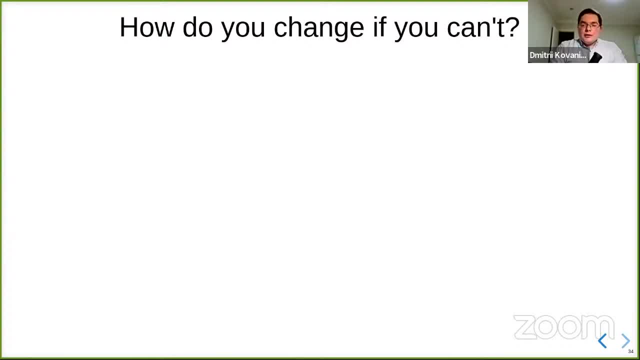 things. for example, i have a list of elements and i want to find the sum of all elements. how do i do that? i will create a variable and i will add all values to this. i need to change this value. how could i do this if i cannot change and the answer is recursion. so if you need to change things, you. 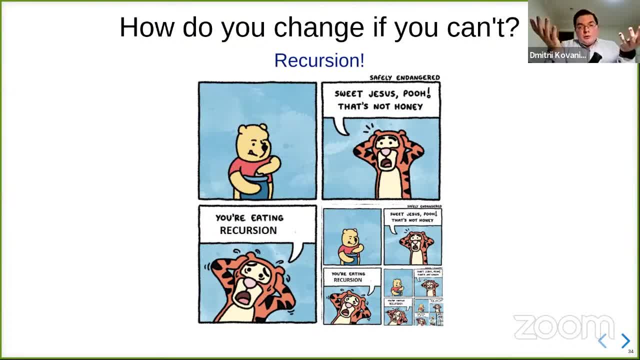 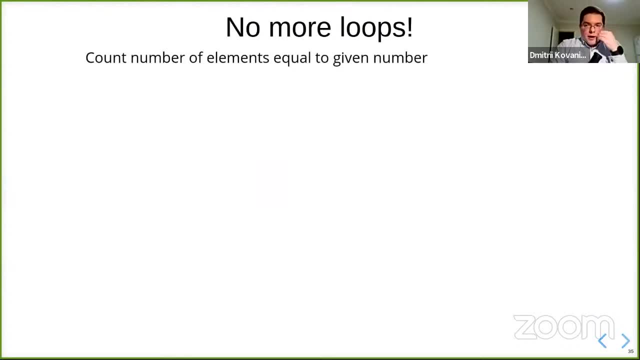 use recursive function. you cannot change values, but you can pass new values to function and you can do this recursively, and this is usually how you can update variables. let's look at an example. so we want to write the function that takes a list and it takes an element and it counts how many times this element- uh- appears in. 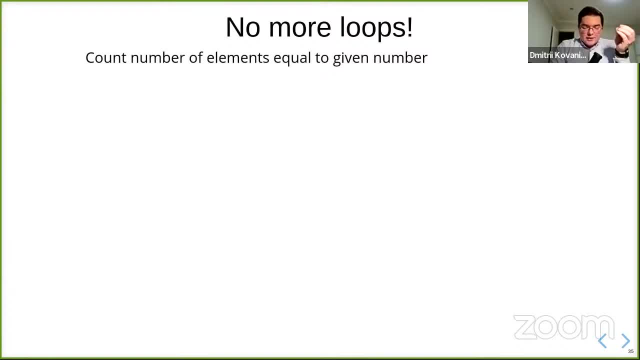 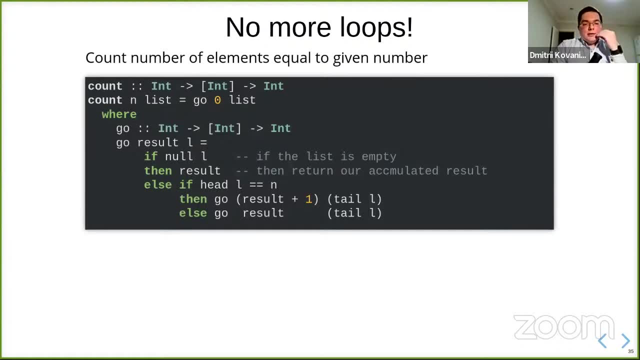 the list. this is going to be so far the biggest function we wrote so fast, but so bear with me what it does. so this function count, it takes an integer number and it takes a list and we want to return also an integer: how many times this element appears in the list. so again, we write the numbers. 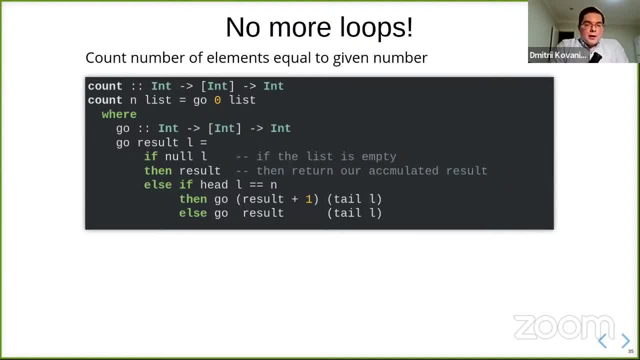 in the list and it takes an integer number and it counts how many times this element appears in the list. so again, we write the numbers in the list. so again we write the numbers in the list. and what we do? we create a helper recursive function called go and we put it inside the where close. this is also 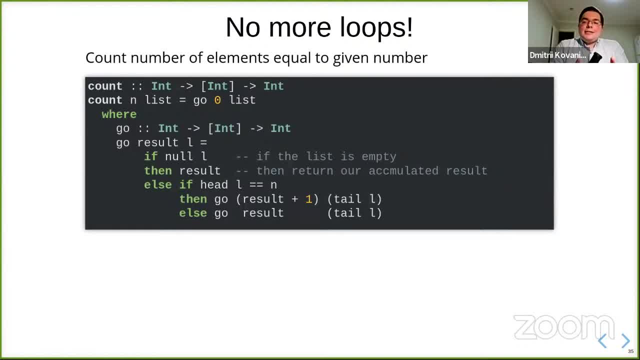 common haskell pattern. so sometimes you need a helper recursive function and you name it go. it's called the go pattern and this function it takes an. it makes an argument which we pass zero initially and this argument tells how many times our element appears in the list. so at the beginning, 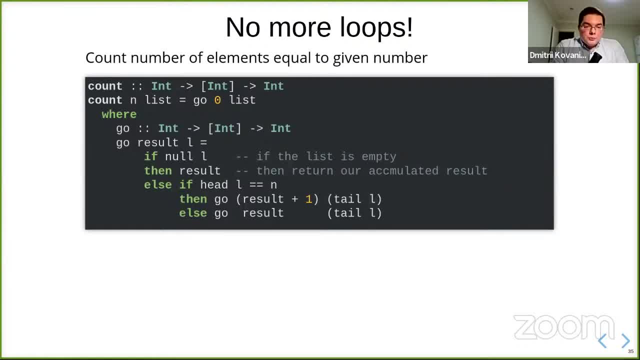 just be zero. so what does our function go? do it again. a result is: uh, the number of elements, the number of times n appears in the list and the list l. so we first check if the list is empty. so if the list is empty, well, obviously there are no more elements in this list. so we just 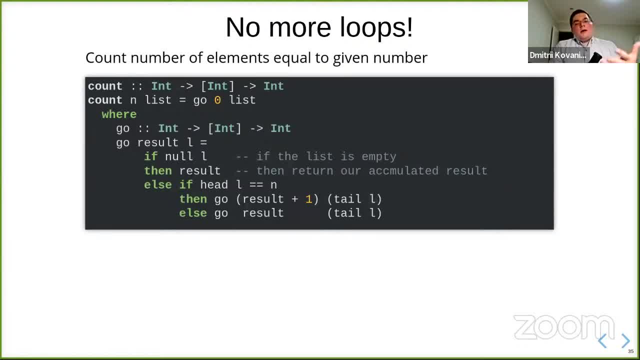 return our result. so you can think that the result is kind of: uh, how many times we've seen the number n so far. so if there are no more elements in this, just return it. otherwise, if the list is not empty, we compare the head of the list with our element n. so again, had the 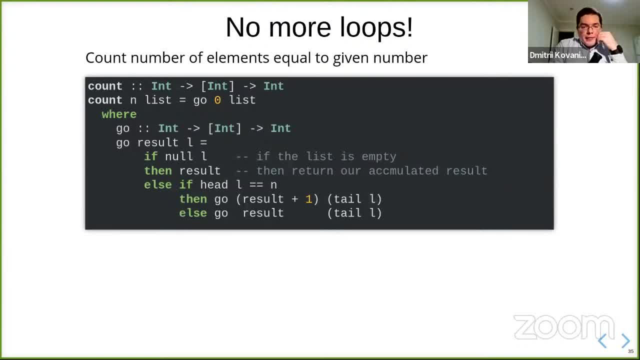 save function here because we used null before and you see that i haven't passed the function and the- uh sorry- the value and to this function go. but a function go can see m because it's in scope, so go is like local function and it can see all the arguments you pass to the account function. 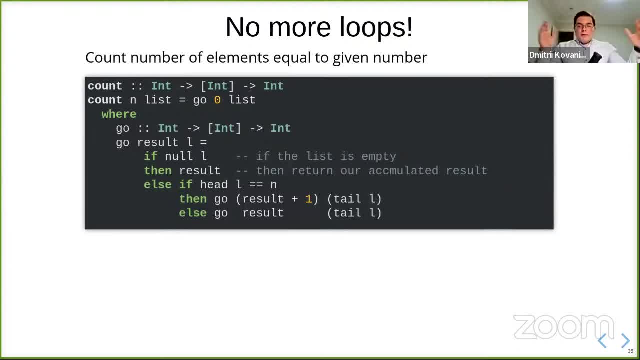 this kind of useful when you pass a lot of arguments to the main function but you need to use them to just have a local function. so we each compare the first element of the list with- uh, our element, and if they're equal like this, so yeah, we found our element. so what do we call we? 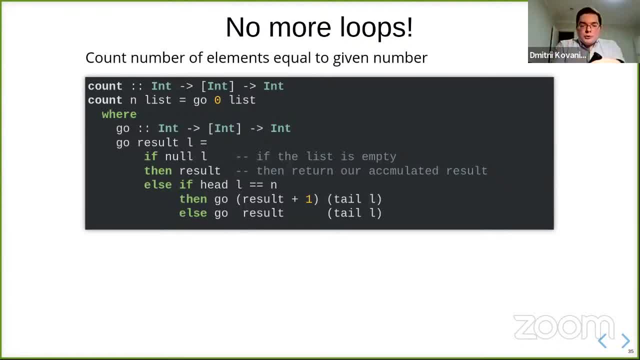 call go recursively with uh- increased result. so we just increase the result by one and we take the tail of the list. so we just cut the first element of the list, otherwise if it's not equal, well, we still haven't found n. so we call go recursively with the with the same result, but still. 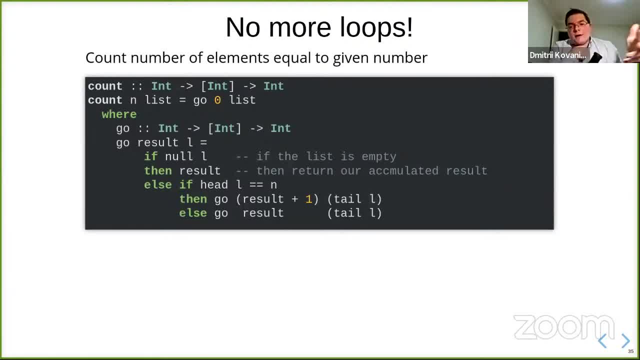 with tail of the list and finally, this function will go recursively through the end of the list. so we just cut the head of the list every time and we finally- um, we'll get to the list. of course, if this is not infinite, if this is on, if this is infinite, we will. we have some problems, so there, 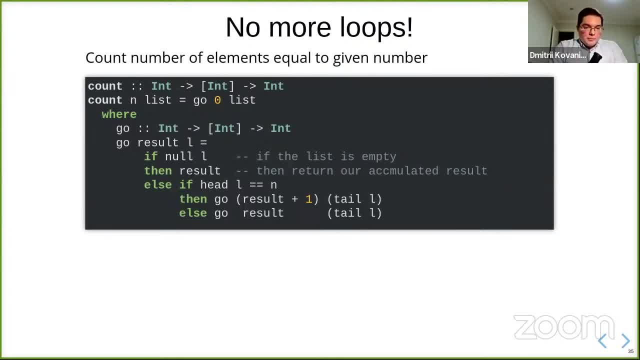 are better ways to write this function. we will definitely write better without using unsafe functions like head and tail, but for now, just the way how you think. so you see, we don't change the values, but we just pass new values to the recursive call and we don't need to change we. 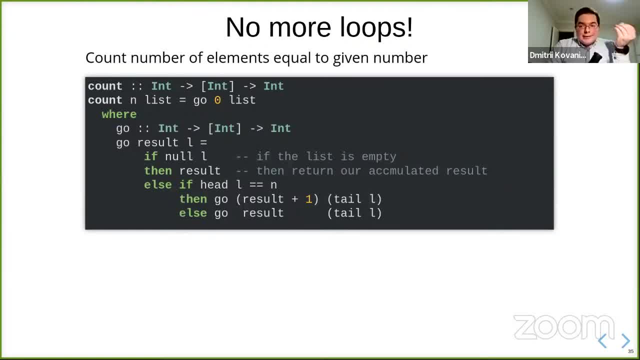 don't have mutable variables, just go recursively calls, and haskell is actually really optimized for this. this is a case of so-called tail call optimization and it actually doesn't allocate like lots of memory or stuff. it's as equivalent as a loop in other languages but semantics could. 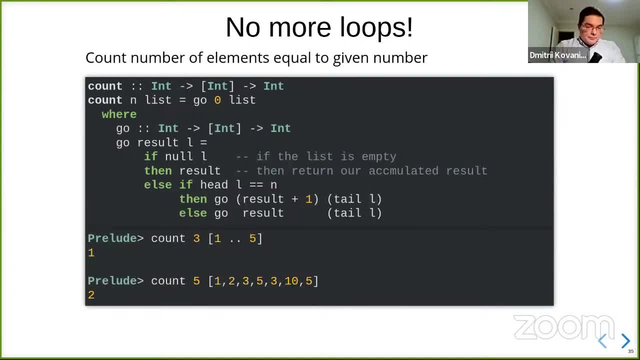 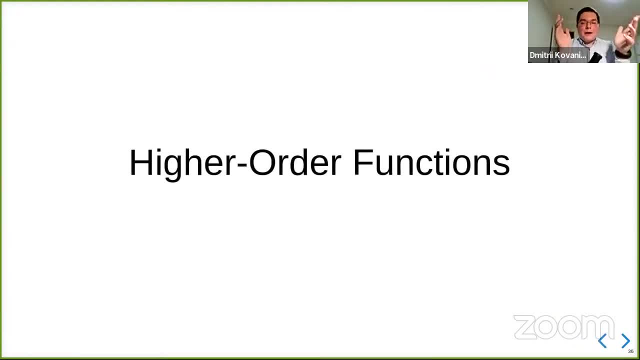 you need to write precaution and this function works, which is great. it would be uh pleasant if it didn't work. okay, so final um part is higher order functions, which is like the main concept of function program. let's let off of this. so in for higher order functions. 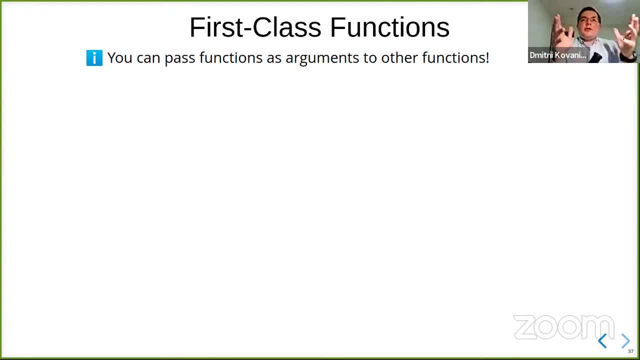 or in other words first class functions, is that ability for functions to take other functions as arguments. so in functional programming functions should be like kind of the same objects as us else, like as ins, and you can pass integers or strings or lists to functions as arguments. but 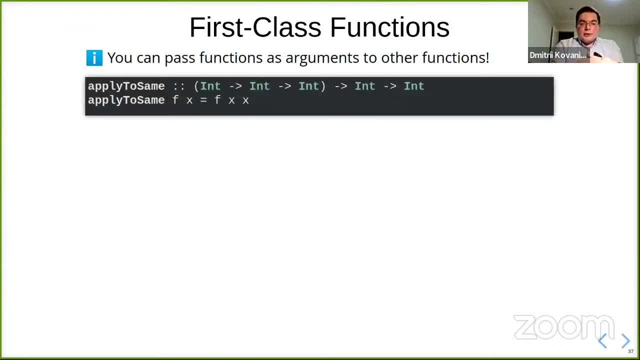 one function is the same object and you can pass integers or strings or lists to functions, to our not pass functions, and actually you can and let's write such functions. so we have a function applied to same. it takes a function, uh, and it puts- it's put in a round brackets, it takes a number, integer. 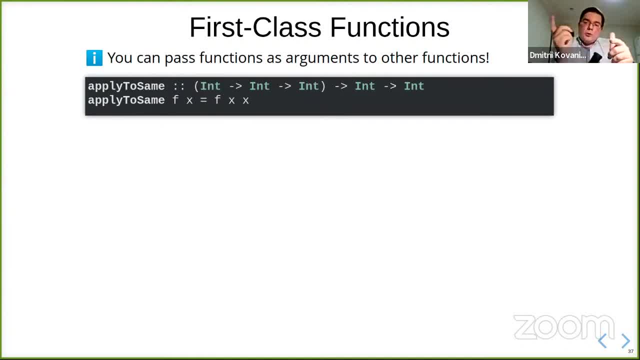 and returns an integer, so it takes only one number. but it takes a function that takes two numbers, so it takes integer, integer and returns integer. and what we want to do? we want to apply this function to a given number twice. so we give a function, we give a number and we apply this function to the 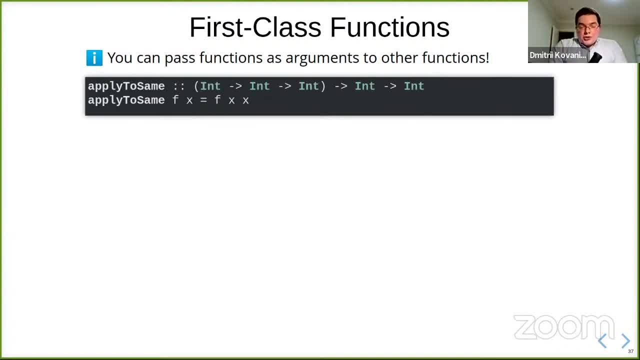 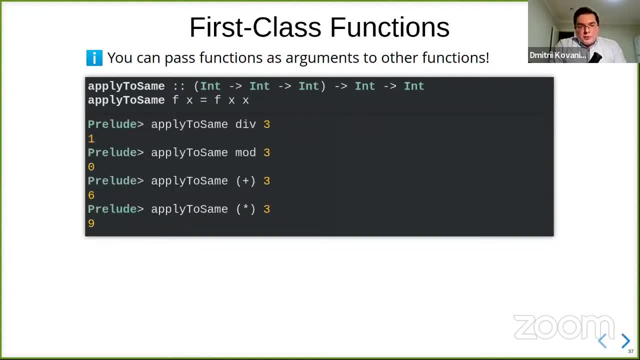 same number twice and again. the syntax of calling function is just putting arguments after the spaces. there is no special syntax. don't need to work. it's just the same as for global functions. if you pass function to an argument and and we can pass functions again without special syntax. 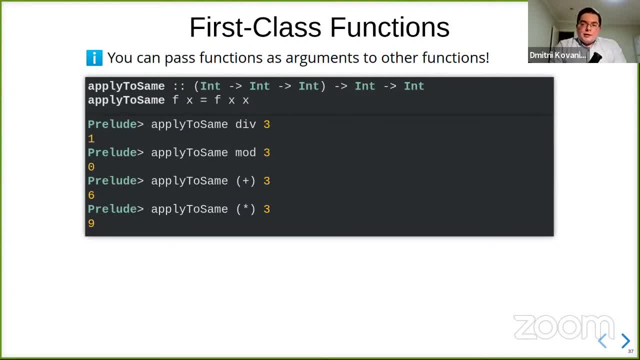 just as it is. we pass function div, which takes a number and divides the number by itself, well, it will always will be one. no much sense, but still example. or if you pass function mod, which takes a module of the same number, again, it will always be zero, but if you remember, 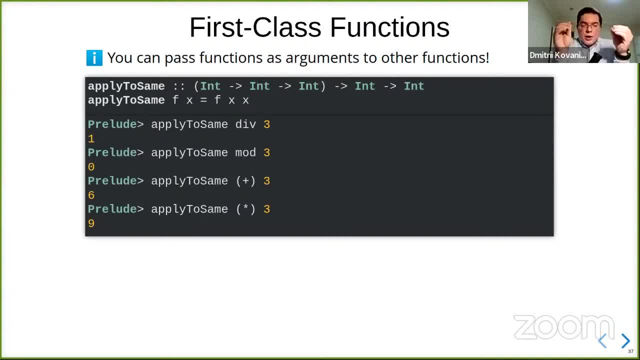 operators are also just functions. so i can put: uh, i can pass an operator plus to the function: applied same. i need to put it in the round brackets here. so haskell doesn't think that i'm not trying to to add: apply to same and three. so if it thinks, if i'm passing this as a function, 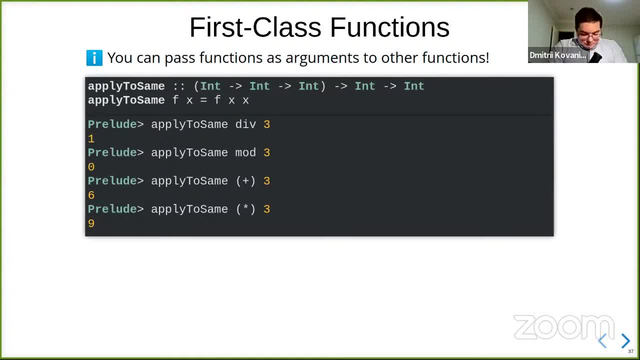 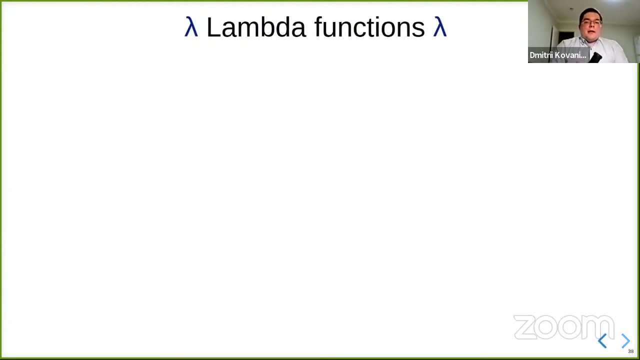 i just put it in round brackets: and three plus three is six, or i can uh pass operator multiplication. so until day nine, so nothing special. we can just uh pass functions as ordinary arguments. uh, usually functional problems associated with lambda functions. but lambda functions, this is not very special, just a function without a name. so you're. 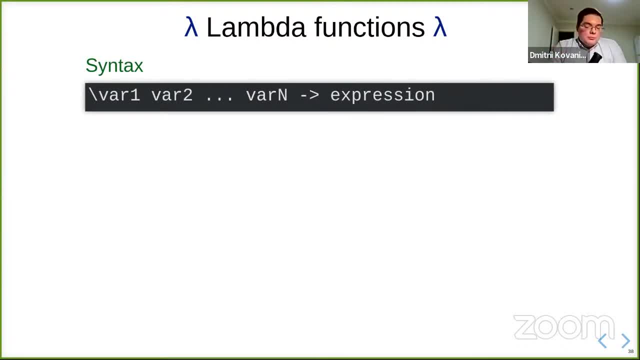 lazy like haskell and you want to have a function but without name, because naming is one of the hardest problems in software engineering. so we can just avoid great name and you can just want to create lambda function or just anonymous function, a different name on the fly and the syntax in. 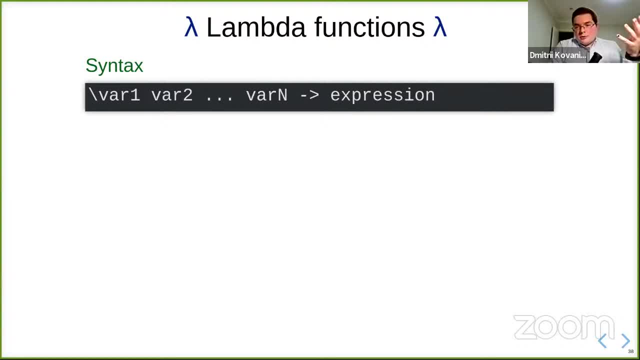 haskell for this is just uh, slash and all the variables for this function, again after, just after space, then the arrow to the right, and what this lambda returns. this is just syntax for lambda functions. let's see, let's first write a function, a higher order function that takes another function, so this function. 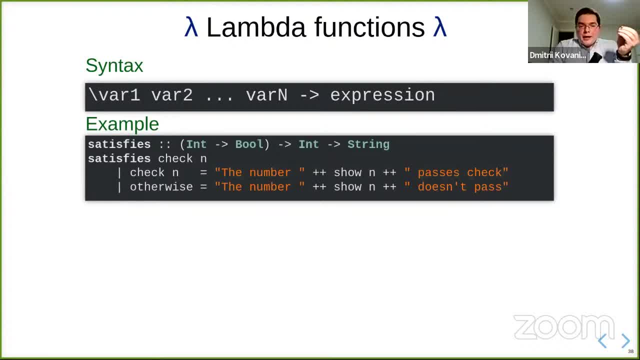 satisfies, it takes a function from into bool and usually such functions are called predicates. i mean function from. if a function returns boolean it's usually called the predicate. so function satisfies, it takes a predicate. it takes a number and returns a string. and what it does? it just checks if the given number, uh, satisfies given predicate and returns one string otherwise. 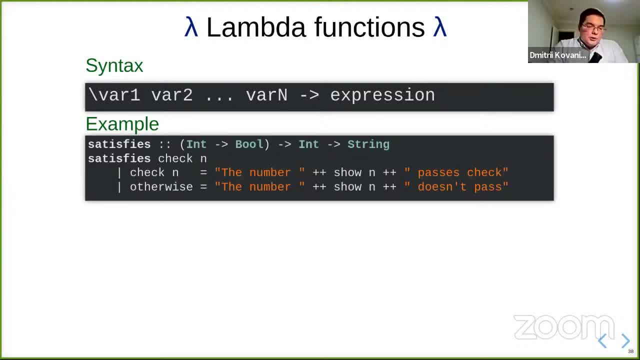 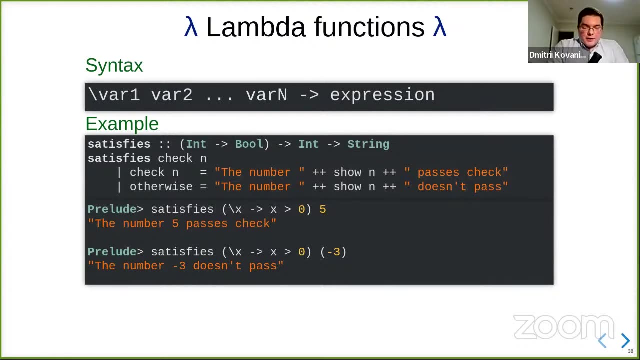 it returns another string. so again, check is just a function and we can use it in guards. we just call it them and it turns bool and if it's false or true- if it's true we will get the number passes check, or if otherwise, it doesn't pass and we can pass a lambda function to satisfy. so this is a. 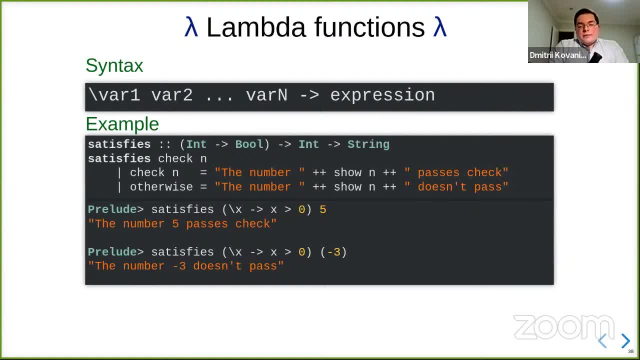 function from x and it checks if x is greater than zero. so again, we might just want to avoid creating separate function because it's just so small. we don't want to create separate function again. and what happens? so satisfies, call this function x greater than zero on five. obviously five is greater than zero. so the first guard works and 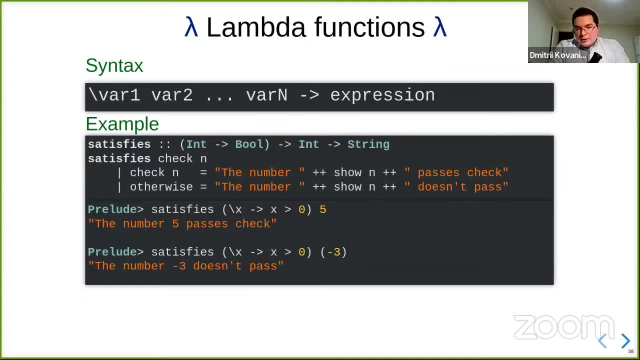 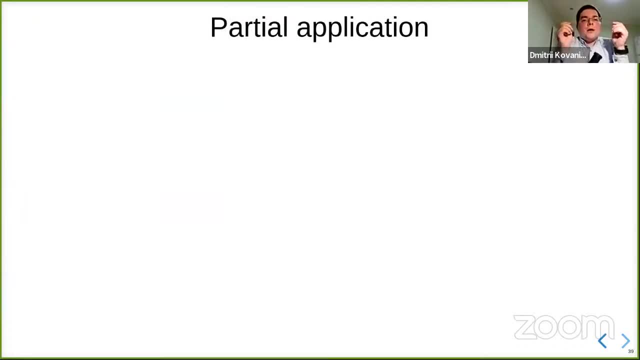 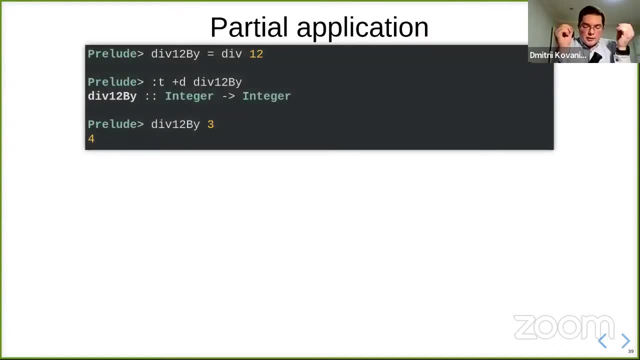 we get the first string, but if you pass on a negative number then we get another string. so nothing special, just uh, lambda function. so uh, cool thing in haskell is that functions can actually be partially applied. so let's create a variable div 12 by what, which is a div apply to 12.. and we 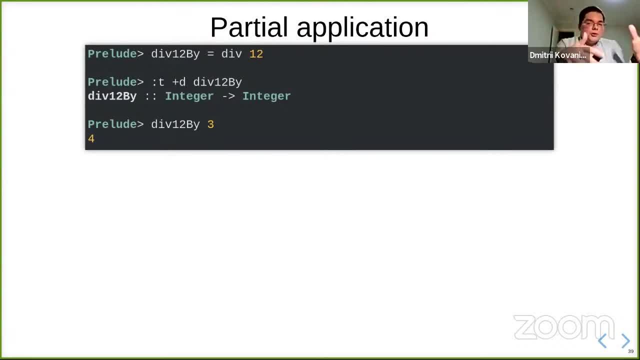 know the div. if we check the type of div, it's a function from integer and integer to another integer. it takes two integers. but if we now check the type of diff 12 by- we see it's have now a function from integer to integer. uh-huh, we applied function to one number and we get another function. 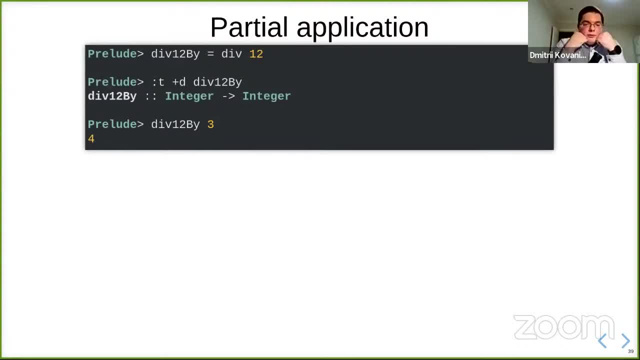 as a result. so just partially applied, and we can apply this 12b, 12 by three and we get four, because we just will divide 12 by four. this is really neat because, uh, you can apply partially functions, then you can reuse them. you can specify some arguments in. 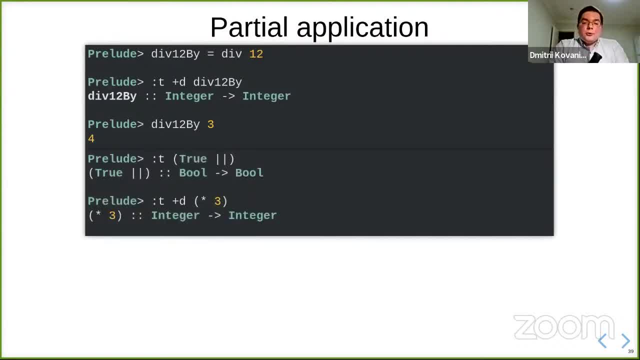 advance. and what is even cooler, that you can do the same with operators. uh well, for operators you can, because, as I remember, operators just functions. but for operators you can put the element on the left side of the operator or on the right side. for some operators it doesn't matter, for 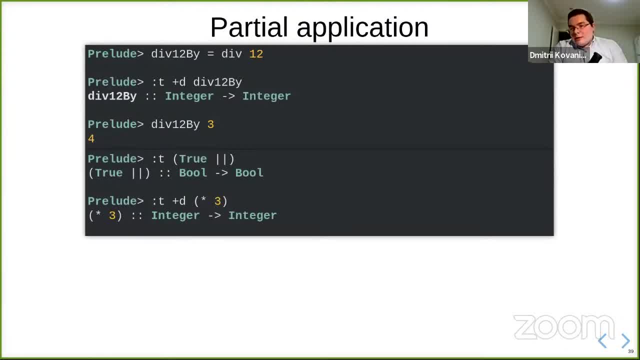 example, multiplication. it doesn't matter where you put it, because three multiplied by something or something multiplied by three, it will do the same, but for some operators it matters and uh, yes, we can use it. let's write another higher order function. this time a function takes an uh function. 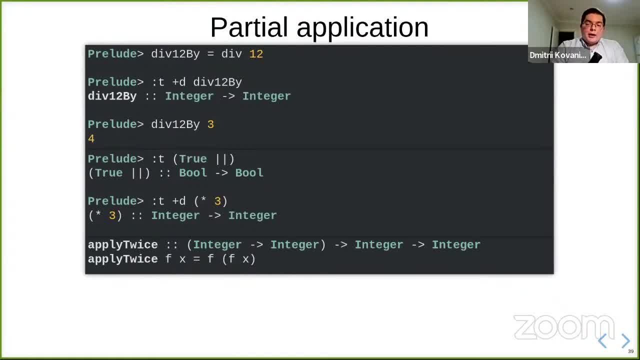 from integer to integer. so it takes one integer, it takes another integer and what it does, it, uh- applies the function to a given integer and then it applies to the result again. so we just want to apply the same function, consequently, uh to it, to the result of the previous call again, just apply twice. 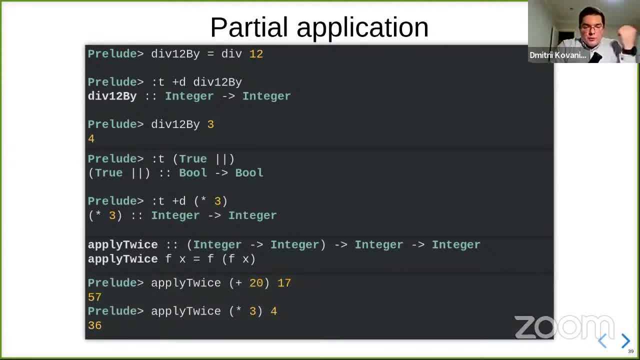 applying the same function twice and if we again we can pass operator, as it's called, like operator section. uh, partially applied operator if you pass this partial function from. so plus, it's a operator or function that takes two integers. we apply it partially to 20 and we now get the function that. 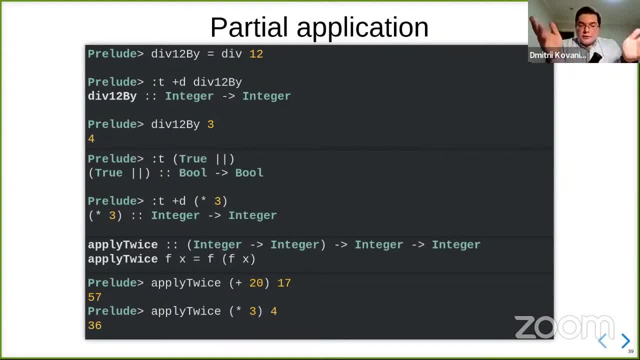 takes a number and adds 20 to it. so now, if we pass this function to and number 17 to apply it, we'll get 57, because we add 20 to 17 once we get 37 and we get another 20 and get 57. the 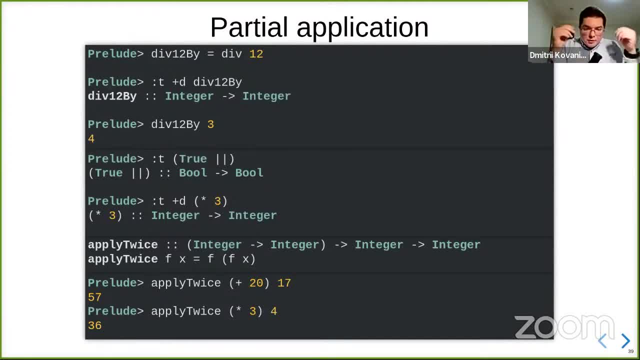 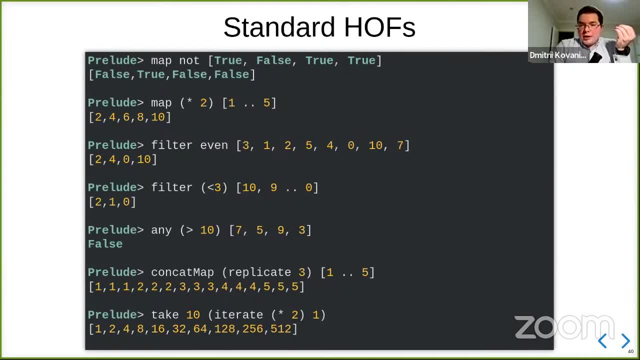 same with multiplication. so this is basically worse um recent working sky underneath and there are some um standard, higher order functions which are very useful. one of them is map. so map takes a function from element to another element, from one element to the other, and it takes a list and it. 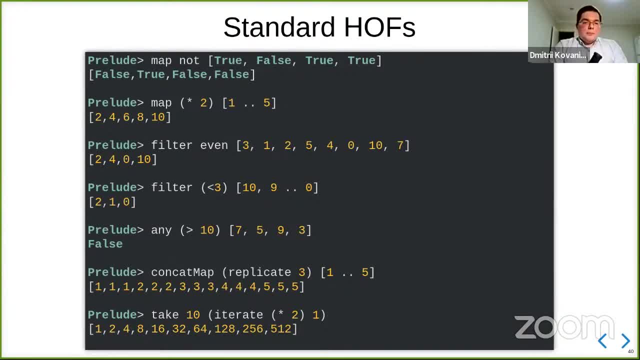 applies the given function to every element of the list. so let's say we map function node over the list of booleans and it will inverse the every element of the list. oh again, if we uh give like operator uh multiplication and apply it partially to two and 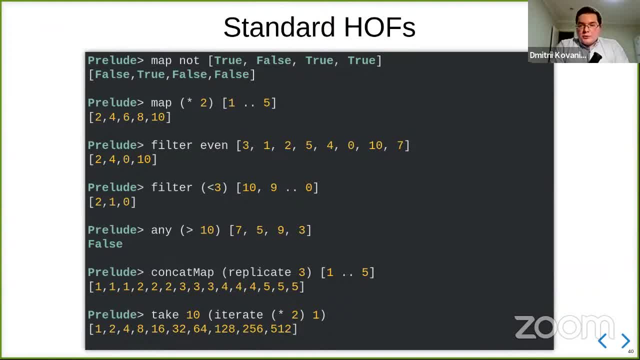 then pass it to map and the list from one to five, we will get list of odd numbers from two to from all, sorry- or even numbers from two to ten. another helpful function is filter. it takes a predicate- remember what's predicate's function. that returns uh, boolean value and list and it keeps all the. 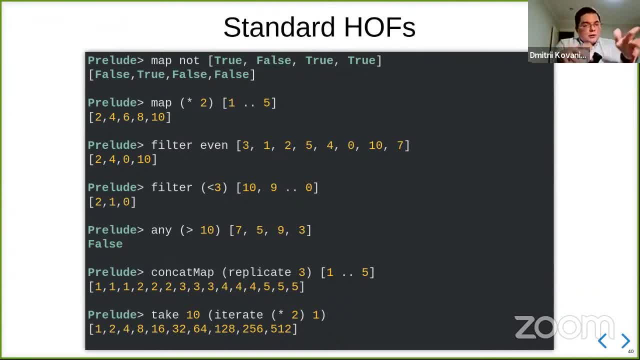 elements where the predicate returns true. so it runs this predicate over all the elements of the list. and if the list and if the element is true, if the predicate is true on this element, we keep it in the result. so this is a example where we want to keep only even elements in the list. 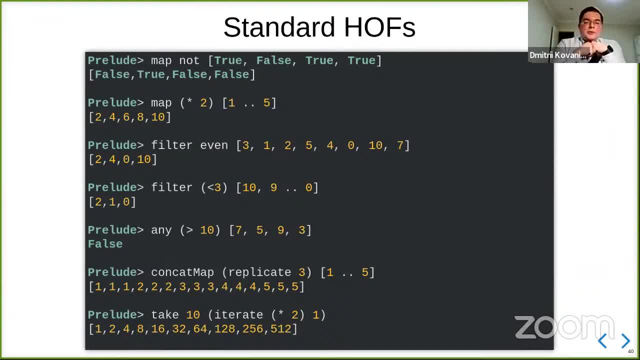 oh, there is this cute heart operator where you want to keep on the elements less than three. um, you can also apply pass operators to filters. another helpful higher order function: any just checks if there's at least one element of the list that satisfies the given function. so and it will first stop, so it won't go for the entire list. 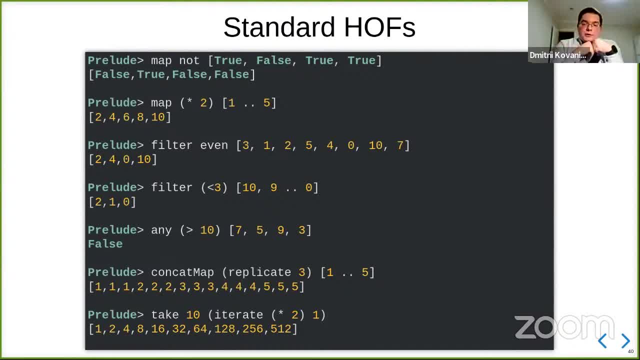 and it can actually work on infinite lists if there is element that satisfies first earlier. so again, everything is lazy. another helpful function is concat map. it takes a list of elements and a function from element to a list. so you have this element, you apply this function, you now have a list of lists. but 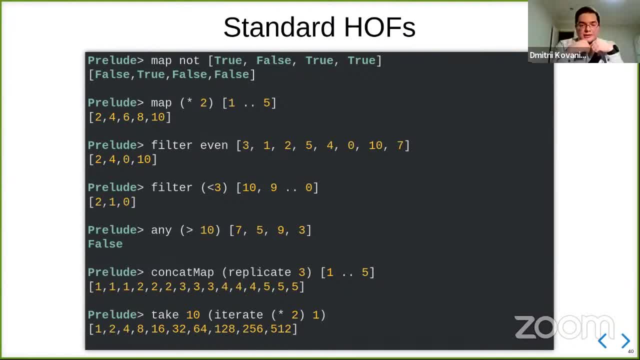 it takes an initial element, it takes a function and it creates an infinite list of applying this function to the initial element is the previous result of the second. so, for example, iterate multiplication by two, one. it gives you a list of all powers of two. so one, two, four, eight and. 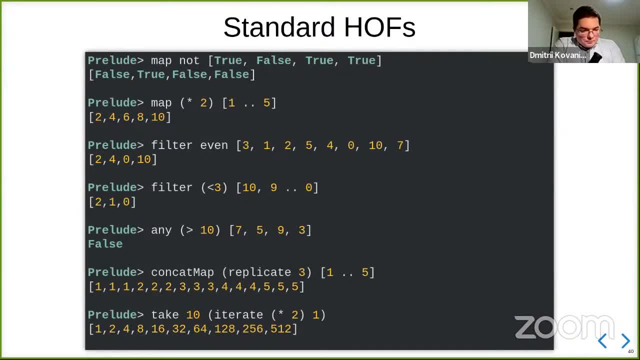 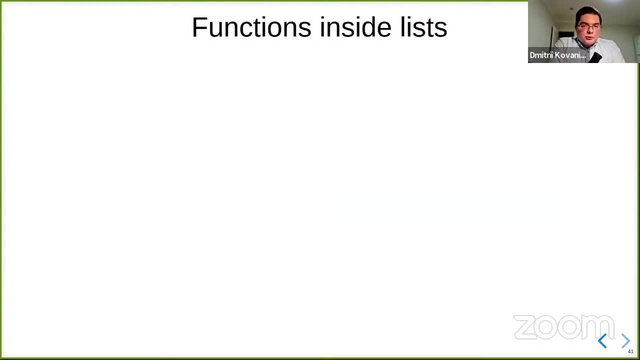 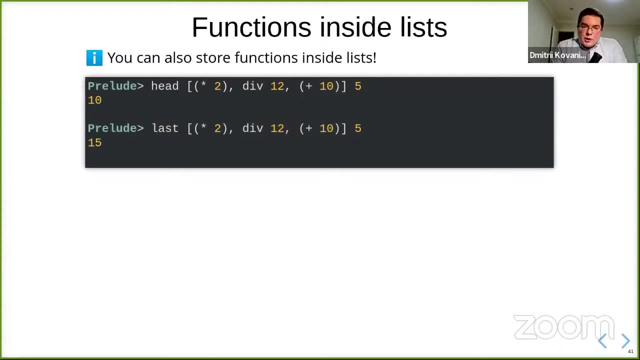 we just get, uh, we use take ten to get first ten powers of two. this is how functions work and again, as I mentioned, functions, uh, first class object and which means that we can actually have them inside containers so we can pass them as arguments to other functions. so why not have them inside lists? so we have a list of functions, again, because why? 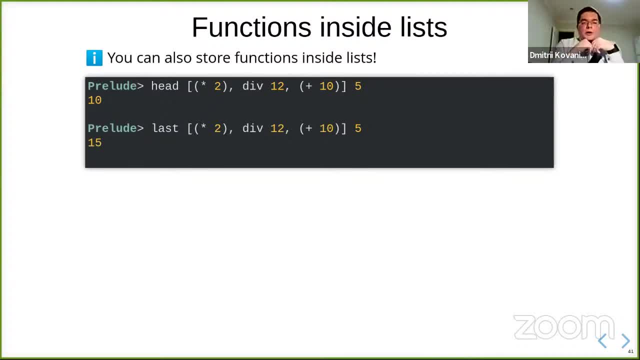 not, and the first functions multiplication by two and we use function head to extract the first element and we apply it to five. so five multiplied by two is ten. again, no special syntax, function is just a space. so we apply, we get a head to list and then get a function and we apply it to five. 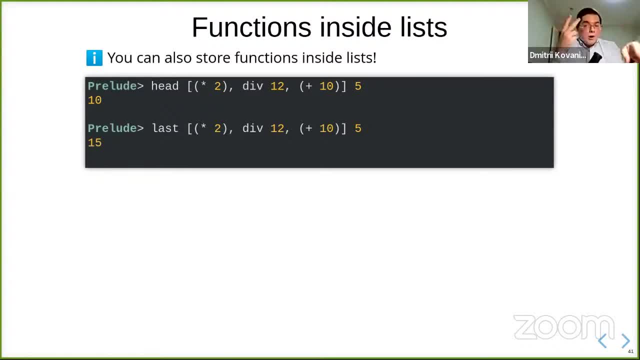 so it may look like function head takes two arguments, but actually it takes one argument, but it returns a function and we just immediately apply it to five. so yeah, I kind of see that it might be a little bit difficult to understand and kind of strange, but this is what is happening. so 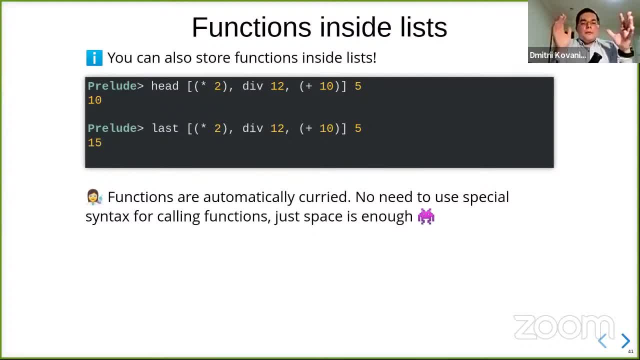 if you want to take one thing from this lecture, what's important to remember is that everything is a function. so, uh, operators, uh, functions, uh. applying function to something is a function. partially applying, so lambda function of functions. a function is a function, obviously, uh. and the function application is also function, just a. 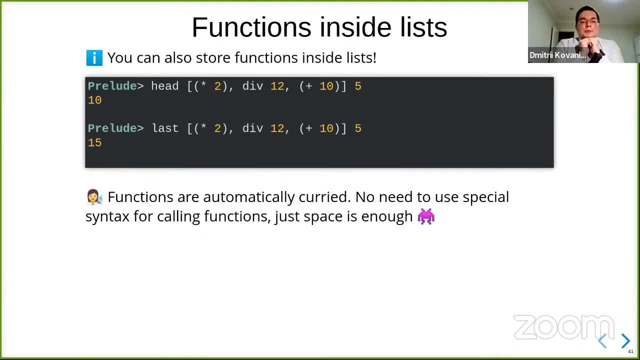 focus of functional programming is on function, and this is how it helps you to, oh like, compose things, and which is great is that the syntax is actually the same, so you don't need to have special syntax. you just don't. okay, I just put the function, just put space and argument. 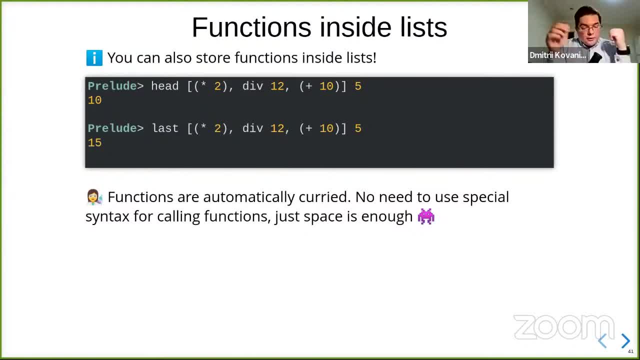 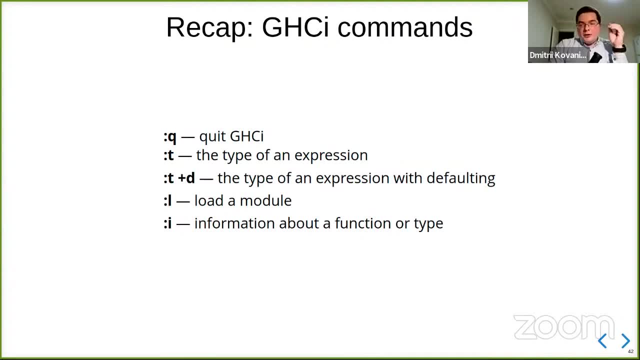 and I apply it and here you go, so everything just works out of the box. so finally, just to recap of jc commands, the most important is actually colon Q is when you're finished playing with jc, you can actually quit it by typing colon Q. and uh, I haven't mentioned colon I command, which is short. 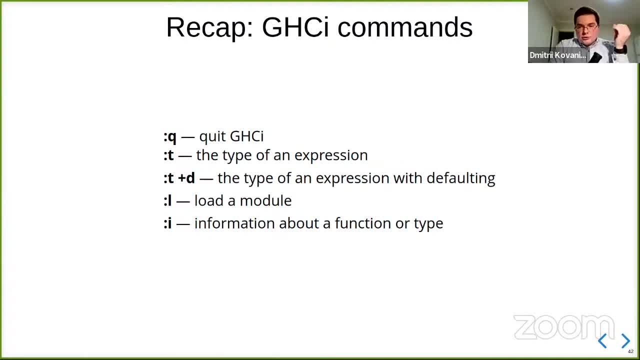 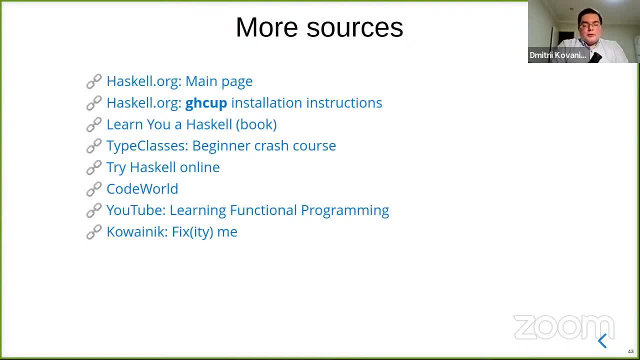 for info. information if you want to inspect something about functions or operators, you can use it, and this is a list of resources that you might want to read if you want to dive into some topics or if you're struggling with some of the home exercises and uh, that's all. thank you for coming. 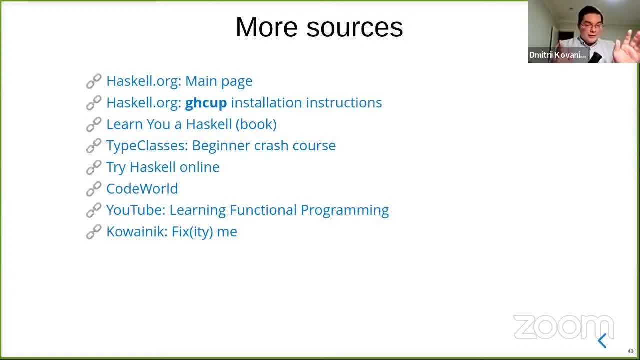 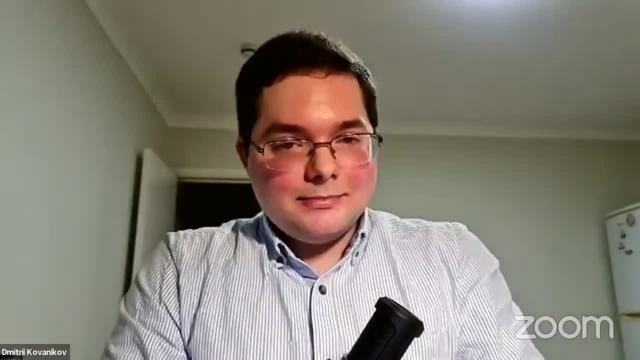 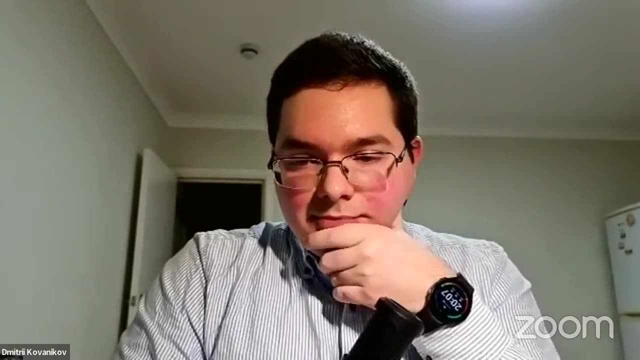 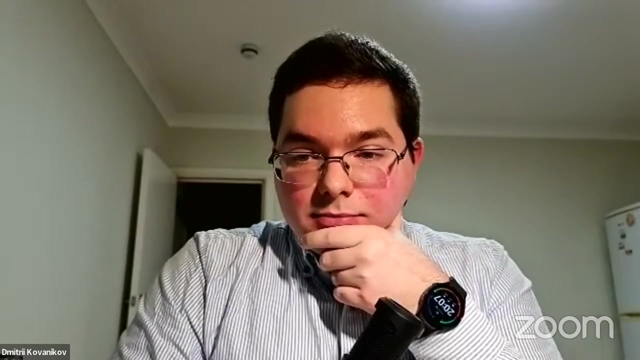 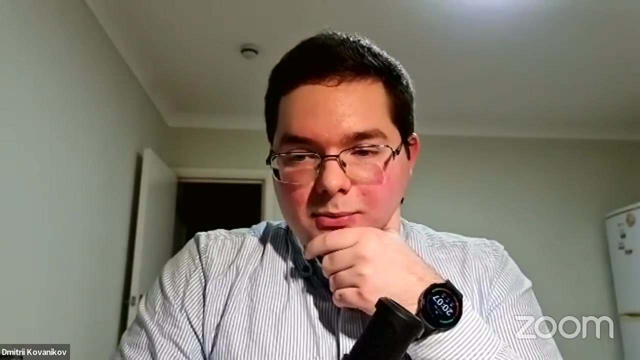 to the first lecture and, uh, now I'll get, I will. I will answer all questions, whew. so I see that the chat was quite alive, which is great, because actually can't see the chat while I'm presenting and I wasn't even sure that you could. 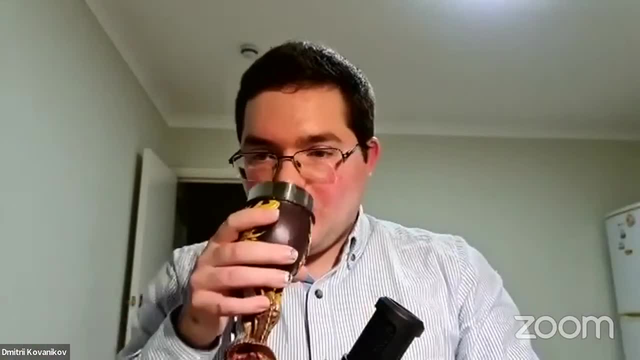 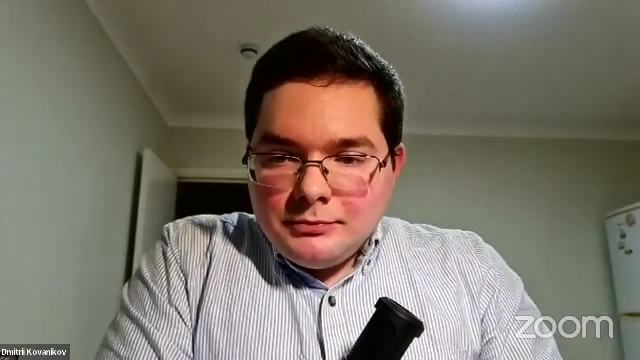 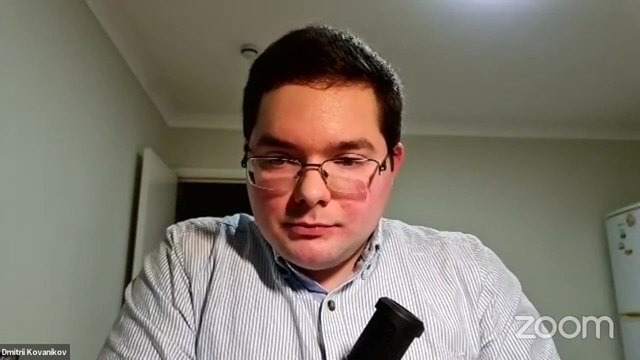 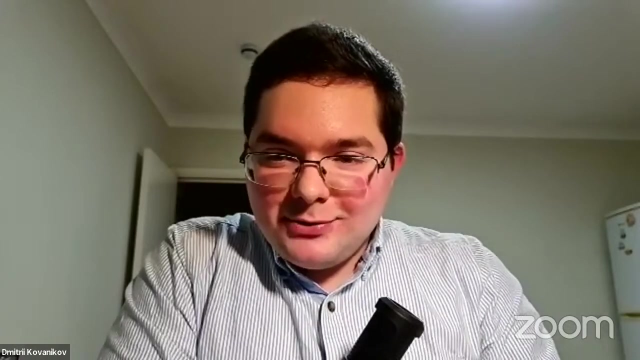 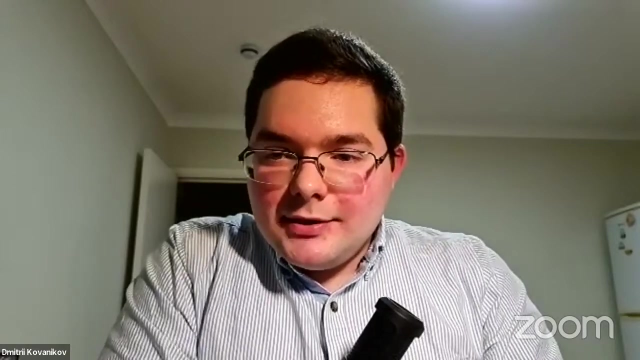 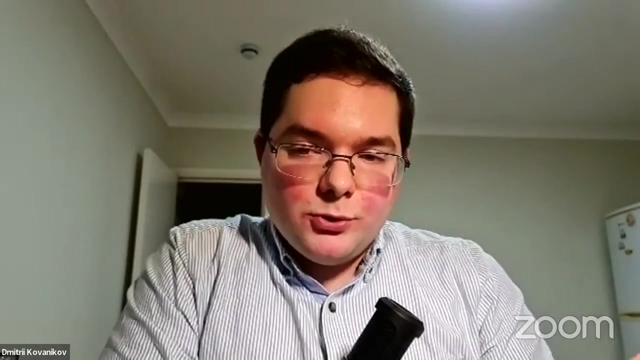 see me, foreign, foreign. all good functions are four letters long folder. well, maybe it's not a good function then? can the elements in the list be of the different types? uh, no, all elements in the list must be of the same time, so you cannot have like true and the number. 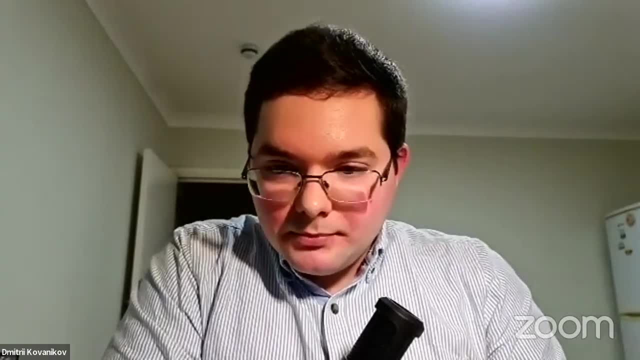 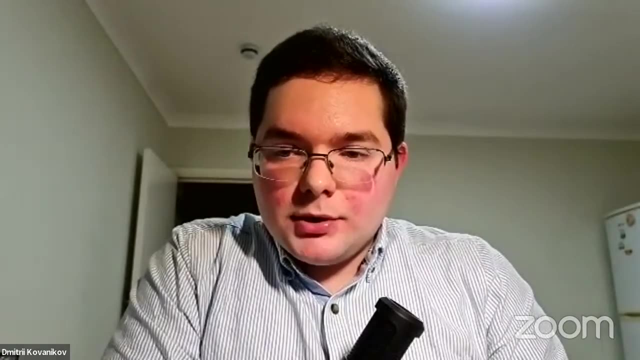 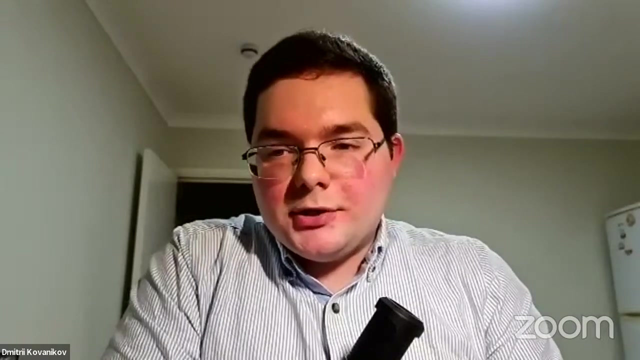 there pattern. um, here we can see. uh, this is actually. um, I can just use this. this is a positive thing. one letter, THINhoo, uses the long produce button, but this is a positive thing. all elements must have better to use. take one than double exclamation marks. well, um, 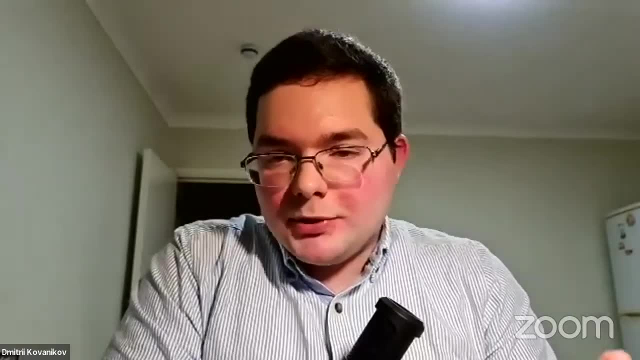 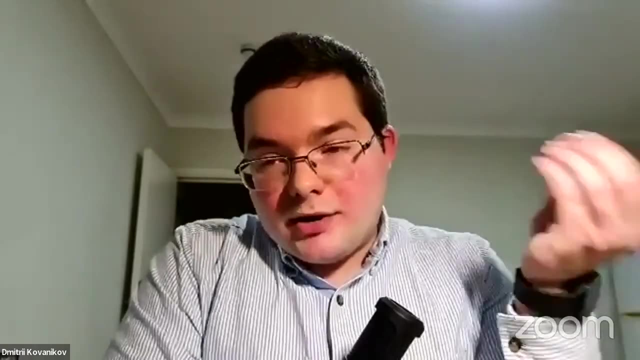 the types of are different. so take returns your list. so if you take one of this, you will get the list it also. essentially it will contain only one N, but still the list. the exclamation marks that вже extract this element from this, so you need to do again head or. 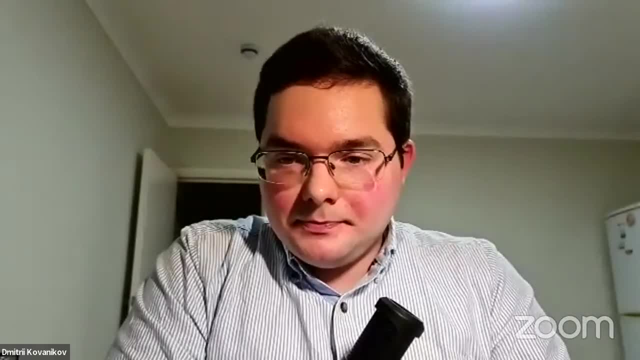 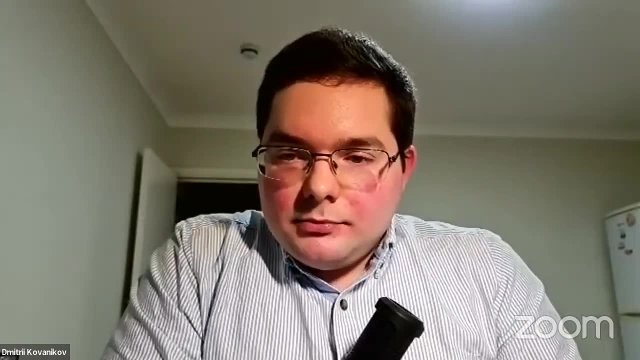 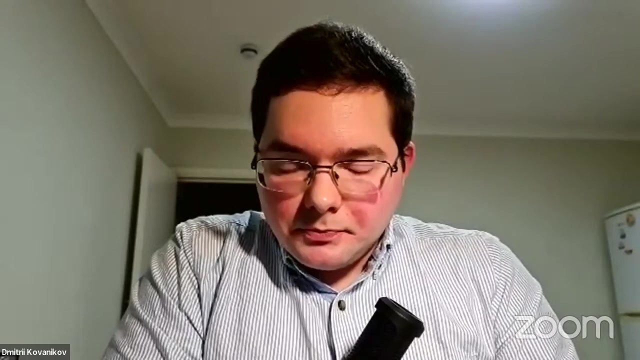 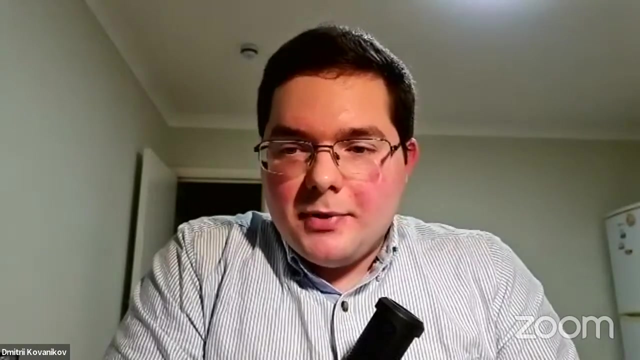 something else again: exclamation, double exclamation, mark zero, wise lens, computed every single time because casco has a time for this, was kind of information cached when you do it once and the list and doesn't change. well, because it's how lists are implemented. so, to give some like more algorithmic, brown background lists are linked. 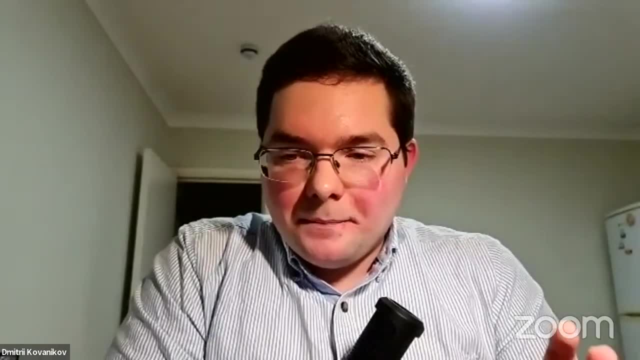 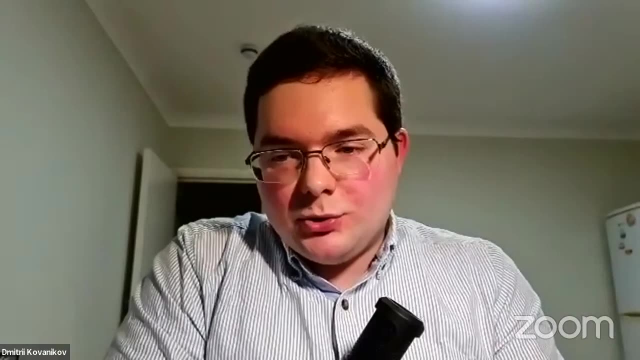 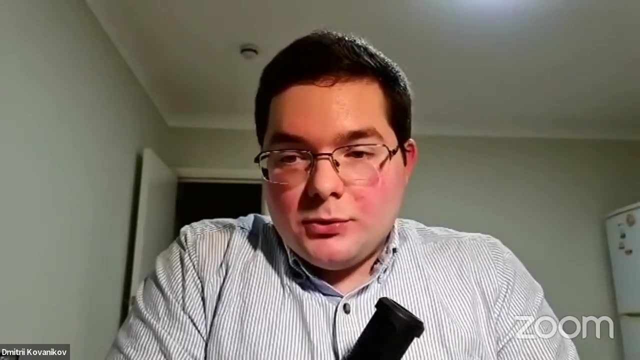 lists so they don't uh uh store, uh like the lens inside and with that, to calculate the length of link, listen, you need to walk through every element of the list and just increase the lines by one again. if you want to have the multiple times the same list, you can just use a let in or where, and 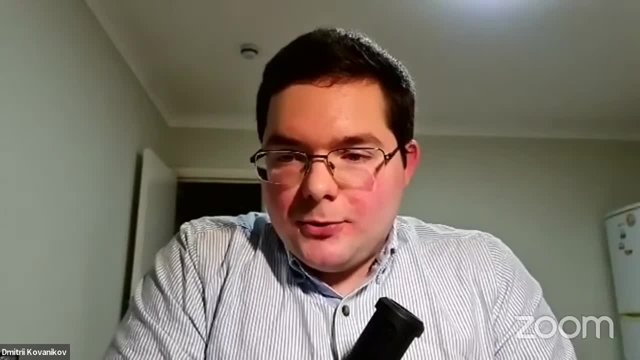 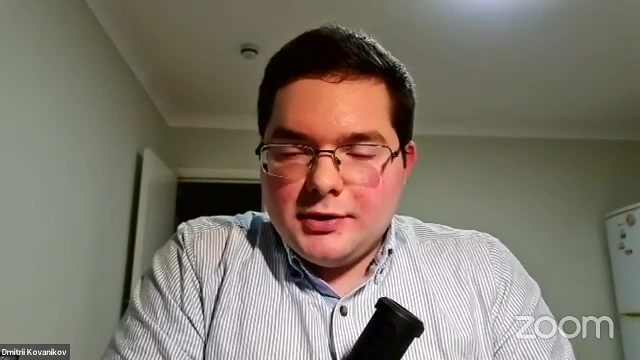 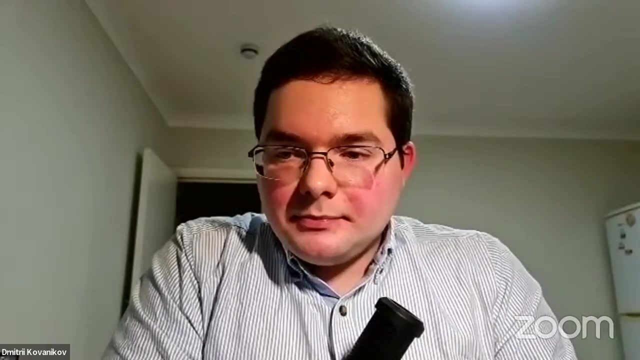 just complete it once and then reuse the same variable, but you still need to go through the dialest. is it possible to get element on infinite index then? no, because you need to construct an infinite index first. good luck with that. if you have an infinite list, how could i get the last element of it? well, if you try. 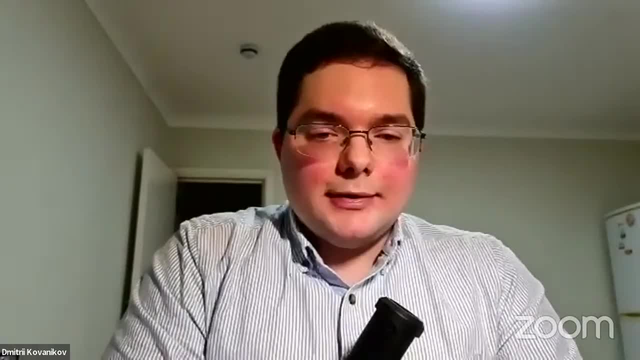 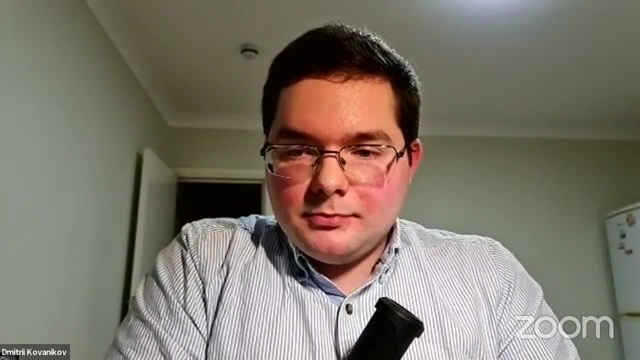 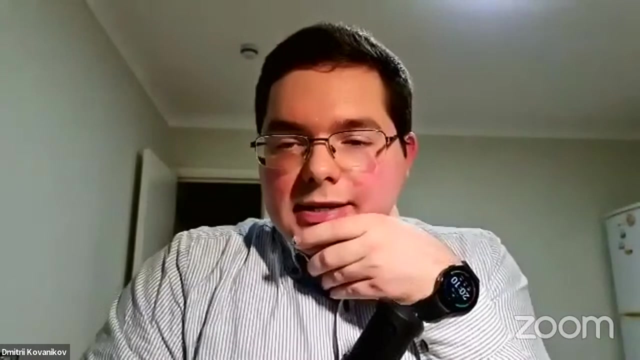 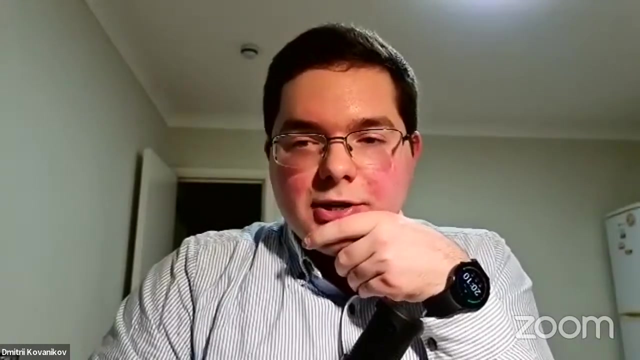 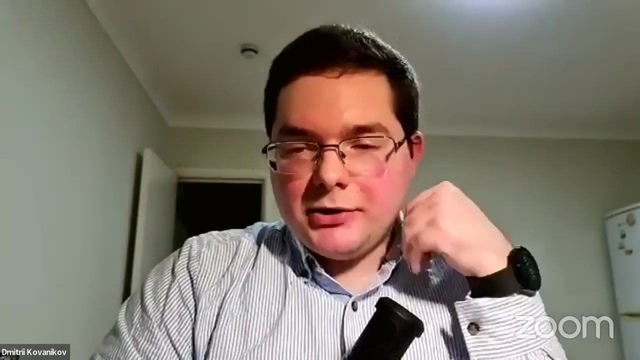 the function last will just hem, so it's not uh possible to do so. yeah, see some replies around this. sorry, i'm just browsing through the chat open to answer people questions. if you, um, maybe have some notes on some slides, feel free to ask questions. now there is as: 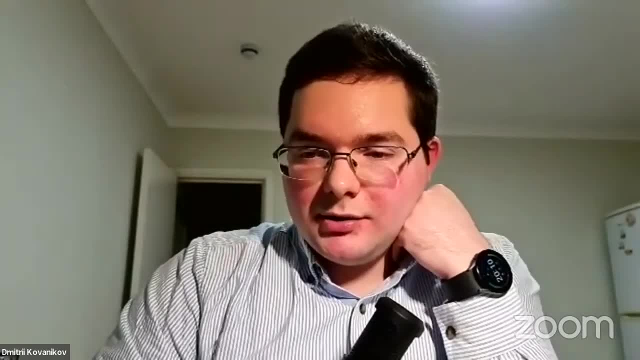 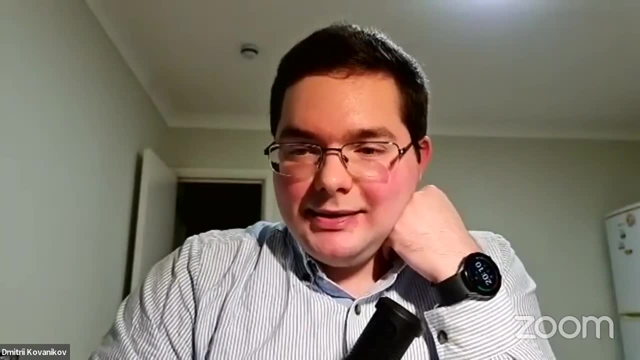 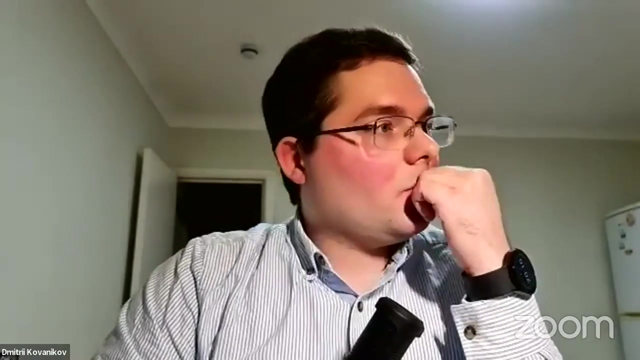 i mentioned previously, there is delay 20 seconds between what i'm saying and the uh when you're hearing it, so it might be better to ask questions earlier. will slides be available to download after the stream? well, slides are already available online, so you can download the html, i guess, on this platform. 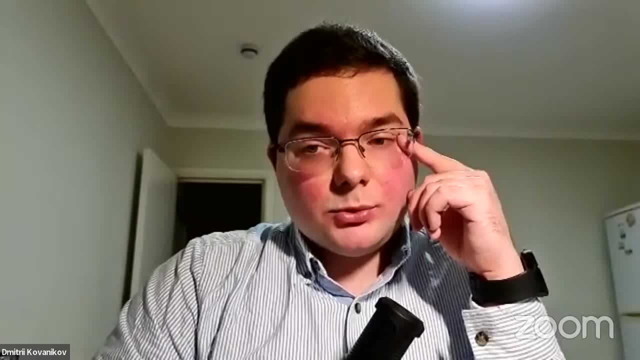 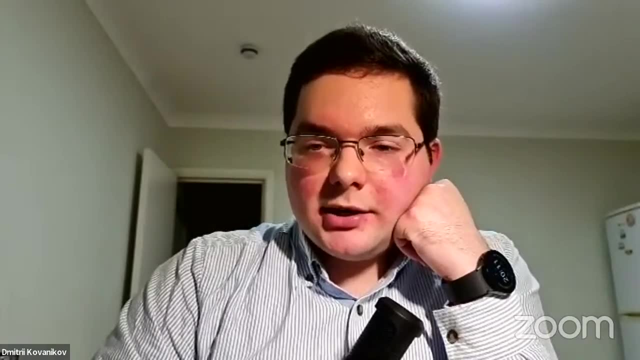 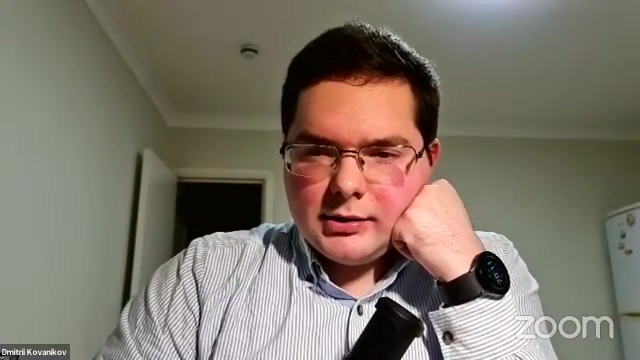 slides, you need kind of to pay to export them as pdf. so if people want pdf, well, maybe interested people can cash in and i will be able to download slides pdf. but html you can get from now. it, i think it's uh, it can be used offline, so it's not really that. difficult, but i haven't checked. what's the difference between int and integer? okay, so, um, integer is actually an unbounded integer type, so it can be arbitrarily long. so if you want to calculate two in power, 100, 1 000, 1 million, 1. 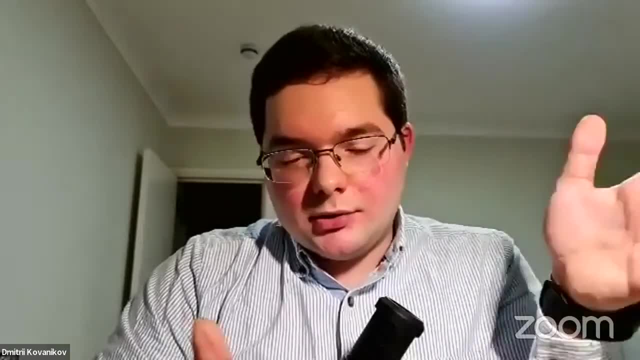 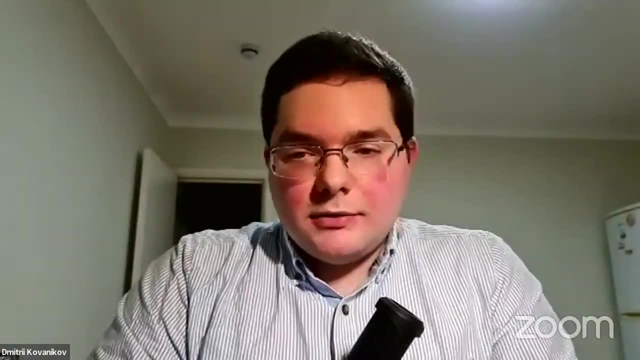 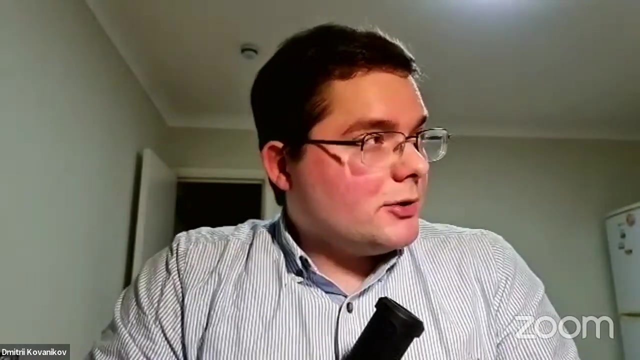 gazillion. it will fit into integer because integer just expands all the memory as long as you want. so because of that it's like less efficient but it fits all dumps. int is a complex, it's between, it's like a machine word how it works in principle. between two, between minus two in uh power 63 up to. 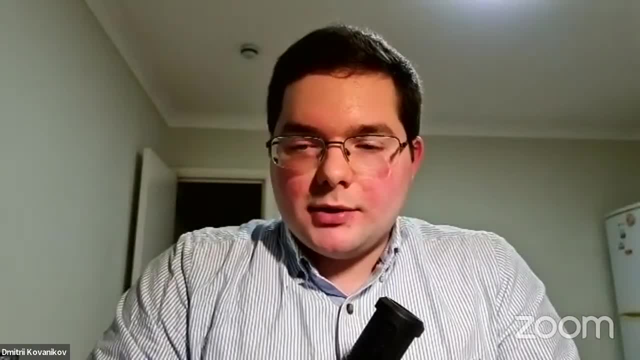 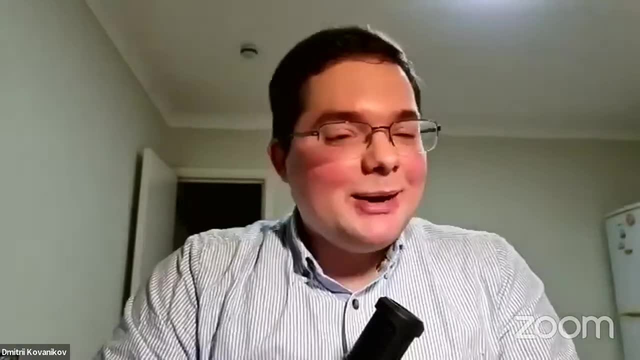 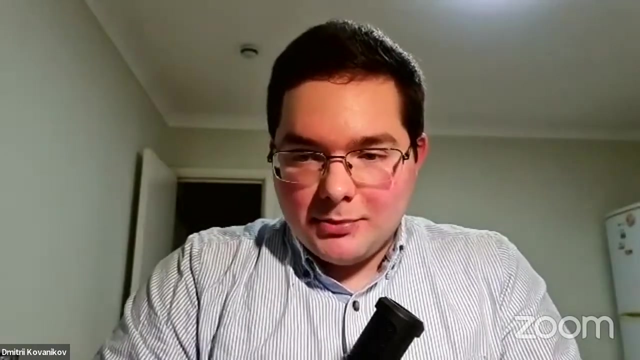 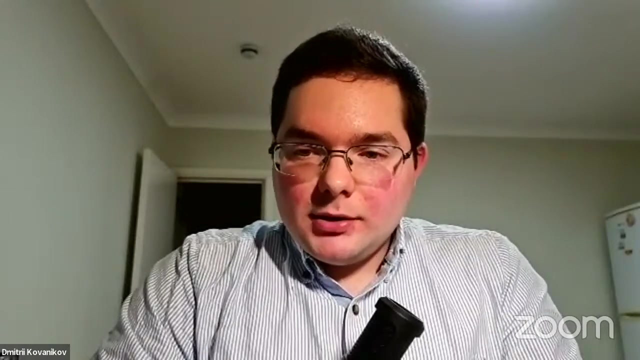 up to um two power 63 minus one. so yeah, the haskell documentation says about something, this power 29, which is really weird. so way, way ahead from something standard, but for now just 64 bit number. the standard int number guard is like pattern matching well. 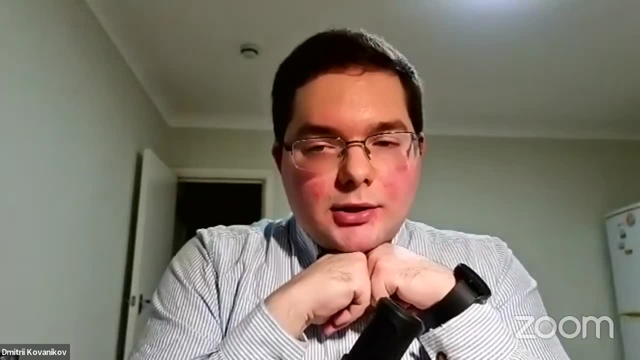 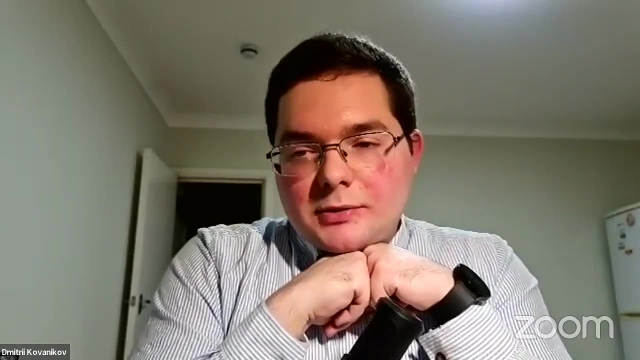 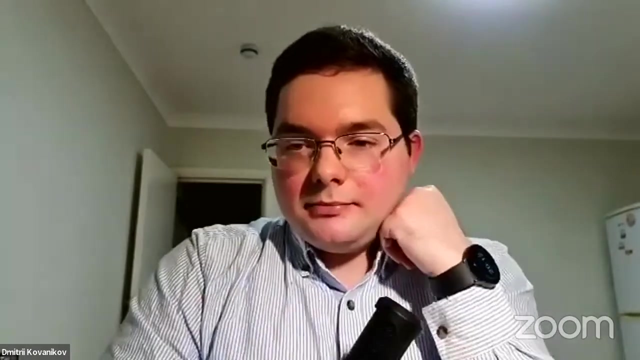 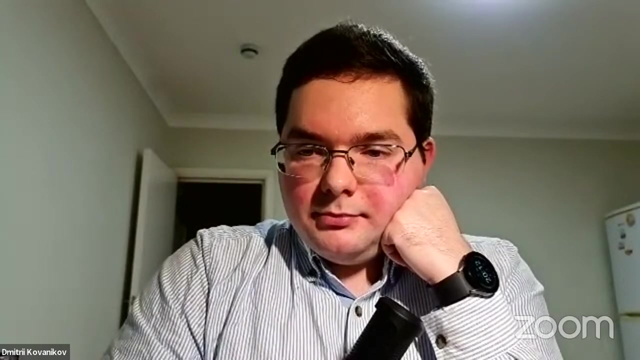 not really, but i mean it just. you can think of the syntax, sugar phone, nested ifs, if the analysis, so you just write, you can think of this pattern like kind of checking boolean values, like a special case of patterns and water matching, but not really is otherwise a keyword. no, it's actually not, it's just a. 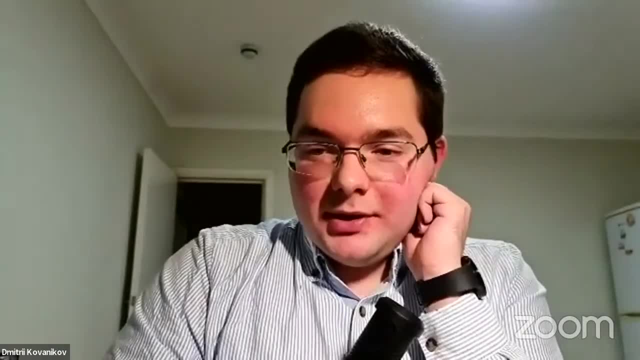 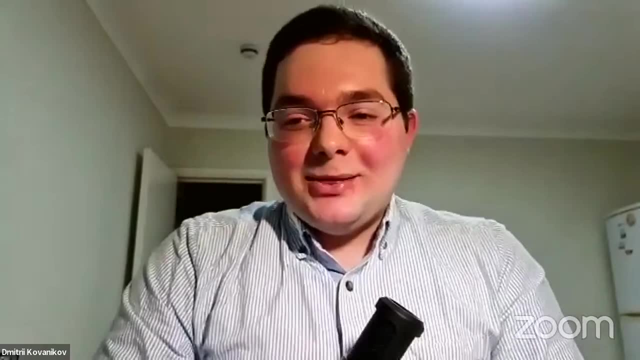 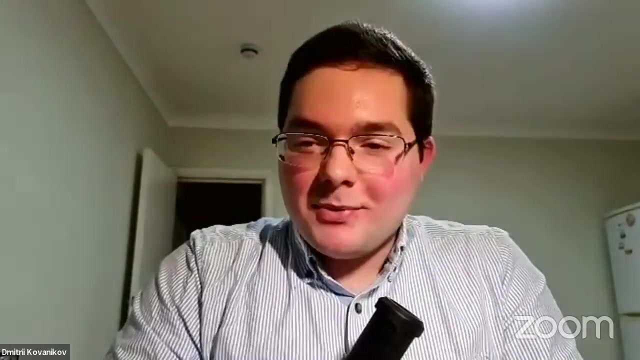 a global variable in prelude and it's all and it's defined as true. so just a top level variable story. so it looks like a keyword and when people find out, i didn't want to tell that it's a standard function. so just don't, uh, uh, prevent people from having this joy of one year after learning haskell. 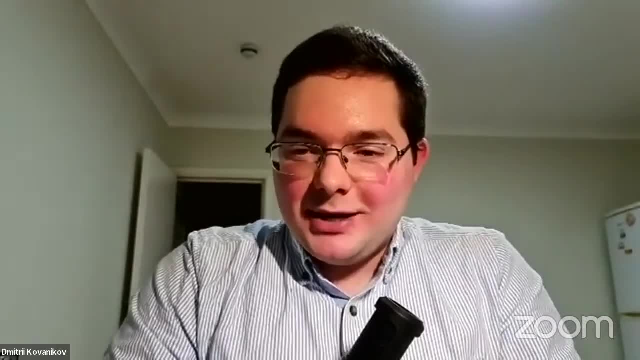 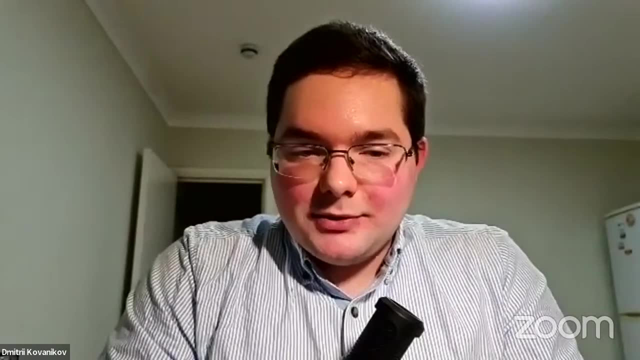 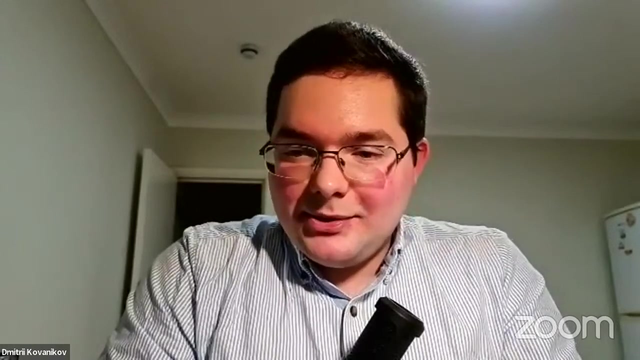 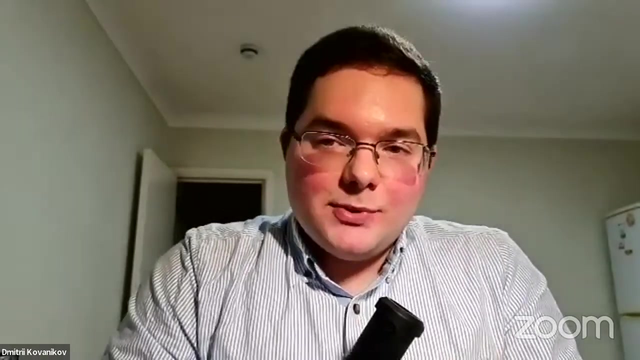 finally realizing that otherwise is just, uh, just an ordinary value. um, so i guess that's all i wanted to say. so, um, thank you for watching, uh, i will see you next time. bye, thank you all. thank you all for kind words. um, don't worry, the recording will be available later. so if you skip something, if you want to, 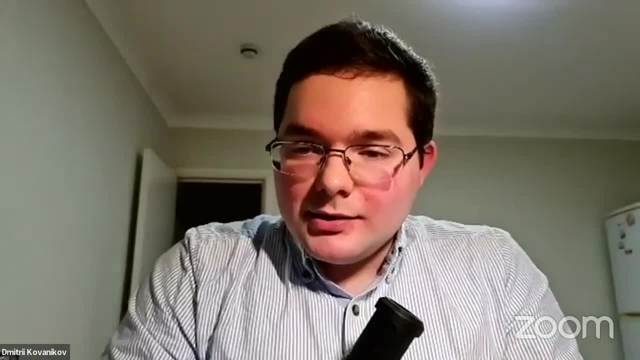 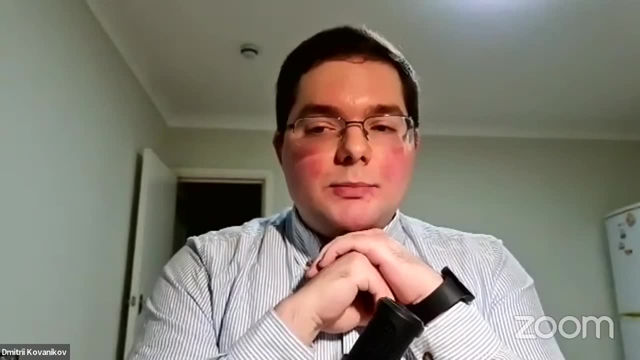 re-watch. um, you can watch it later as many times as you want. so i see some questions. uh, more Where else? Yes, as I mentioned at the beginning, Haskell is a layout-sensitive language, so it's better to keep the intonation on somewhere else. 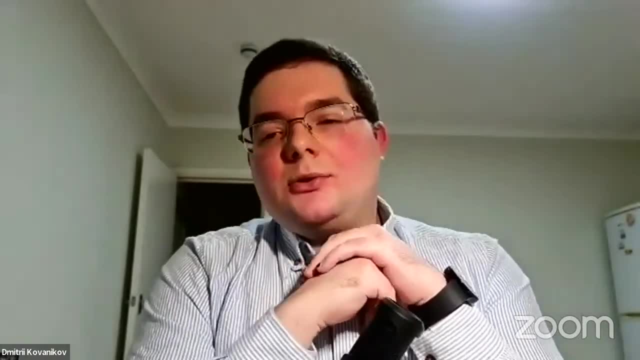 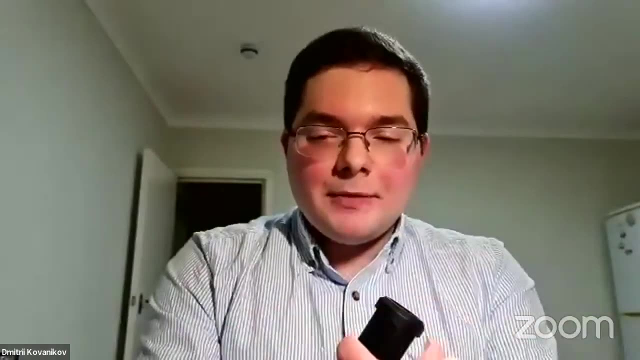 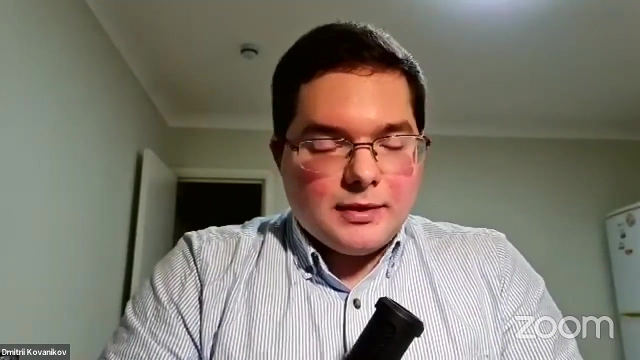 So sometimes rules can be really tricky to get. some things don't work. And also you cannot use the tab character, so tabs are illegal. you need to use exactly spaces. So if you use tabs you might get weird results. Just use spaces, and the suggestion for now is just a copy-code from the slides. 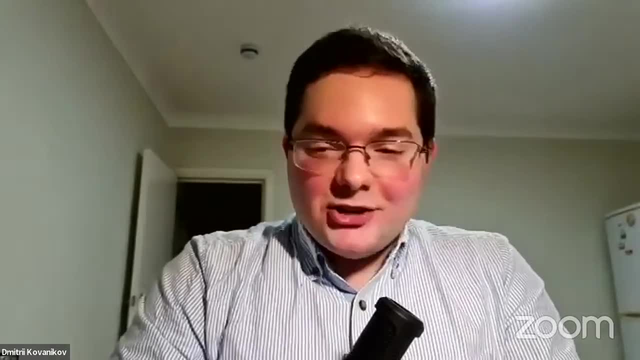 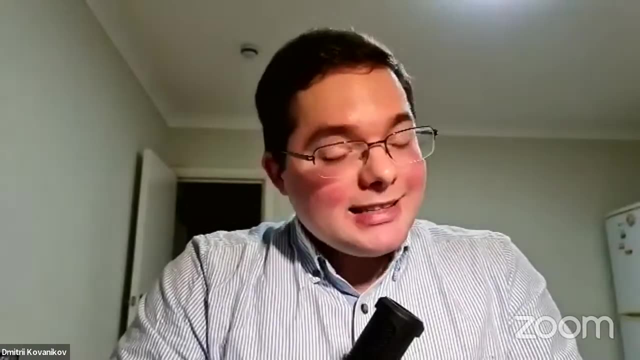 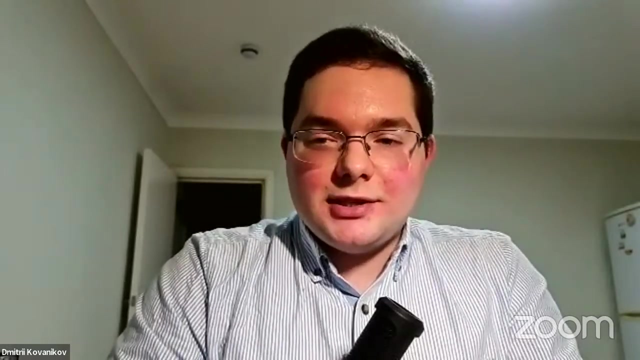 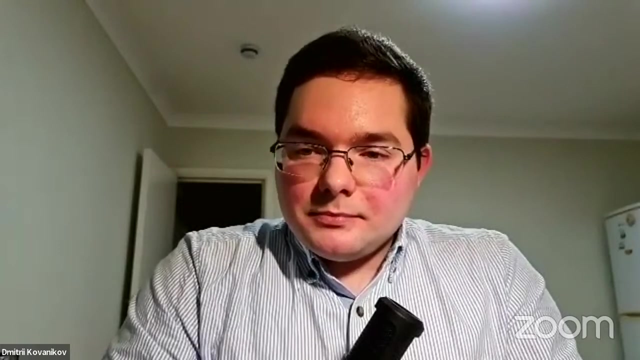 It's verified that it works and just change the relevant parts when you need for now. Later you get kind of intuition, but sometimes syntax doesn't make sense, So you can try to torture Haskell compiler and play with different syntaxes. and well, you don't want to see this. 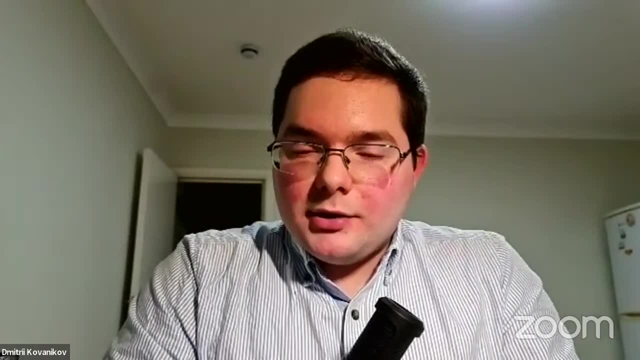 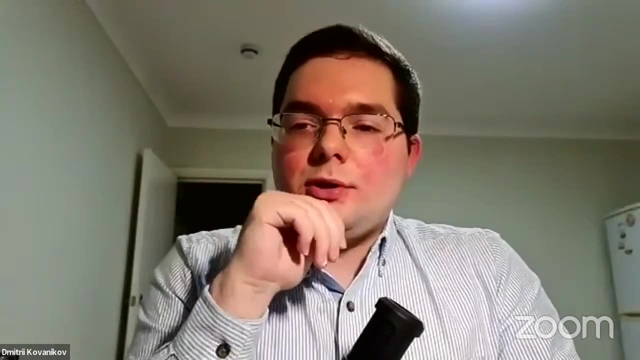 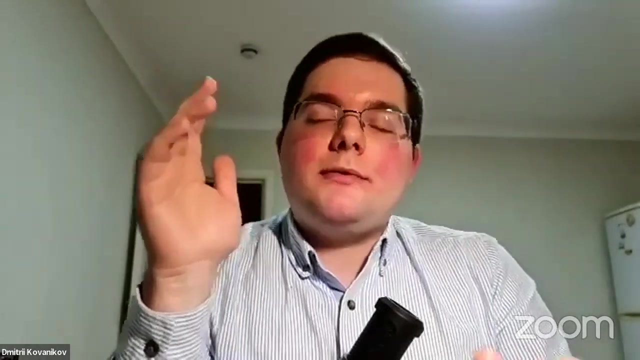 What is the best? What is the best or any solution for spaces? Space leaks, cause of laziness? Well, best solution is to write good code, But there are some standard practices which can help you to prevent having space leaks. So I usually I mean, yeah, laziness, I mentioned the benefits of laziness. 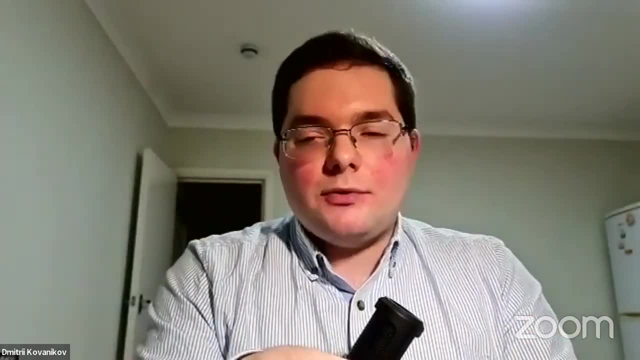 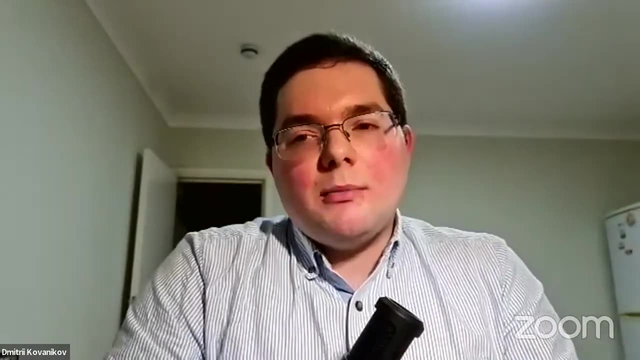 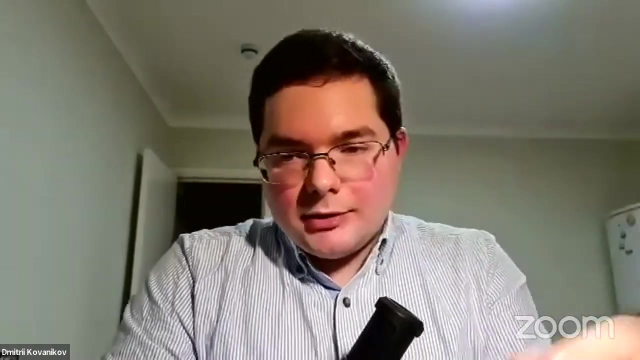 that you don't need to like evaluate something you don't need. But the problem with this is that sometimes it can be you can have an obvious space leaks when program consumes more more memory than it actually needs because of laziness, And there are some standard patterns which you can use to avoid it. 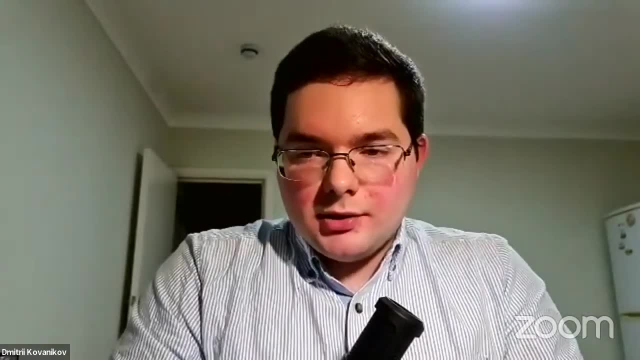 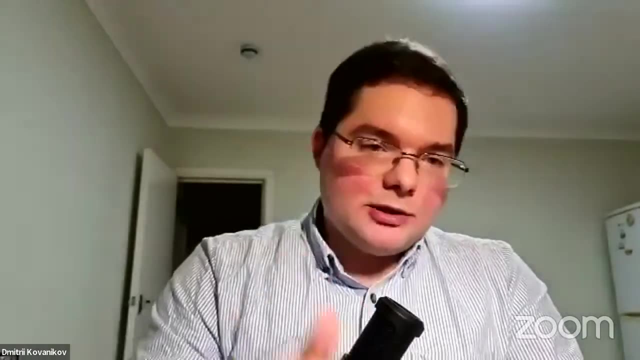 They cover like 95% of the cases and the rest There are tools to investigate specific, So you can just monitor performance of your program. You see that this memory consumption grows, grows, grows and bigger and bigger. And you there are ways to see why it's happening. 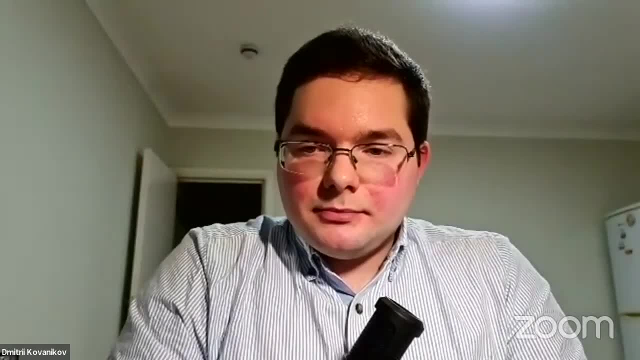 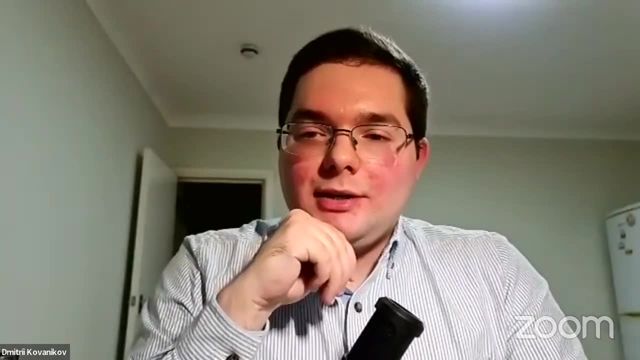 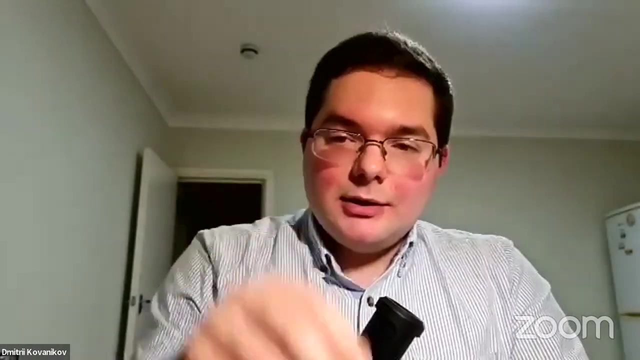 Well, not always easy, but sometimes Folder roasting is something I didn't expect from this lecture. Well, we'll get more into folder on the third lecture, where we'll expand folds and other stuff. Well, just the not always neat and it's not always used when it's actually. 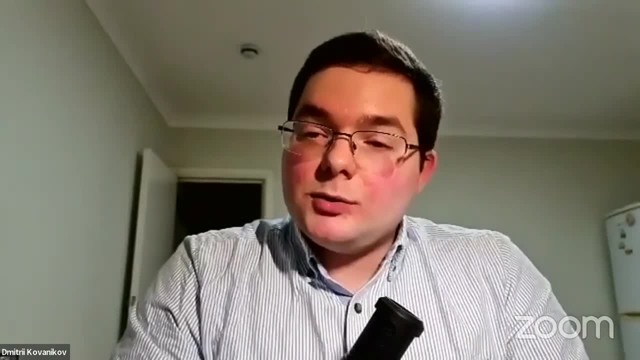 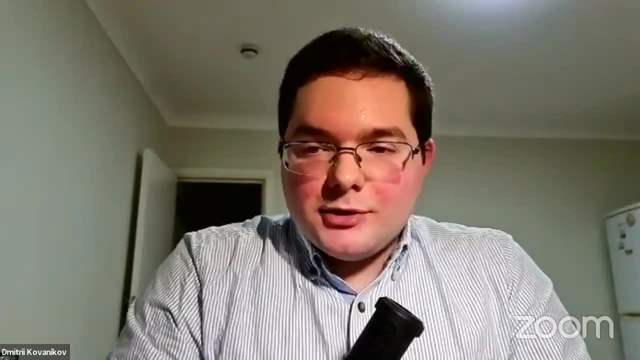 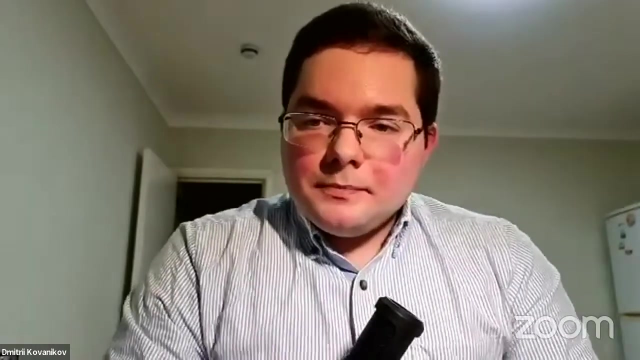 because, again, because of space leaks, sometimes it's used with something else would be better. And also, sometimes, again, it's maybe better to write explicitly recursion rather than using folding function. Well, understand that folding is great, But you don't necessarily need to use it. In other languages, there is usually a limit to recursion depth. What about Haskell? Well, the limit is the sky, as in favorite content movement. So, as long as you have memory, there is no limit, And so, yeah, if it fits on the question stack, it's good to go. 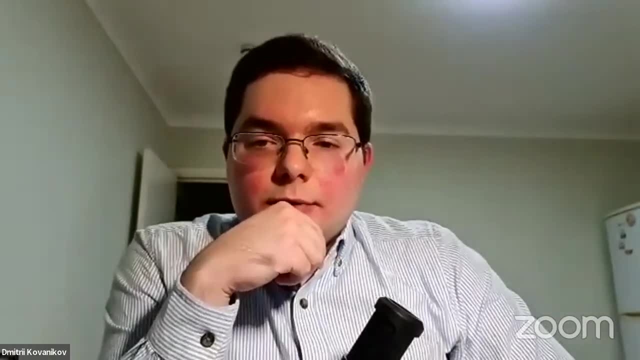 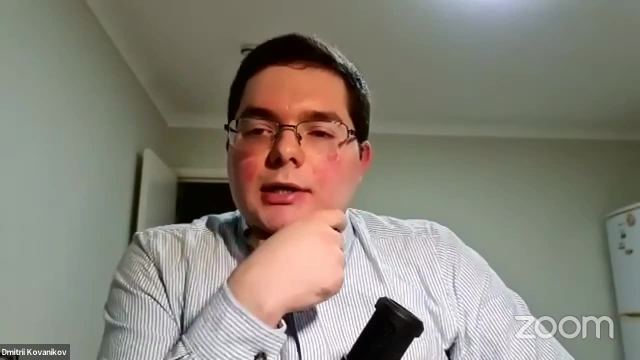 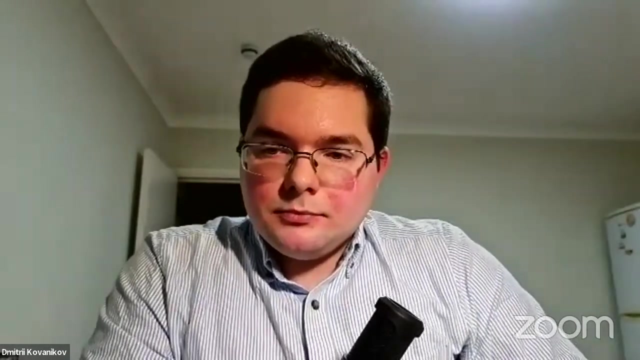 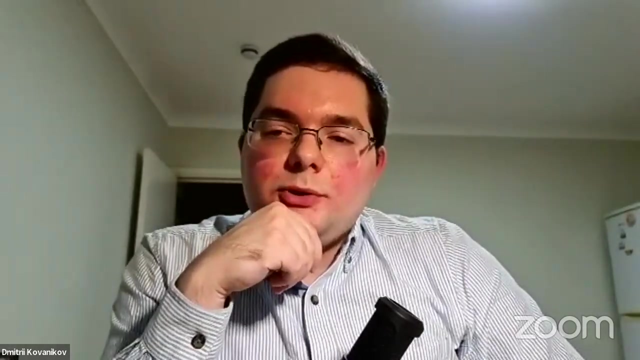 I missed why it just number F o one is treated like int to int function. Sorry, I didn't quite get the question. Maybe you can elaborate and repeat in more details. But for me type hello will return hello, colon, colon string JCI version nine, point two, point one: 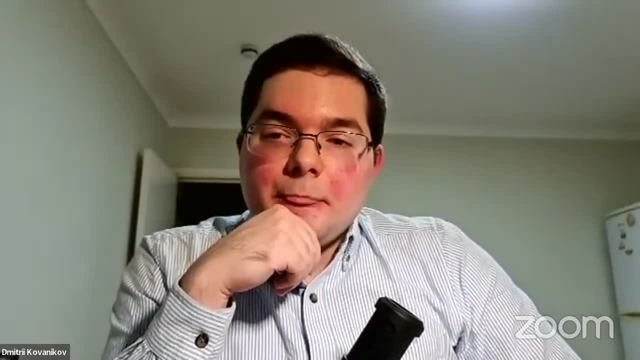 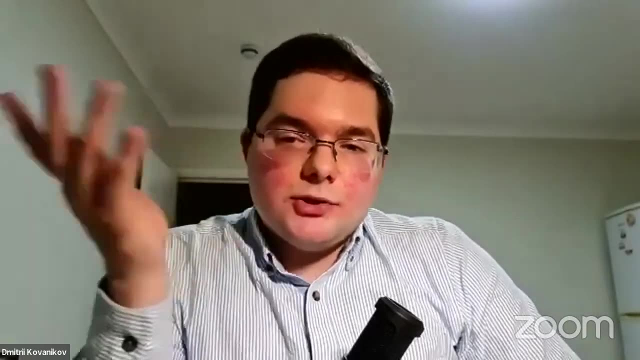 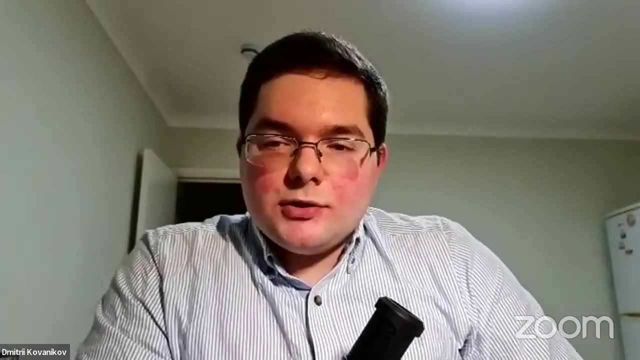 Okay, oh, great that it's finally fixed. uh, we will see why it's string on the second lecture. but string is just a list of characters, so different name for the same thing. potato, potato. what is the preferred type? it's just four spaces. well, if you ask me, i prefer four spaces. 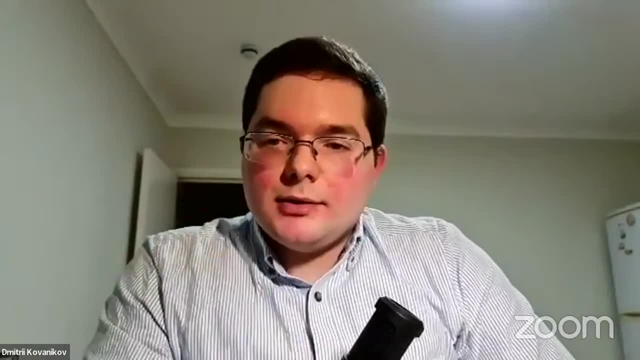 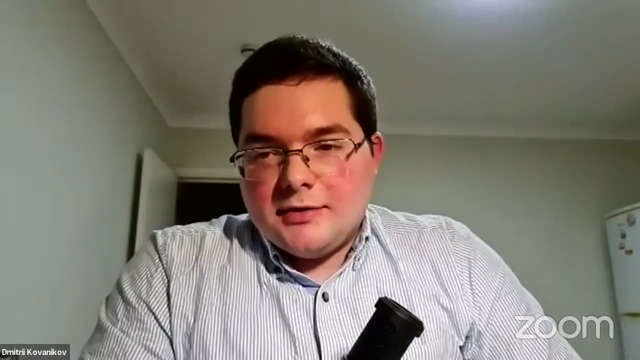 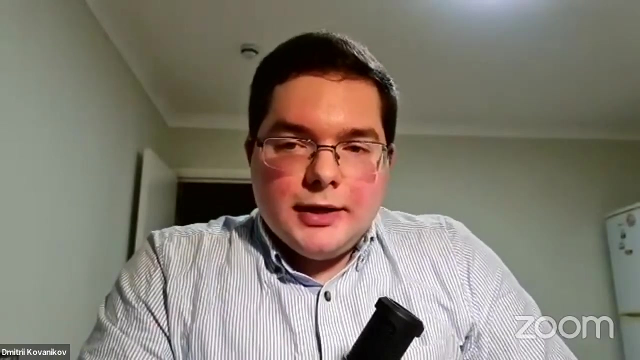 but there is no like accepted worldwide uh haskell style guide. so some people use two spaces, some people use four, some people use three because they decided it's impossible to agree on two or four. so just to make everyone unhappy, they use three. uh, so yeah, you can use whatever you like. 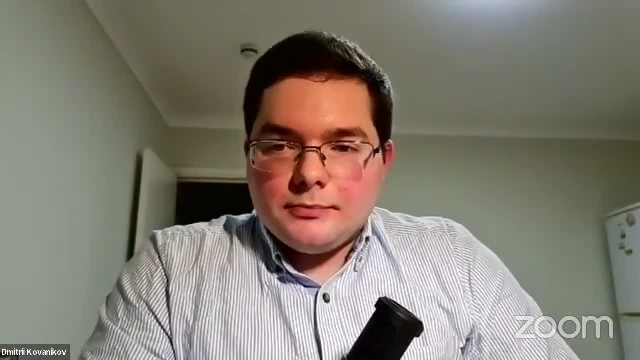 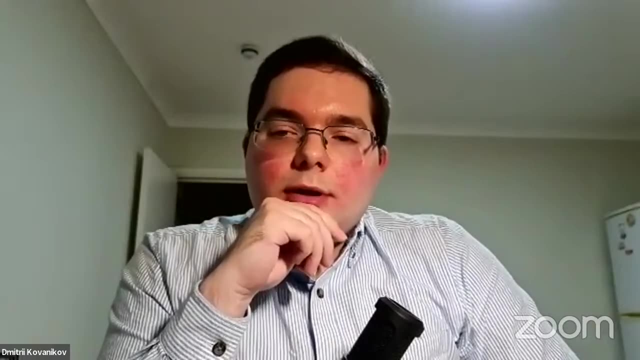 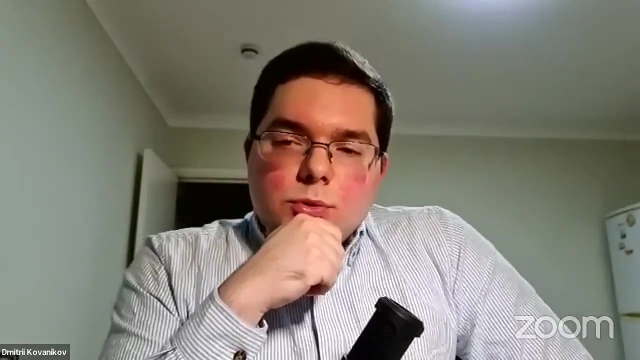 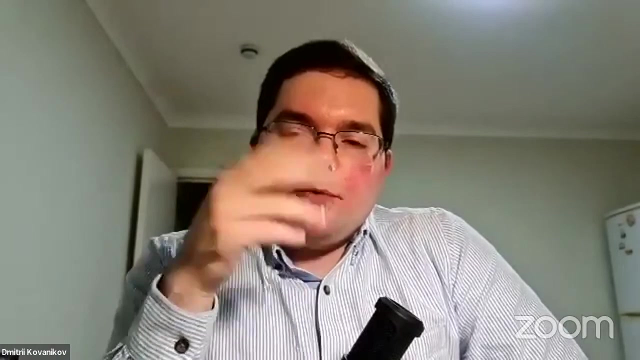 i will check your solutions anyway, i just prefer four. the order of the arguments is unfamiliar to me. are there any reasons for this? can you elaborate more about the order of arguments? so what does it mean? reasons for what the type signature you write just types well first. 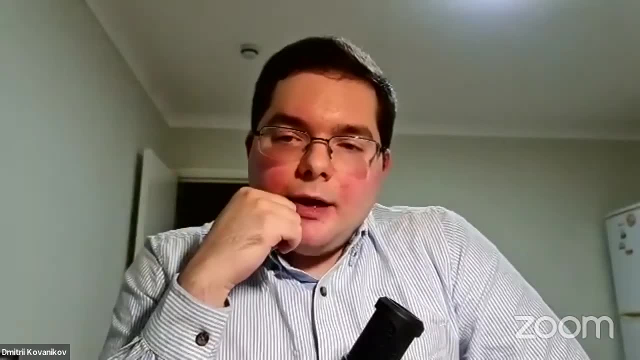 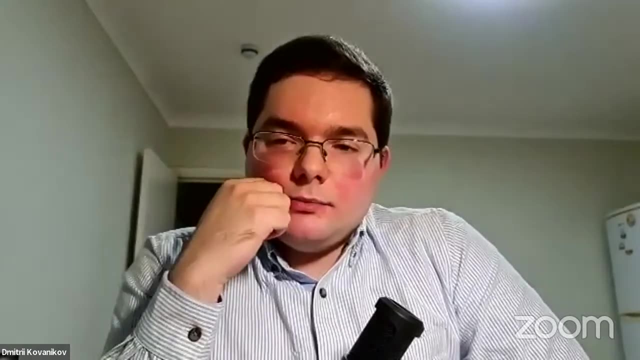 type is an int and the second type is a list. and then the arguments are in the same order. so the first type is the first variable will have the entire, will name. the second uh type is list and the second variable will have type list. so with this order of arguments, 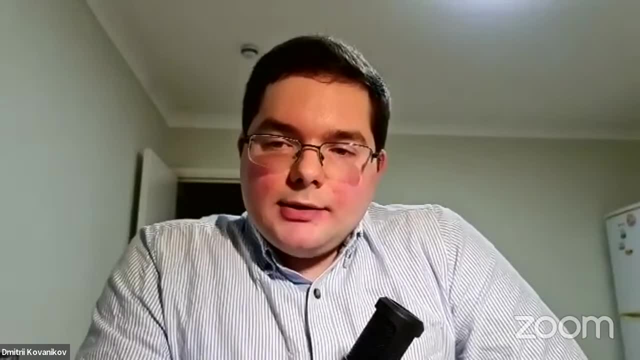 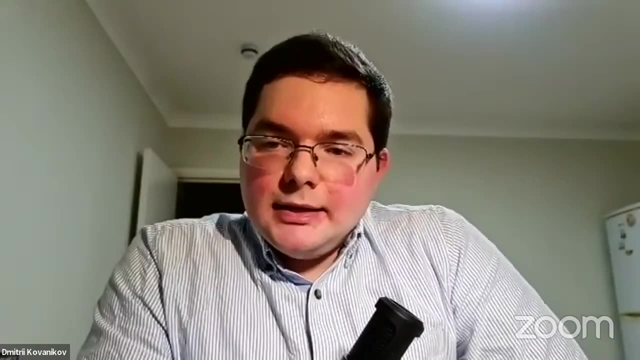 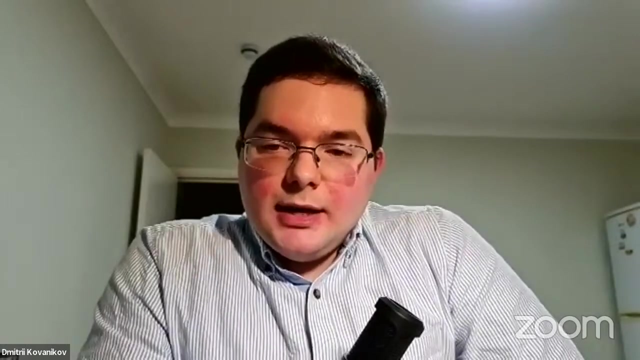 what does it mean? is it necessary to learn some of the mass like lambda calculus or category theory, successfully programming haskell? no, it is not necessary. i can't reach. learn your haskell book from slides url. yes, this is actually a problem. learn for haskell. 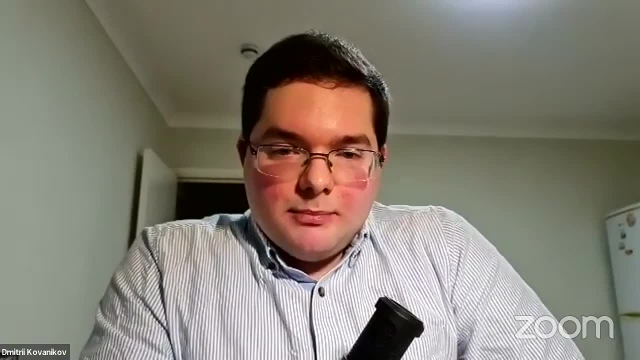 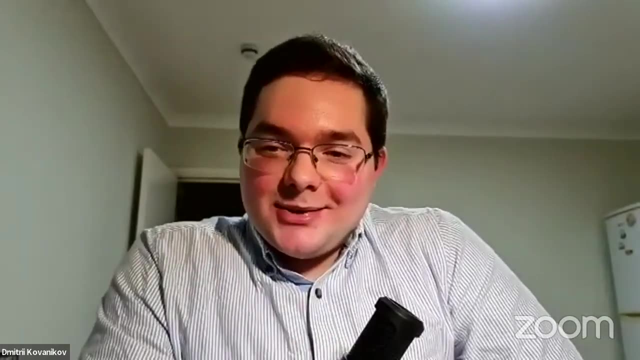 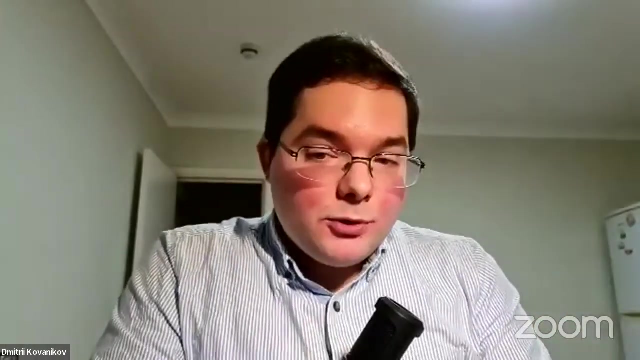 book became down just before my presentation a couple of days ago, which is really unfortunate, just exactly when i wanted to start the course. you can find a height version, so essentially the online version is free. you can buy the book to support the after print book, but the online 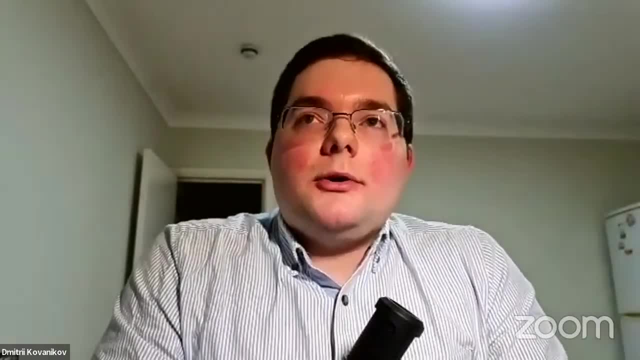 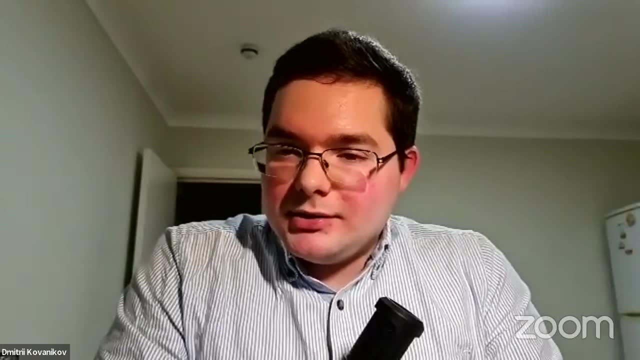 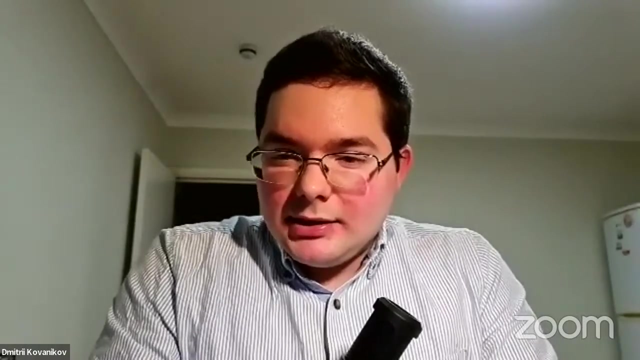 version is free. it's on web archive. uh, you can google it. i will change the slides and i will change the link to web archive so you can actually reach it. but it's uh, you're really unfortunate that this book went down. it has some pretty bad places. i would say some offensive wording. 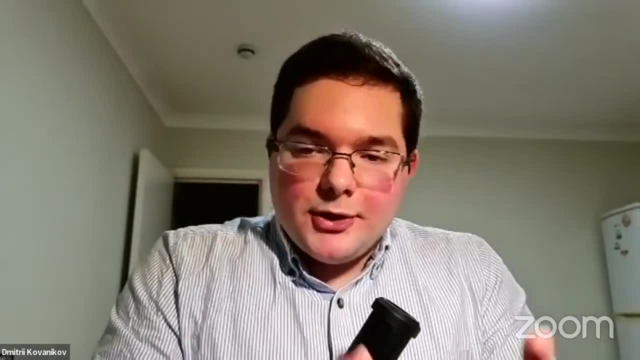 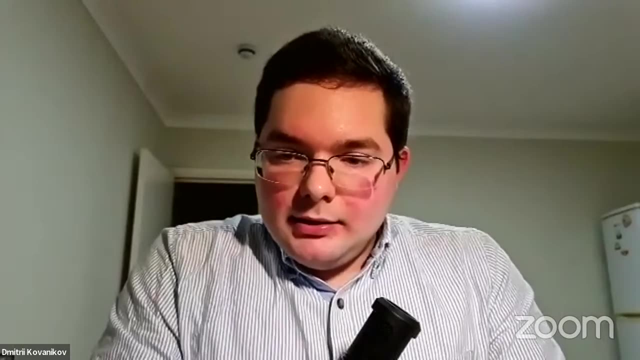 in some cases, but it's a good complementary material to learn haskell besides any course, so i can't say anything about the main thing, but it's a good way to get some useful information. and then some other questions as well, so i can't say anything on how to do it, uh, but it's fine. 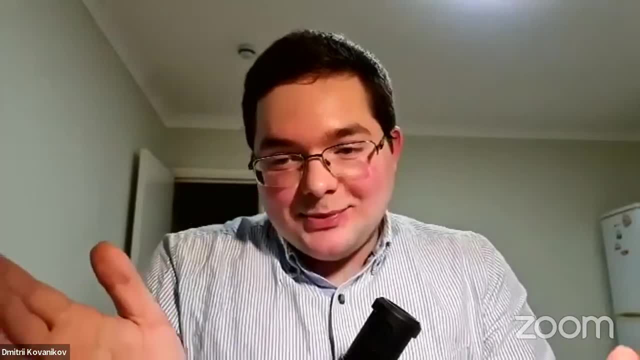 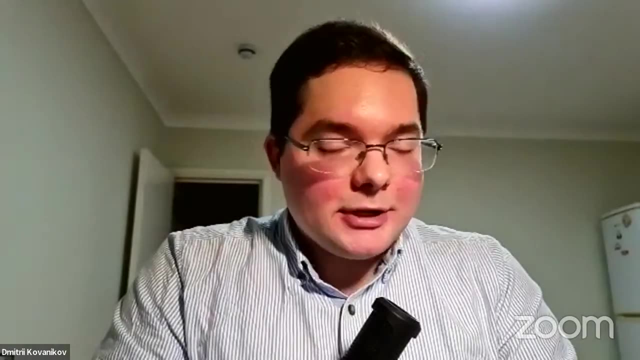 so it's okay to do it, and then you can do it on the subject as well. so if you have any questions, please feel free to ask in the comment section and i will get back to you with a better answer. i will answer all of them as well. when will we get our homework? well, you can start now instead of. 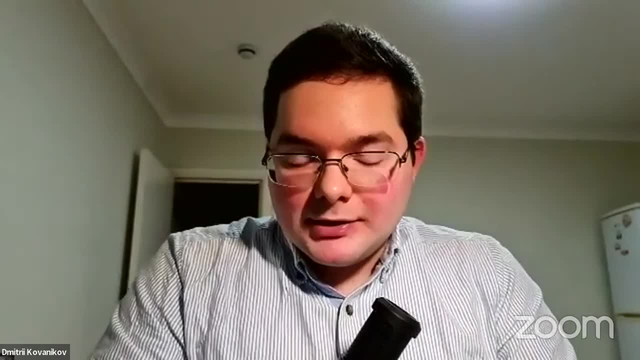 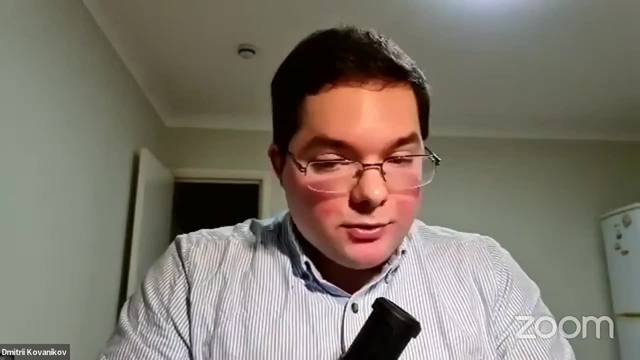 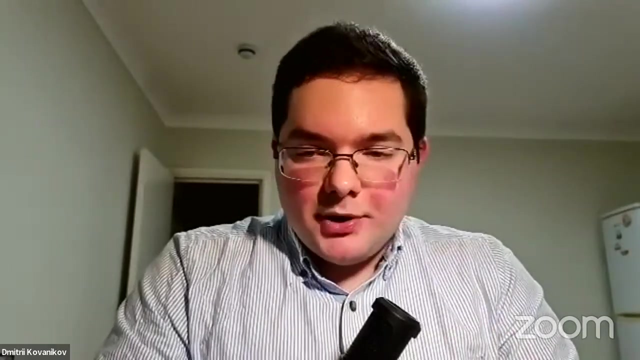 listening to my questions. you can go homework. it's always available public in the finishing exercises for the first lecture, because, um, now should be able to know, to have all the knowledge it's required. so just go to the github repository or fork the repo. start coding openpr. 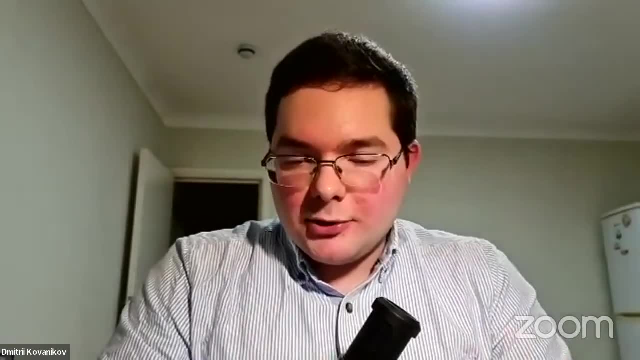 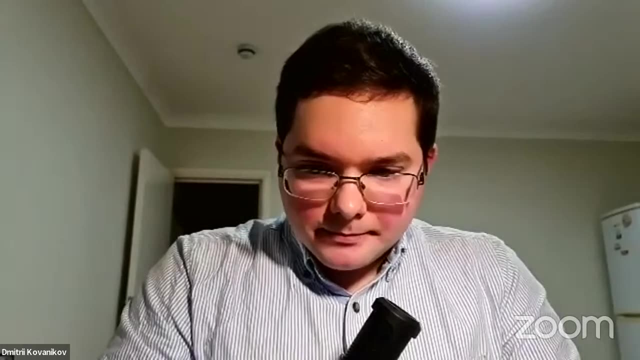 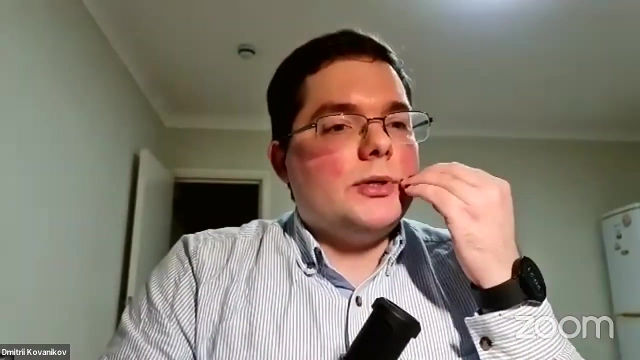 and when you open pr, if there is a pr template, who mentions current mentors? this is me and my friend veronica, and one of us will review your solutions. so, yeah, the deadline is one week. uh, i pinned the message with a lecture time frame, but i guess, uh, i'll write another one with the 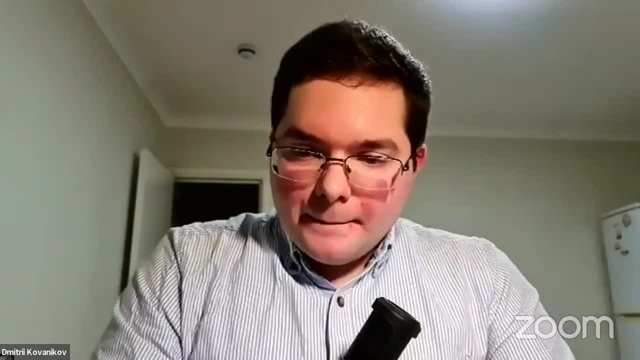 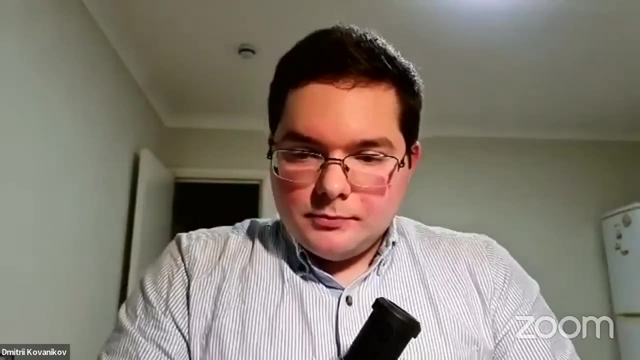 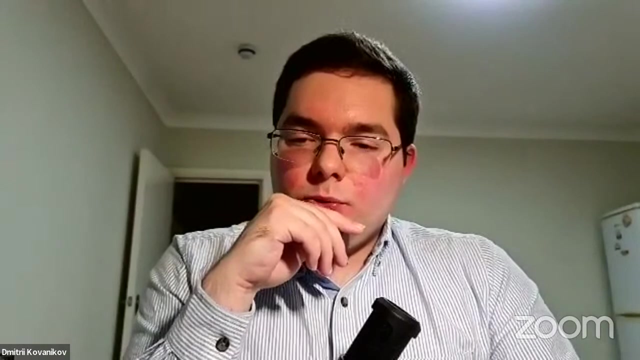 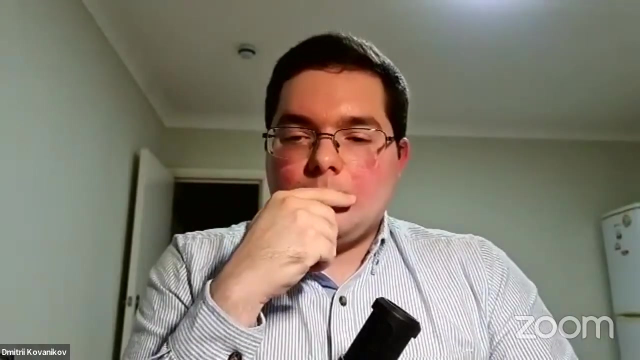 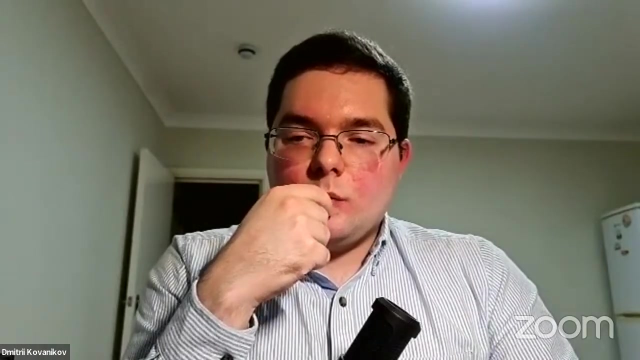 deadlines for um exercises. just maybe same. maybe make sense. and why, when you check the type of number, you get int to int? sorry, i still don't get it well, when you check type of number, you will get this num and the double arrow num. so maybe it's a question for some specific slide. sorry, i guess it's. maybe not that. 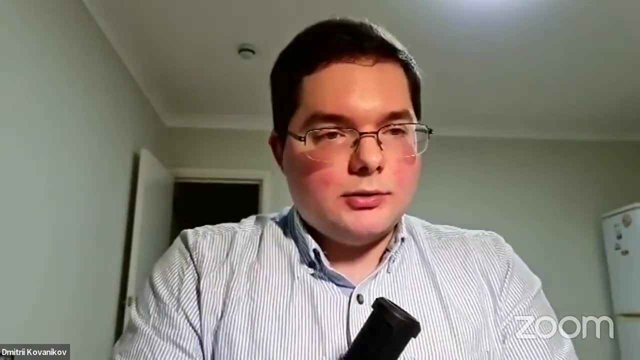 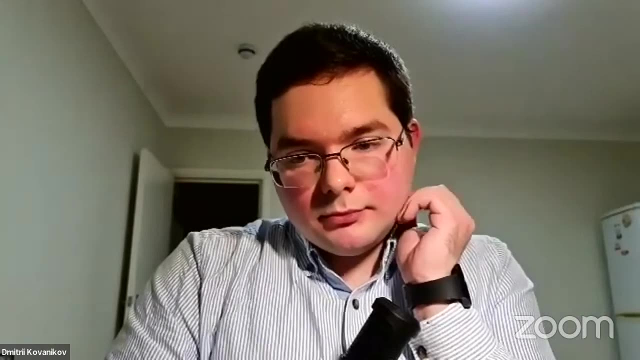 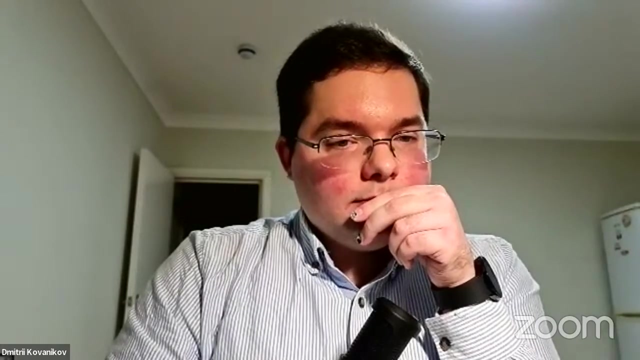 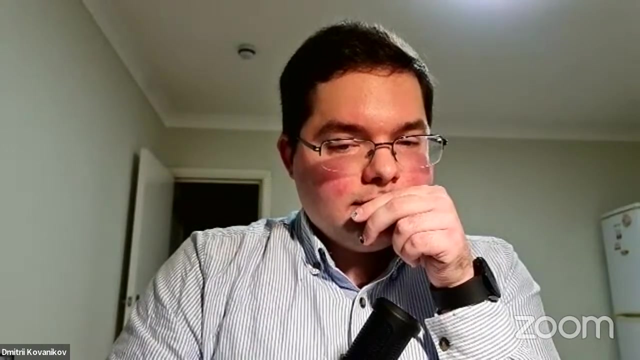 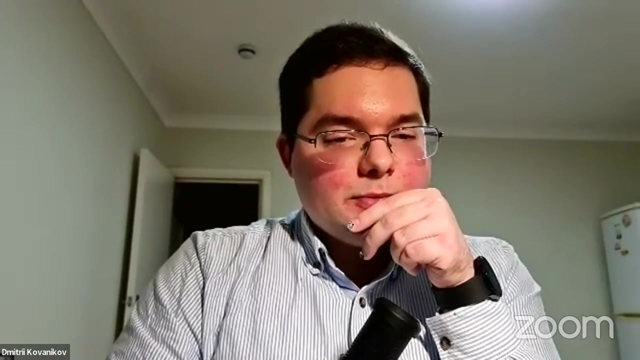 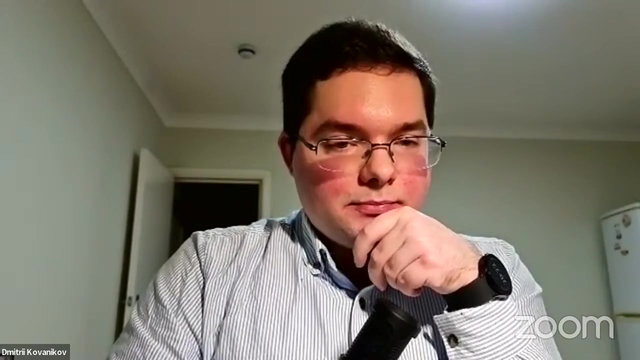 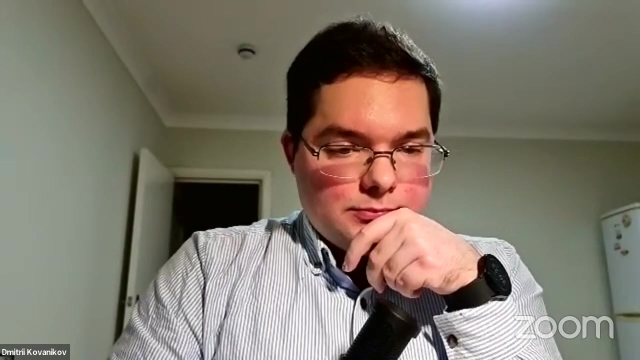 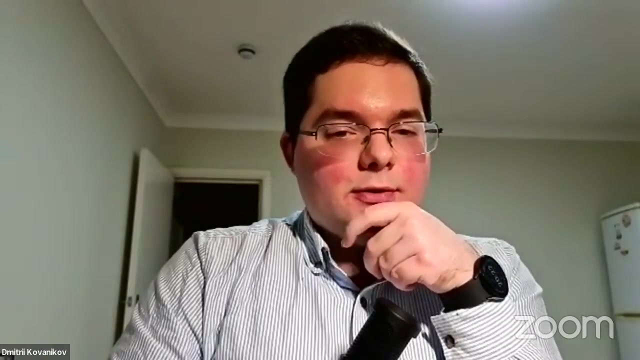 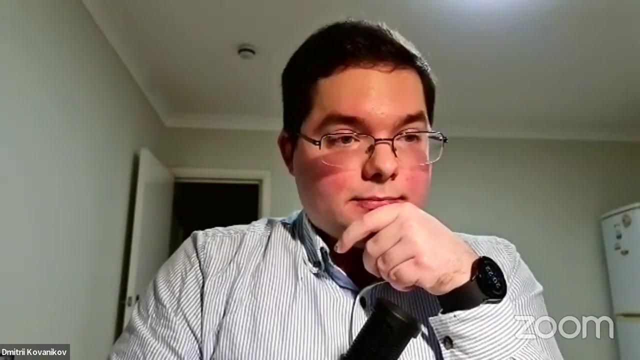 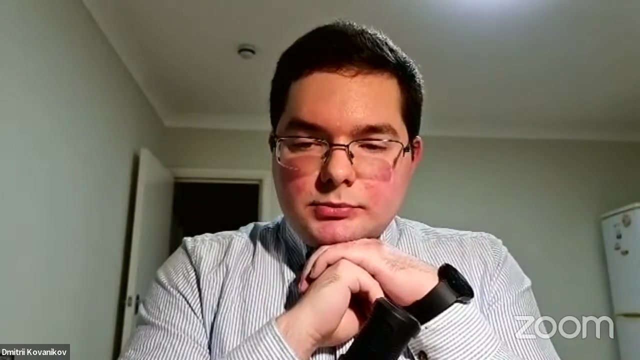 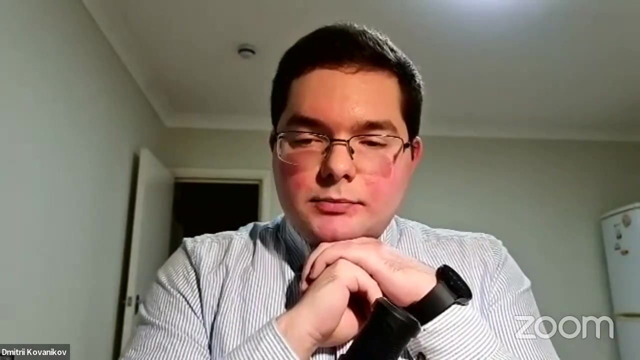 um is to find it, so let me check if there are any questions. that telegram, oh, looks like the memes game is pretty red in the telegram channel and this one was a random question. um, uh, sorry, the doom is what i'm using right now. sorry to hear that. i hope you will feel better. uh, based at the time of 12. okay, yeah, all questions ask you. i get used to write my list, filter x, creating zero but inUSTrl. i have to pass predicate first and list the second way. ah, i see, so this is. 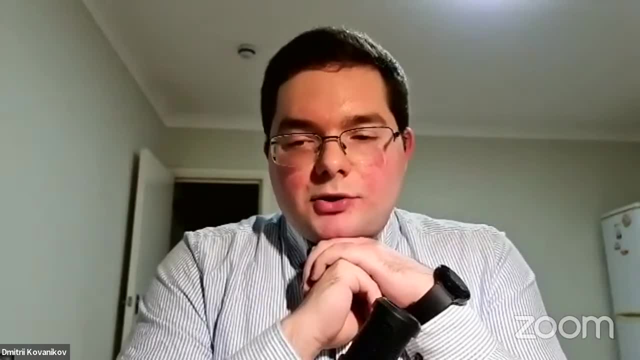 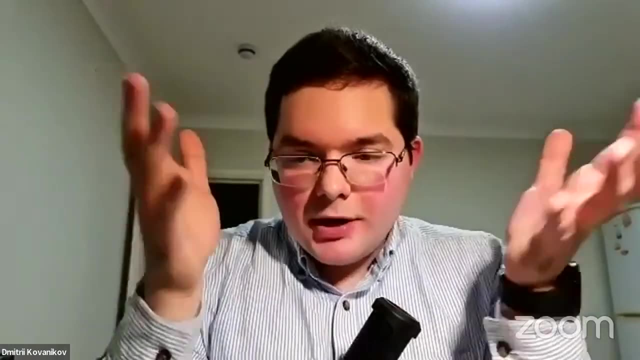 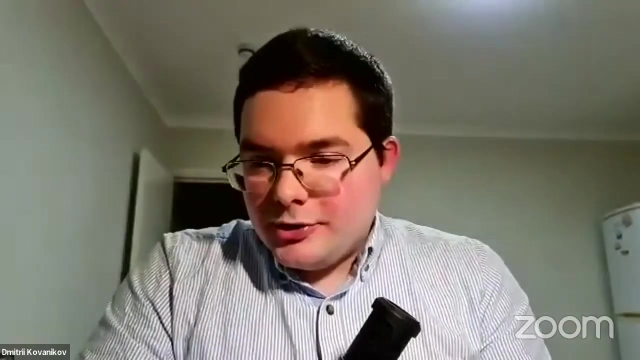 just because we defined our function like this. so a satisfies function, we wrote in the step signature. so it takes, uh the fun. the function is the first argument and the number is the second. if you write your own function, you can just swap the type signature elements in the signature and accordingly. 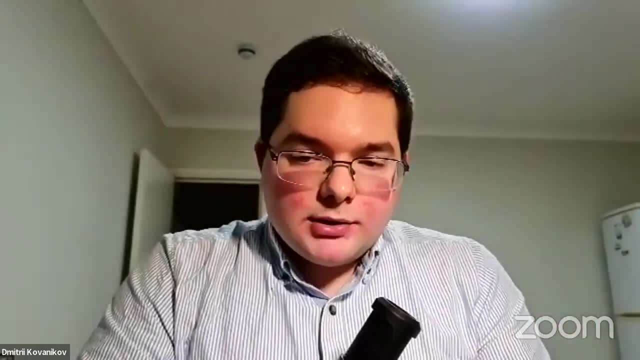 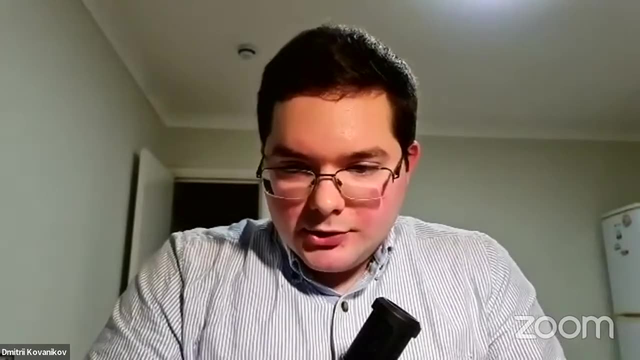 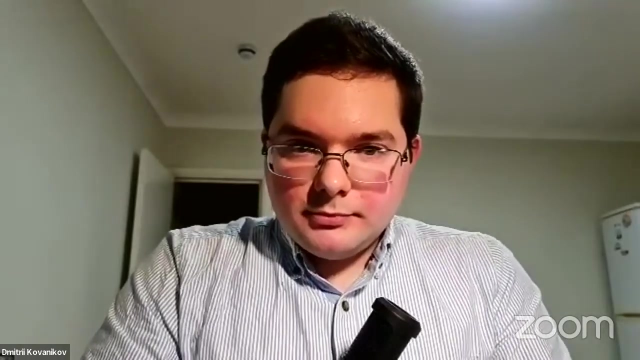 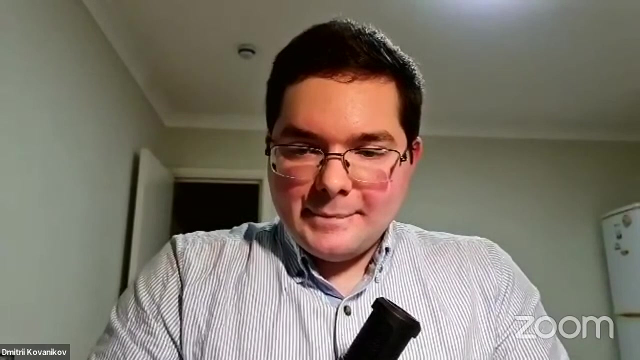 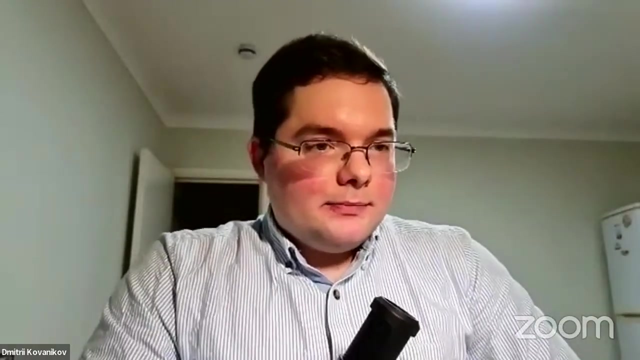 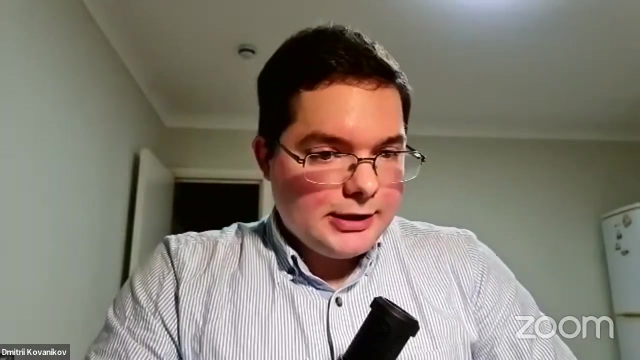 swap the name- variable names, and you will be able to pass the element first and then the lambda last. so there is no special reason, it's just how you want to write: cool, cool, cool. so yeah, as i said, the recording of this lecture will be available later. 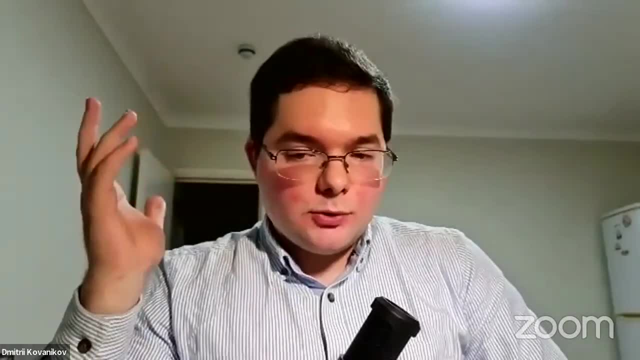 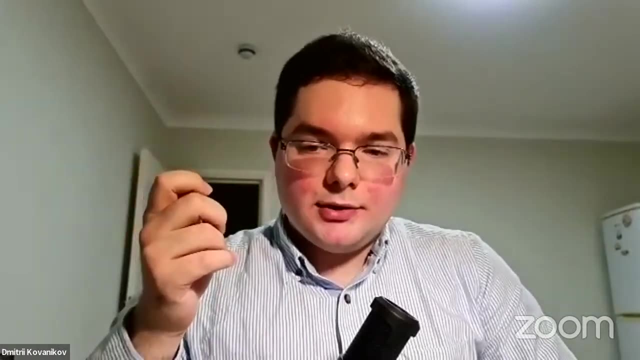 uh, you can start doing exercises, for the first lecture line is one week, so the line is mostly for you, to keep you in good shape, so you will be prepared to the next lecture. as i mentioned that, it's important to practice because you can just watch slides, lecture and understand.